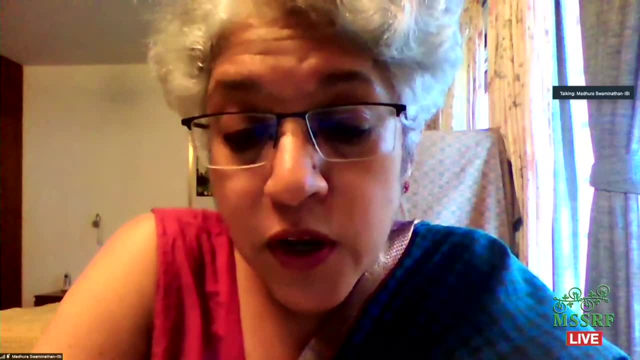 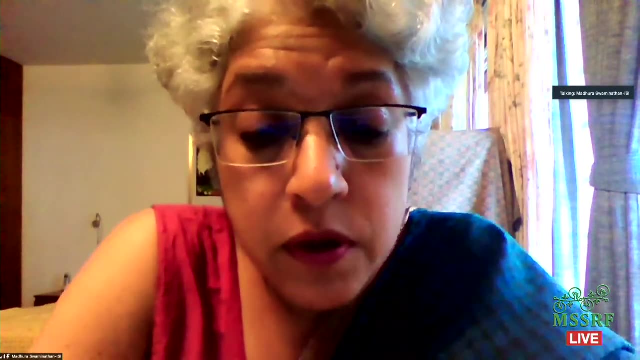 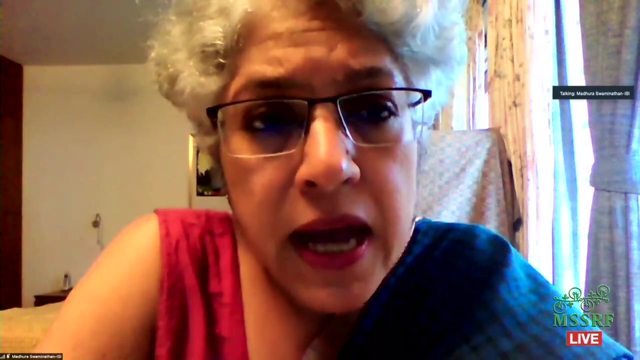 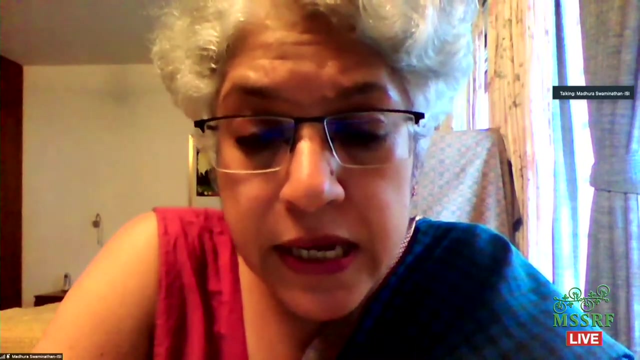 what was started as rationing network in the 1940s during the British period when there was rationing in on account of World War II in Britain and some form of rationing was started here And it has persisted and it has become an important in-kind, in-kind support for households particularly. 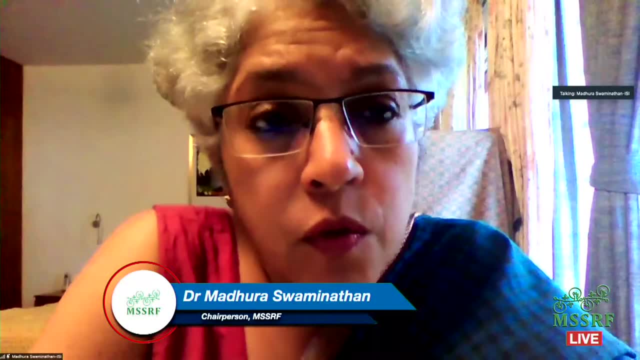 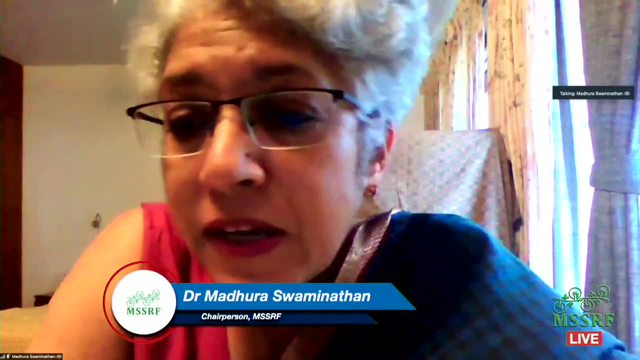 the poorest households in the country. So I would like to start with that and then I would like to move on to the question of the economic liberalization and the economic liberalization of the country Now for the last 20 years, particularly from the 1990s, when economic 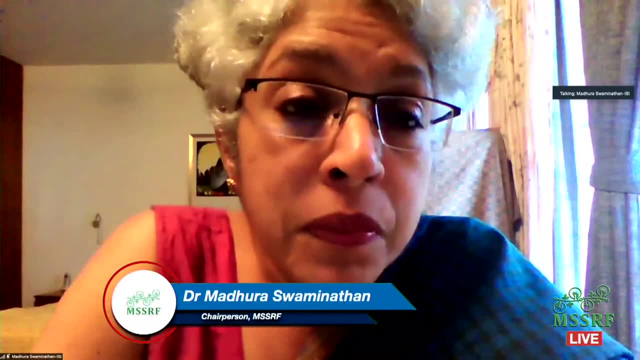 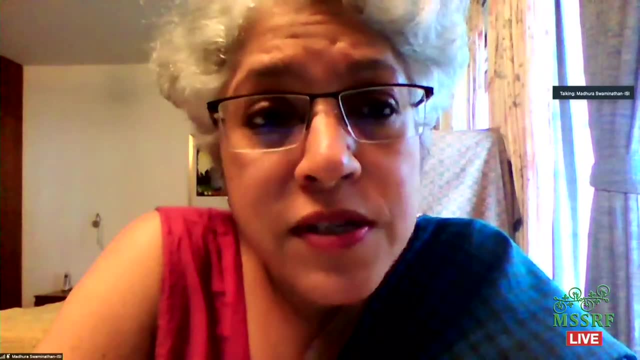 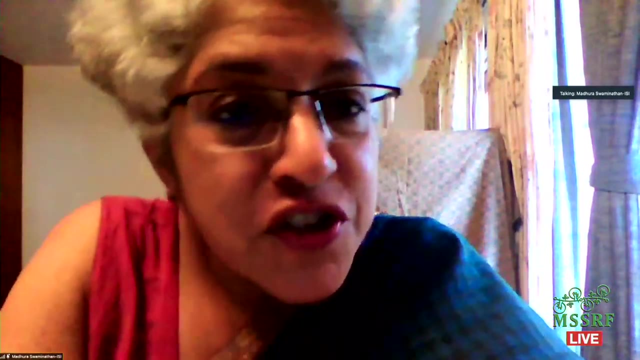 liberalization began world over. one of the big debates in India and I think, in many parts of the world, led by the World Bank and others, was: let us move away from kind to cash. you know why. why go for kind transfers? you know when cash transfers can be. 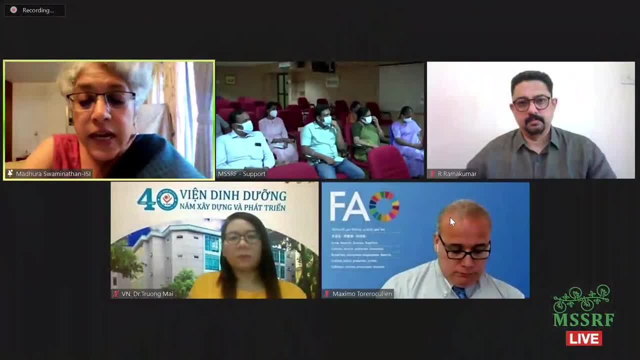 allow the household to make their own choices and so on, And many people in India, including myself. we fought quite hard to ensure that some forms of in-kind transfers remain because, for many reasons, these are inflation-proof And often, as we have discussed even in the previous sessions. 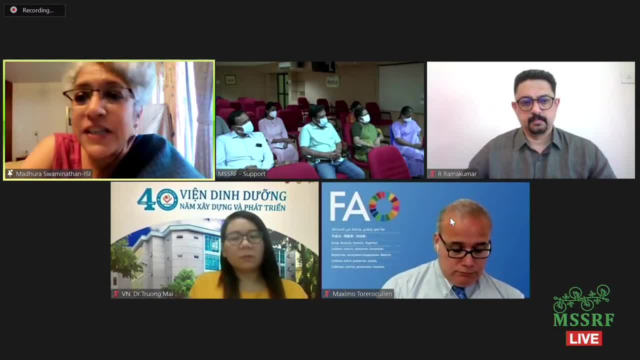 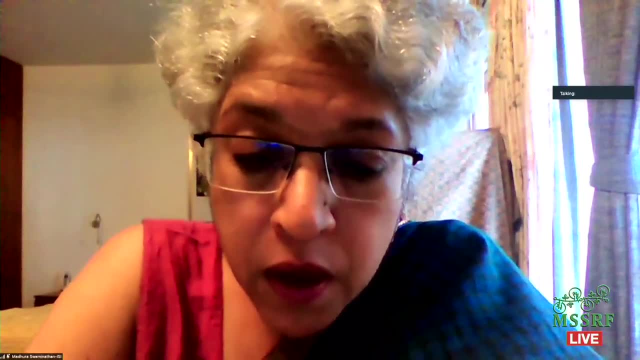 it's a question of accessibility and affordability. It's not just a question of having adequate income to spend on food and other items. And looking back last year in March 2020, when we went down into lockdown in India as elsewhere in the world, 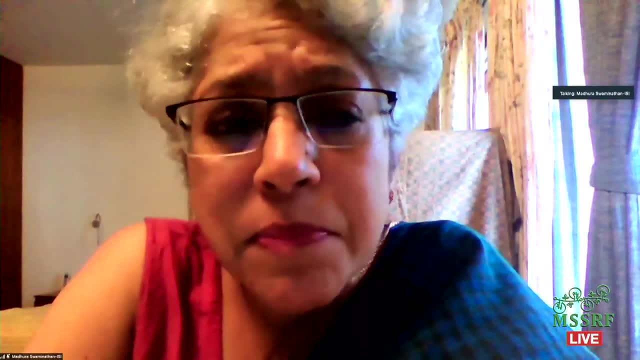 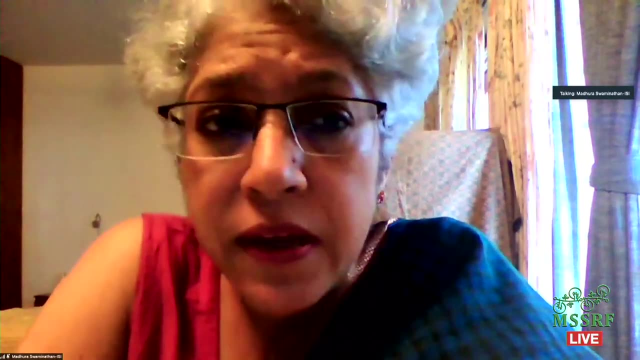 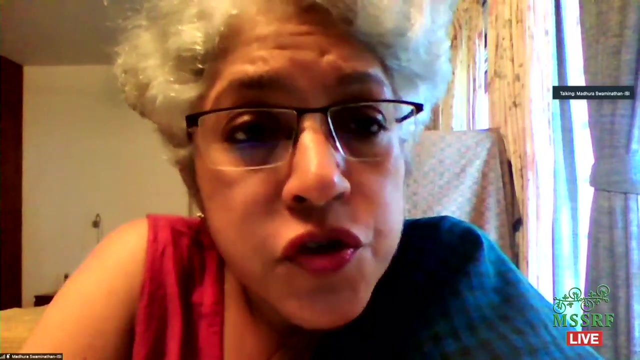 we were lucky that we had this system in place and that it had not been dismantled by neoliberal economic policy, because it could be. it varied, of course, a lot across states, but it could be immediately put put into place to distribute basic foods to households. 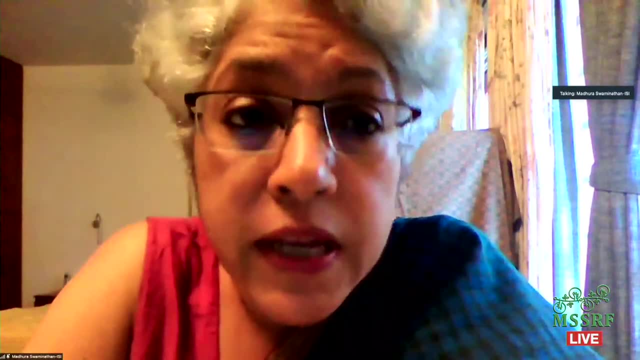 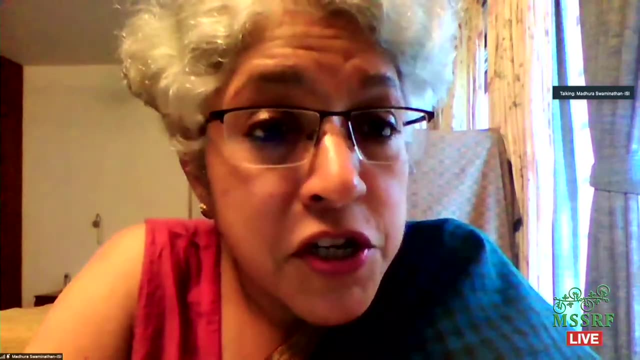 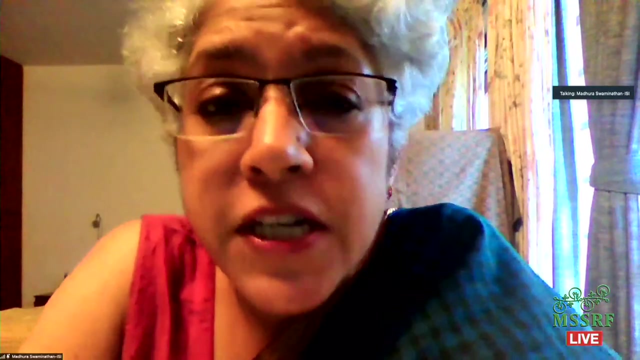 who were sitting at home with no form of employment or income, And some states in India took the lead. some did it better than others, and I want to mention here Kerala, which I think set an example in terms of the variety of commodities that were distributed. 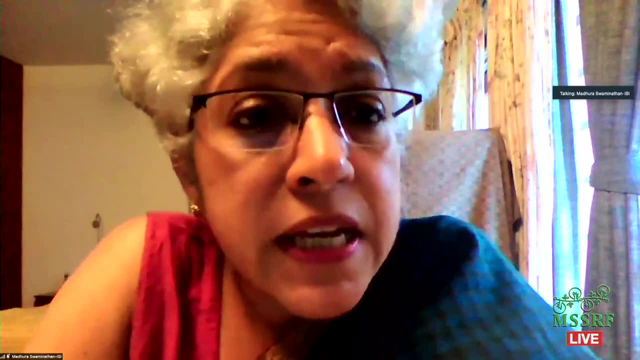 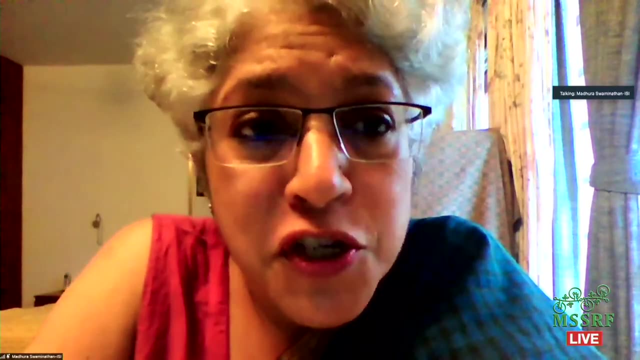 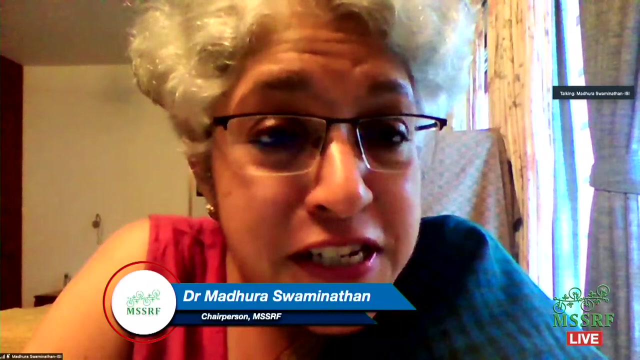 It wasn't just rice and wheat. There were 17 commodity kit that was distributed to households. So I think that's an example of using the crisis to actually take nutritional or dietary diversity to the doorstep. Of course, these costs, these are expensive if you have to provide 17 commodities. 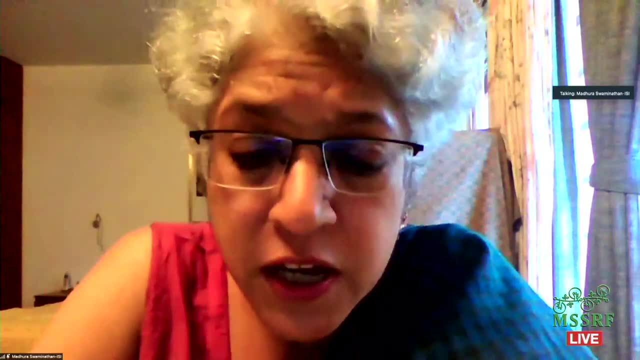 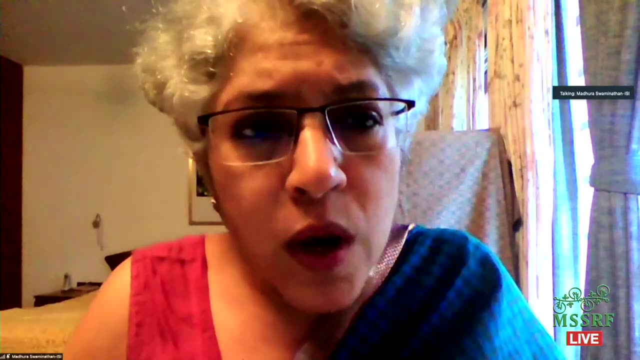 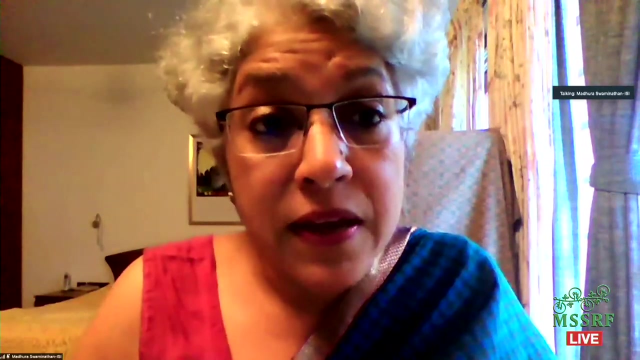 and we need to think about resource mobilization and many other issues. So I hope I'm just giving this example to show that you know when we talk about building back better, when we talk about using this crisis to you know, maybe bring attention of the world. 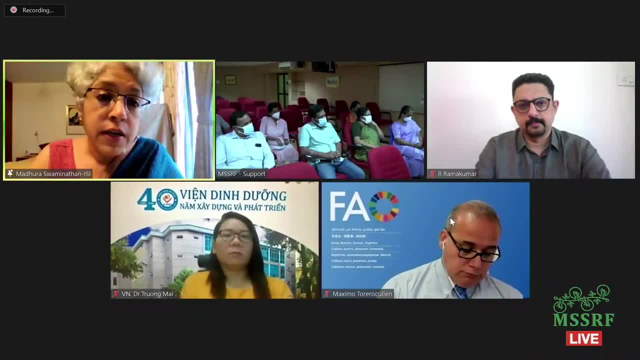 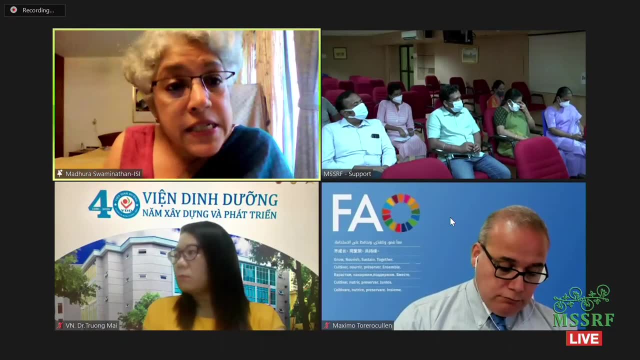 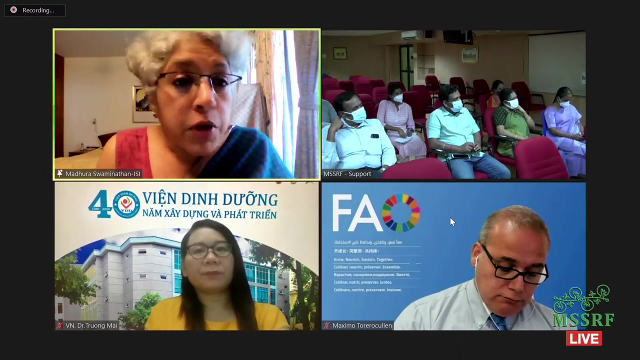 I think people here have been paying attention to this problem for long, but maybe many policymakers have not been paying attention to the severity of food and nutrition insecurity in India, as in many other parts of the world. Let us examine the features of the change and the main factors, and also come up with doable policies. 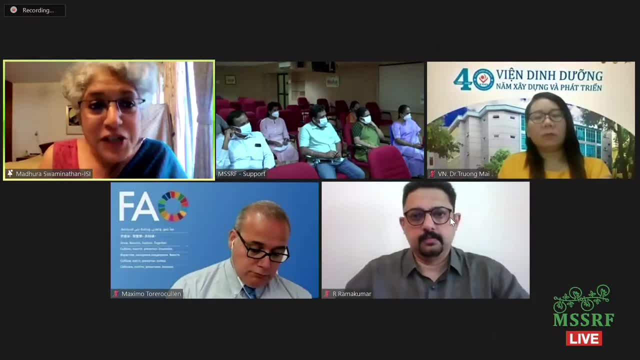 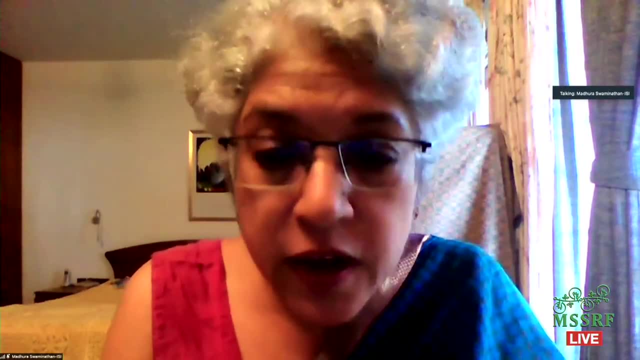 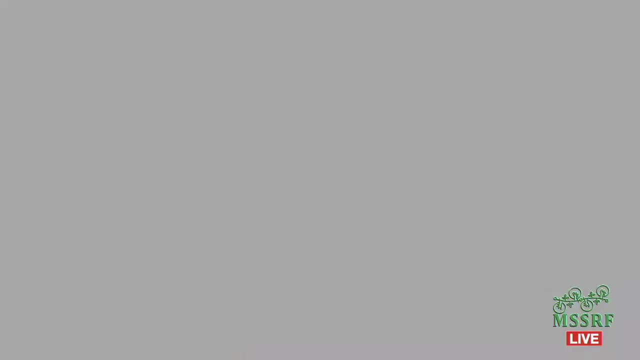 So I will not go on too much, because I think we have a very rich experience in the speakers we are going to hear. So let me start with Dr Maximo Torero-Cullen, who is the Chief Economist of the Food and Agricultural Organization. 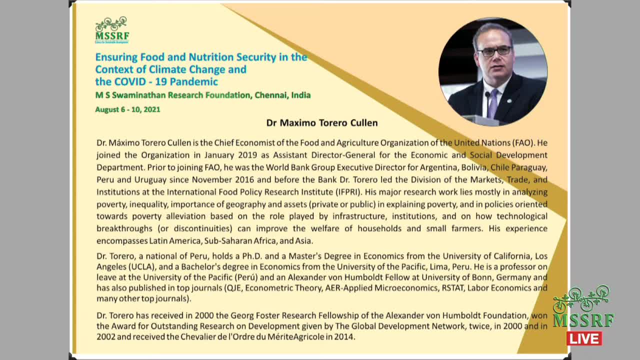 FAO of the United Nations, And earlier he joined as Assistant Director General of the Food and Agriculture Organization. So let me start with Dr Maximo Torero-Cullen, who is the Chief Economist of the Food and Agriculture Organization- FAO of the United Nations. 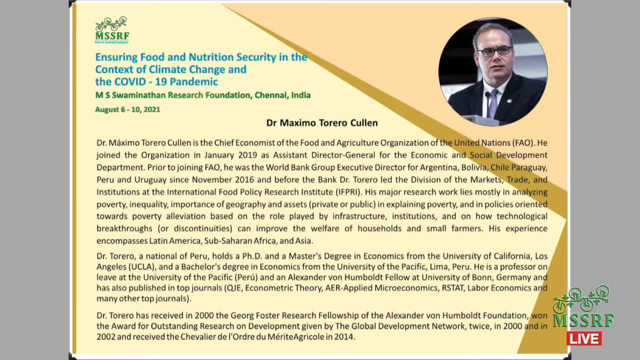 So let me start with Dr Maximo Torero-Cullen, who is the Chief Economist of the Food and Agriculture Organization FAO of the United Nations. He is the Director General of the Economic and Social Department. He has a long experience working at the World Bank, working at IFPRI. 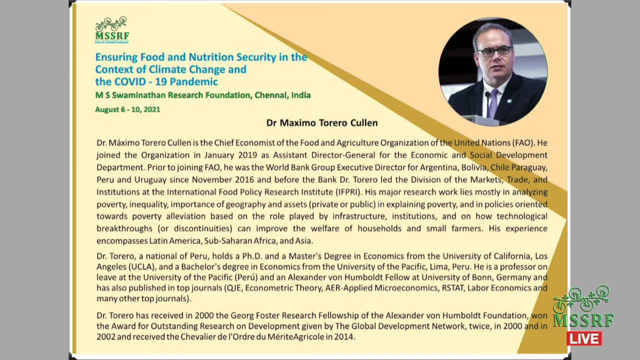 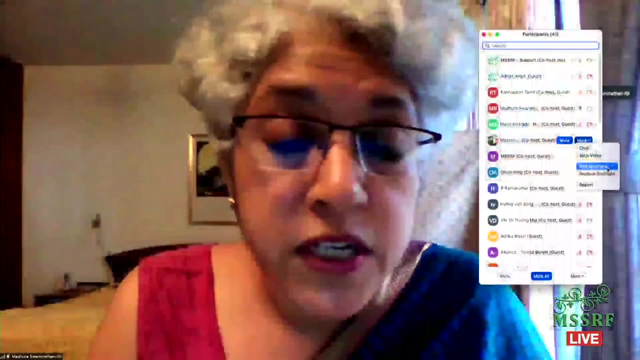 and working in Latin America, Sub-Saharan Africa and Asia. I would like to now invite Dr Torero to make his remarks on the issue of dealing with policies for food and nutrition security in the context of COVID. Five minutes of silence And can I request you, as was done by our coordinator, to speak for about 15 minutes. 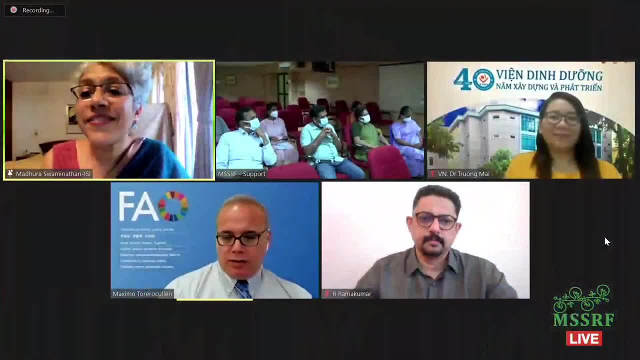 Over to you, Dr Torero, Thank you. Thank you very much, Chair, and it's a pleasure for me to be here. Let me share my screen with my presentation. So, essentially, I think this meeting comes at a pretty important time because this was mentioned not only in the Salım tentang Ty宇tyreł. 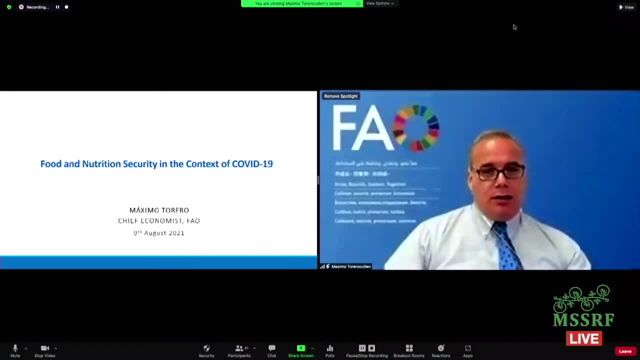 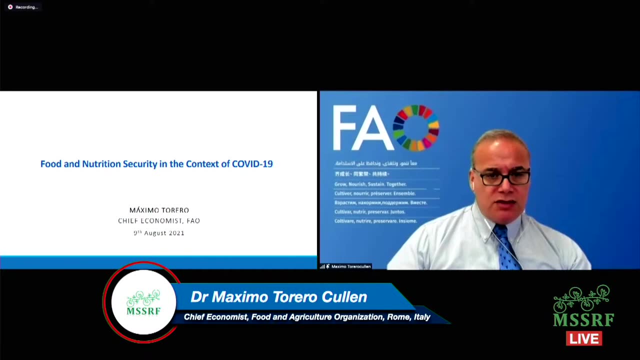 but also in an effort towards redesigning the European Union, because we are speaking about a lot of trade. The trade is 얼마나 important? is it necessary? I don't know if you understand what I'm trying to get at, or it's not just pitch? 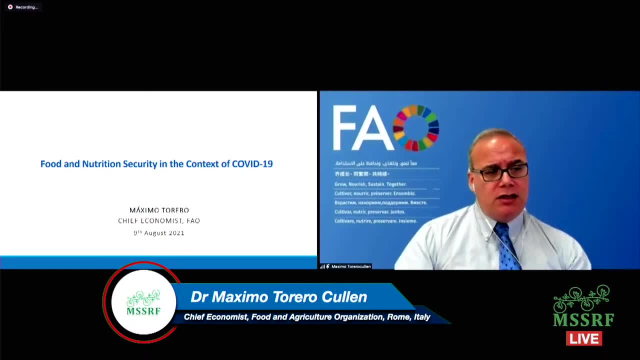 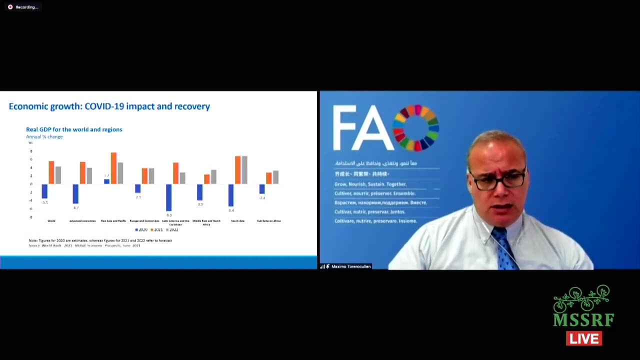 is important for India, is important for the world, is part of the food system summit and the pre summit just finished a couple of weeks ago. so I think what we are discussing today is of crucial, crucial importance. but my job is is more to to bring up the global level and trying to see what 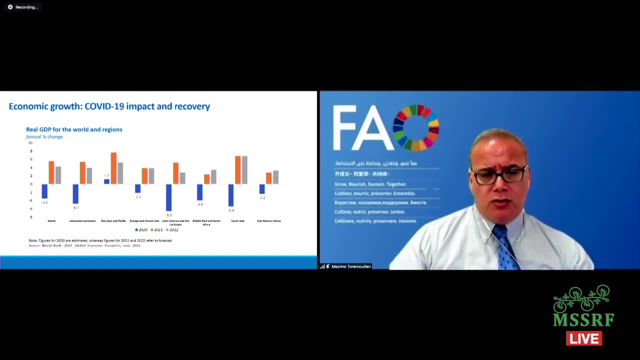 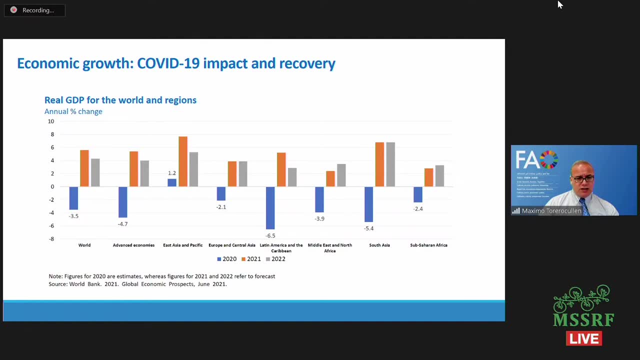 we can learn from from the world, global level. so what clearly we know is that the world economy has contracted by 3.5 percent last year, with regions like Latin America and South Asia taking in a particularly severe blow because of this crisis, and a rebound is expected in 2021, although 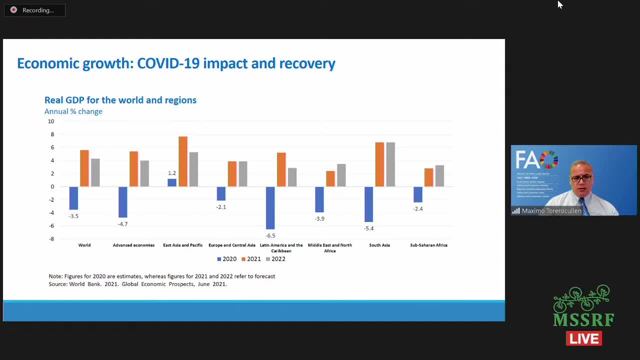 of course, this has an assumption that there won't be another round of coordinating, which sadly seems that will happen because of what we are observing lately. and the other issue which is important is the global disparities that we are observing which are related to the, to the access to vaccines, and how that can also exacerbate the effectiveness of any potential recovery in 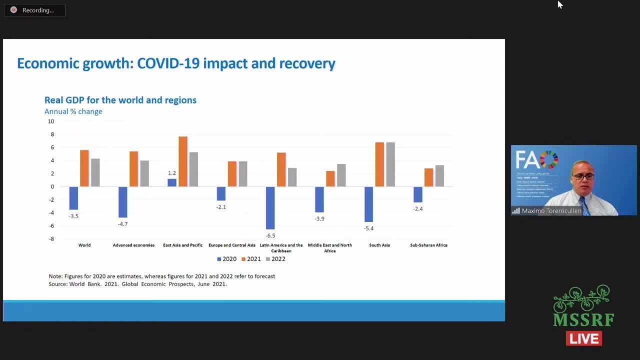 the future. so by 2022, global GDP will remain about two percent below pre-pandemic levels. poorer countries are projected, on average, to see larger output losses than richer countries, and many developing nations, especially Sub-Saharan Africa and America, are not expected to return to pre-pandemic levels until 2023.. so the situation is not a situation of one year, is a situation that 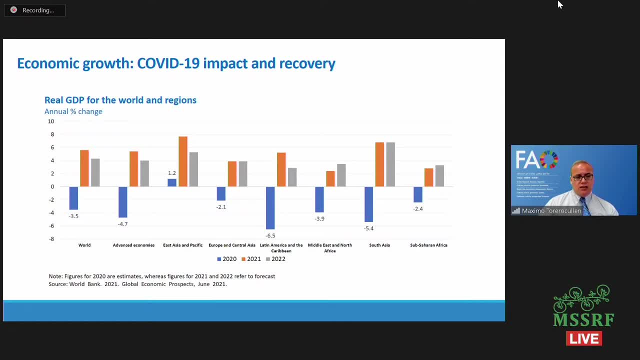 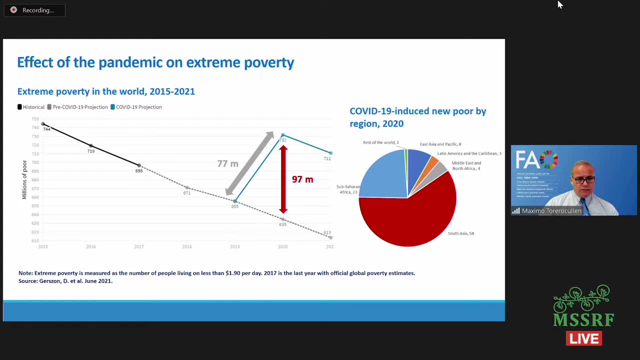 will affect several years, and that's what we need to to take into into consideration now. GDP contraction and the lockdown has increased poverty around the world. according to the World Bank, there was an spike of 97 million more people in poverty in 2020, a historically unprecedented. 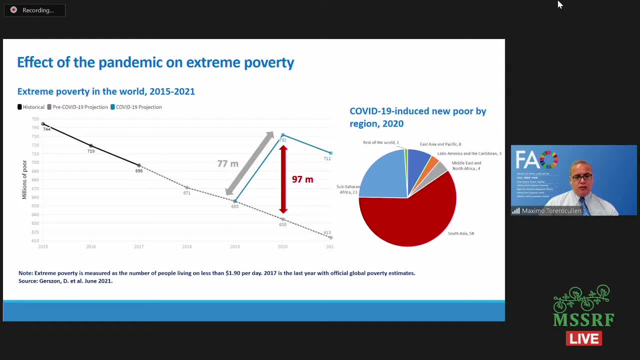 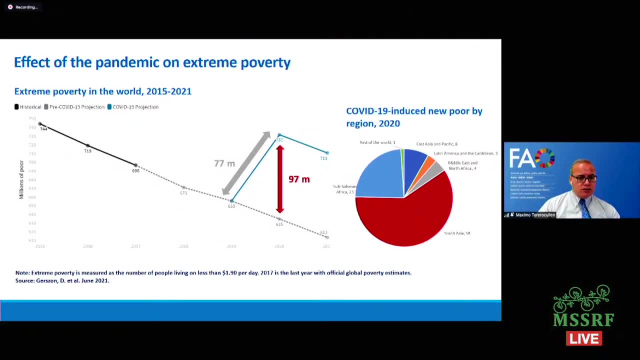 increase in global poverty, with about 60 percent of the new poor in South Asia and another quarter in Sub-Saharan Africa, and the prospects remain dire for many of the world's extreme poor, and the majority of whom live in in rural areas. so, again, it's another element that we 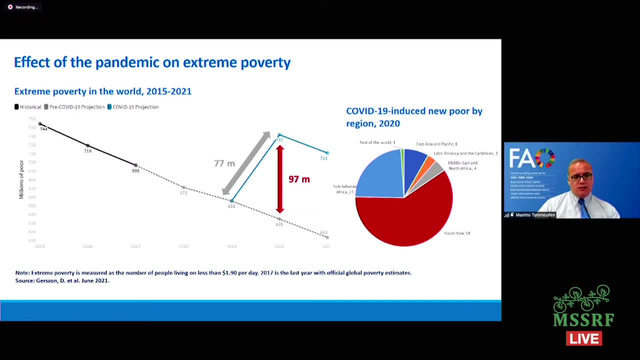 need to take into consideration and in regions where we have a middle class, that middle class has been trained and move into levels of poverty. so, in short, we are far from turning the corner on poverty, and the recovery that is taking place will not be sufficient to close the gap that. 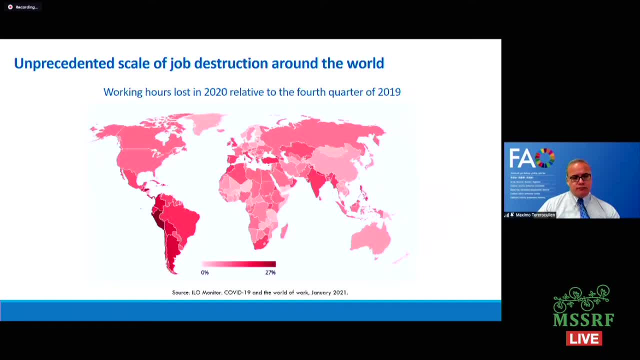 the pandemic is estimated to have caused in in 2020.. ILO estimates also that 8.8 percent of the global working hours were lost in 2020 relative to the fourth quarter of 2019.. and is a decline equivalent 255 million full-time jobs, about four times greater than experience. 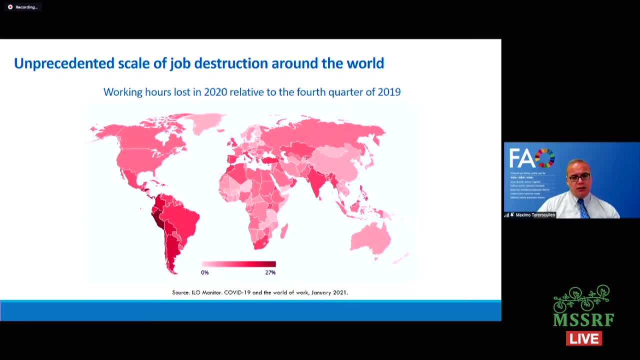 during the global financial crisis in 2009, and while the scope of the disruption was global, there was a substantial variation across countries, depending on the structure of their economies and the restringency of containment measures, and this brings again the importance of inequality. if you look at this map, for example, my country, Peru, is dark right, which means that it has been 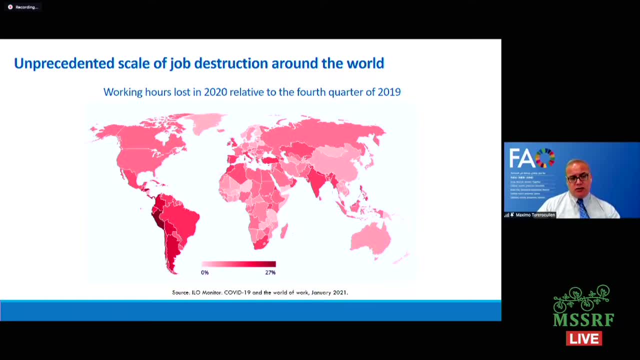 substantially choked, and that was because of the duration of the lockdowns, but also because of the levels of informality, and many countries in South Asia face similar situation, and the hardest hit sectors are those where young workers, women, the self-employed and those in informal economy. 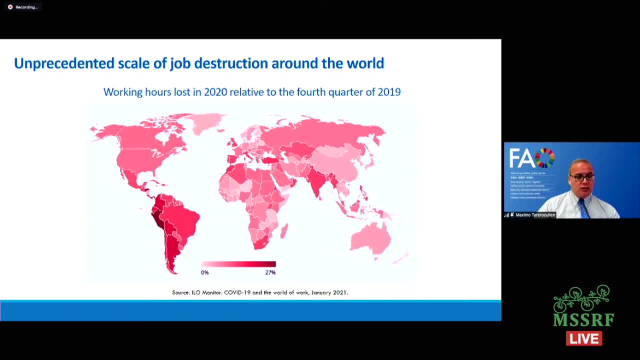 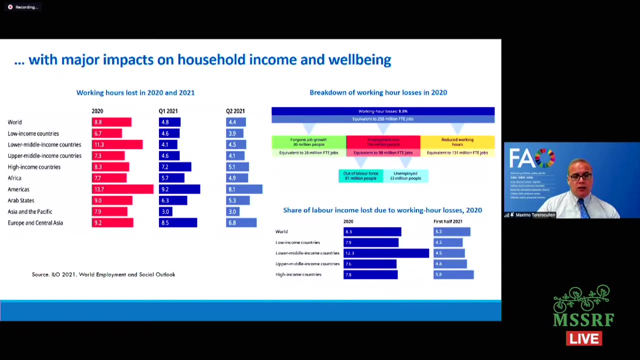 including rural, council and seasonal laborers, are over overrepresented. This has widened the gap relative to high skilled service sectors, heightened vulnerability and inequality and raises the specter of uneven recovery into the future. If we go into details, the global decline in working hours was driven by increasing inactivity and in unemployment, as well as a 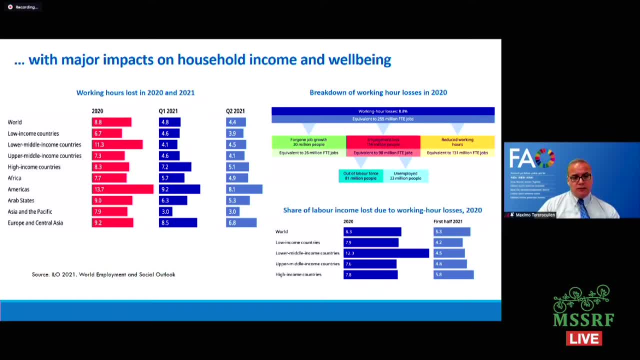 massive reduction in working hours for those who remain employed. Half of the laws took place during the second quarter of 2020. as a strict containment measures kicked in lower means. The effects were mostly felt, with a drop in working hours of 29% during the 2020 quarter 2. 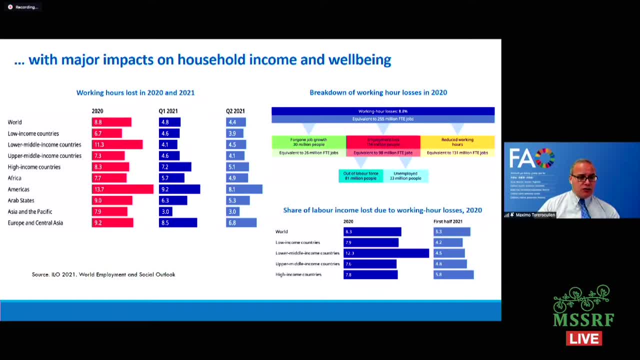 and a total loss of over 11% for the whole year. This has naturally led to a major contraction of the global labor income and, if you must understand, this is a correlate with food access. If you don't have income, you won't be able to buy food, so no matter food could be available, this will affect. 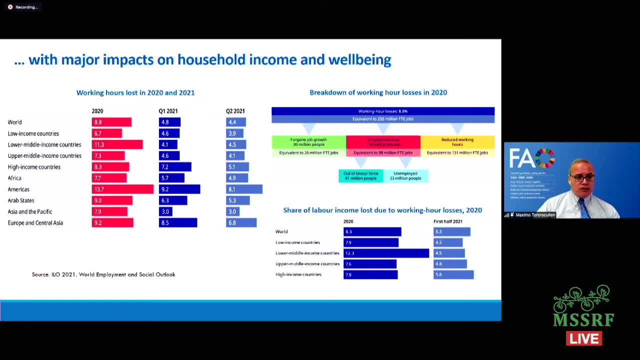 substantially the income And the amount of food that is available is not enough. The amount of food that is available is not enough And the amount of food that is available is not enough And the amount of food that is available is not enough. The amount of losses are. 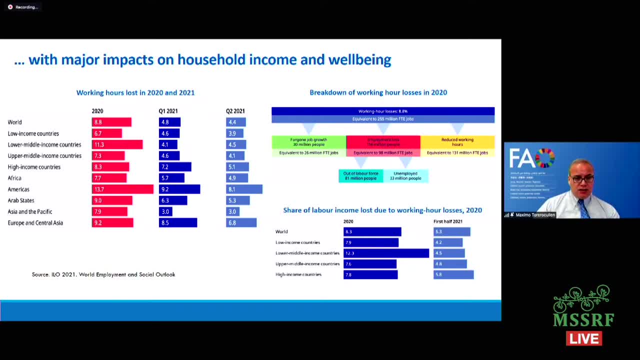 around 3.7 trillion, or 4.4 for the global GDP. And despite the roll out of vaccination and the gradual shift away from economy wide closures, the prospects for the global economy remained by uncertainty, significantly uncertain and restrictions are wide spread. And again this 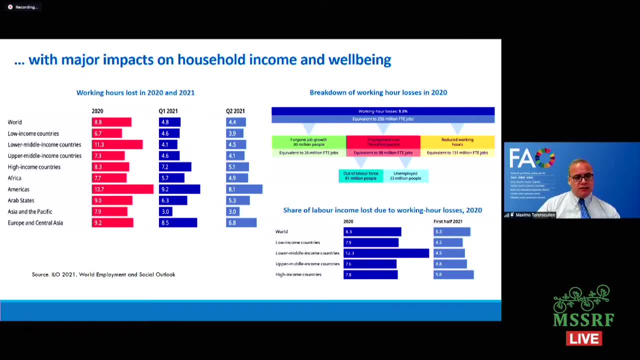 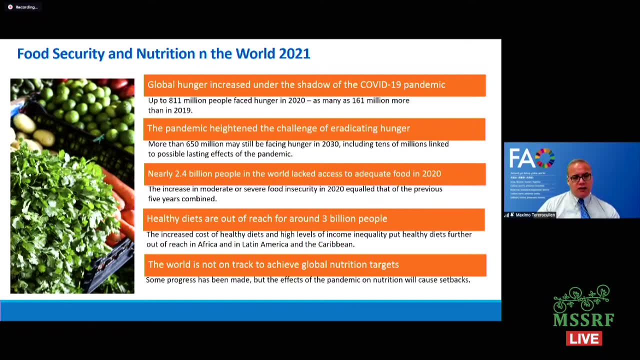 could have a longer period of time effects in the world. Now what is the situation of food security and nutrition? And these are the results we obtain in this rite of due discussion. If we go to a Sophie that was published a couple of weeks away, so essentially up to 811 million people. 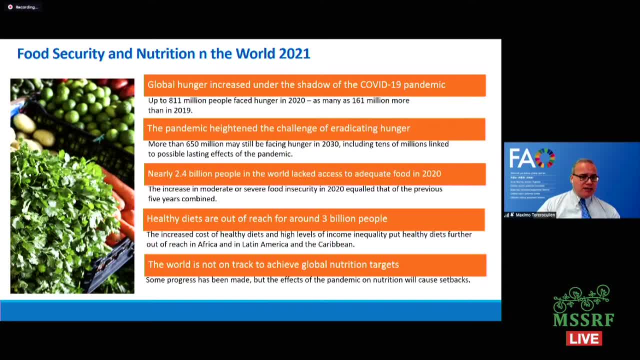 were facing hunger in 2020, and this is up as many as 161 million people in a single year. more so, between 2019 to 2020, there was an increase in 160 million people more, which is one of the biggest spikes that we have seen in the last decade, and more than 650 million people may. 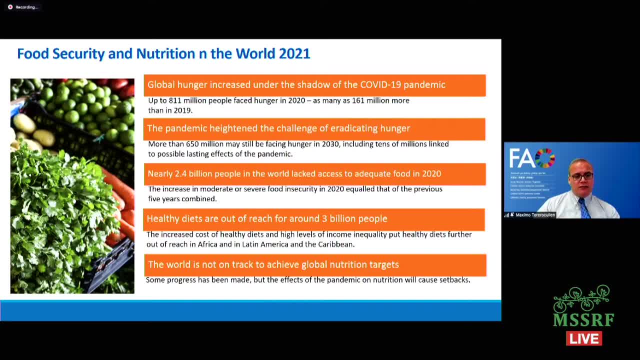 still be facing hunger in 2030, so we will be far from achieving se2 and beyond hunger. nearly one in three people in the world were affected by moderate or severe food insecurity in 2020, and the increase from 2019 to 2020 was equal to that of the previous five years combined. 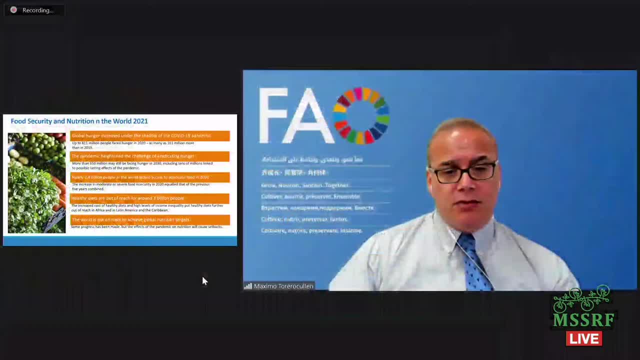 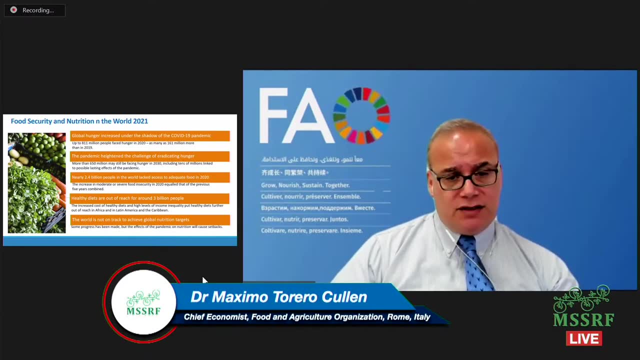 so healthy diets are also out of reach for three billion people due to the high cost of healthy diets and high levels of income inequality in many countries, which has been even more exacerbated because of covet 19.. with respect to indicators of nutrition, some progress has been made. 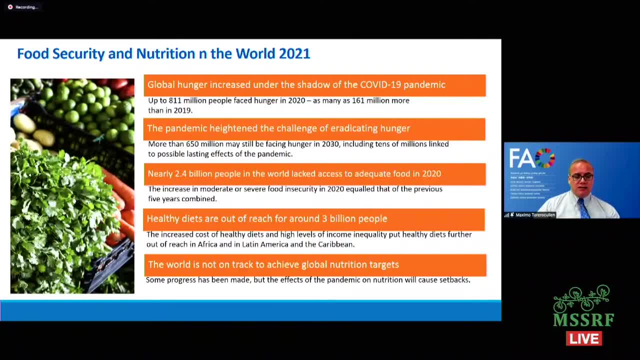 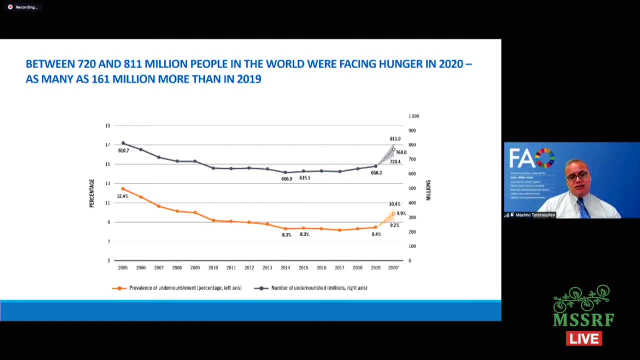 but the world is still not on track to achieve global targets. and the kobe 19 pandemic. now here i'm just showing the historical trend that you see at the last years, the significant spike that we have in the nourishment indicator that we measure at fao and we track every year. 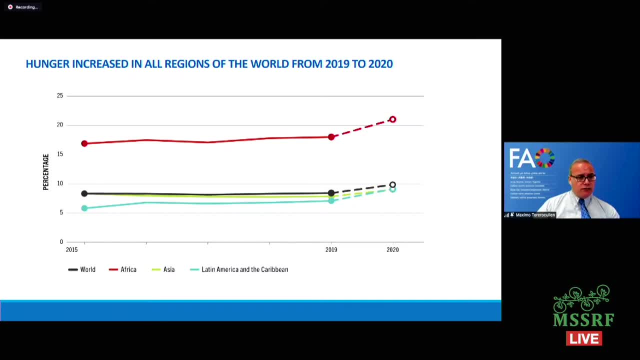 now. hunger increase in all regions of the world. from 2019 to 2020. there was no exception. the sharpest increase was in africa, followed by latin america and the caribbean. more importantly, all sub-regions in africa and in latin america and the caribbean, and most of saharan. 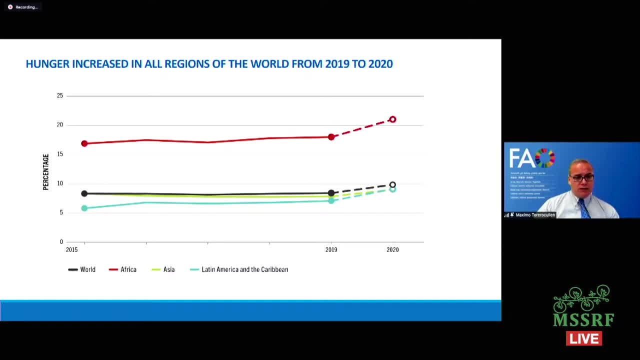 sub-regions of asia also show an increase in the pandemic year compared to 2019. about 46 million more people in africa go to undernourishment, 57 million more in asia, and about 14 million more latin america and the caribbean were affected by hunger in 2020.. so 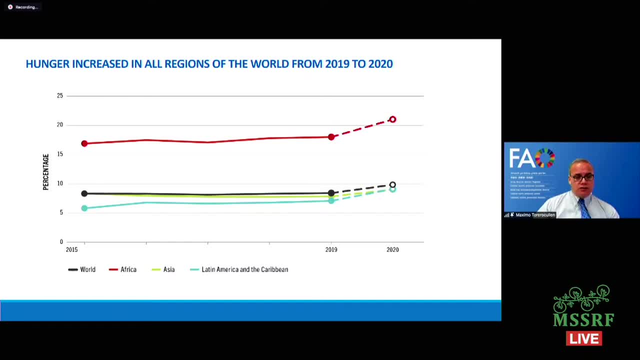 overall, more than half of the global population is affected by hunger in 2020.. so, overall, more than half half of the world's and the nourishment are found in asia- 418 million people- and more than one-third in africa- 282 million people. now this year, we also did an enormous effort to project. 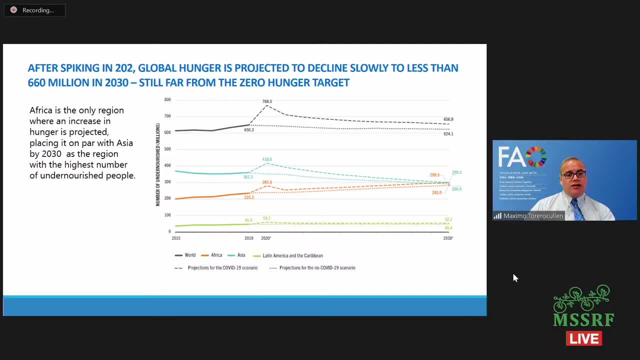 what will happen because of this spike over the future, over 2030? and these projections consider the potential impact of the kobe 19 pandemic and suggest that, following a peak of more than 760 million people in 2020, global hunger will decline slowly and 660 million in 2030. and this is the result of a modeling exercise where we bring all the 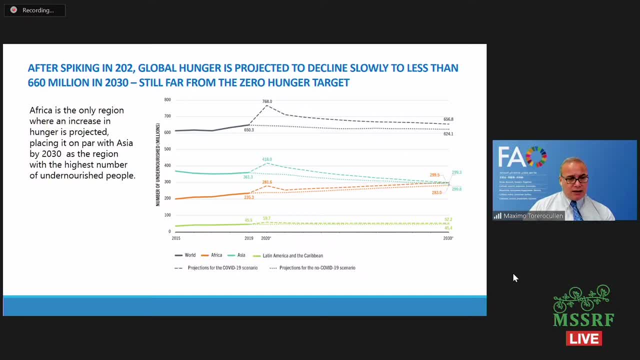 potential dimensions that could be behind a hunger. so this represents tens of millions more people than projected for 2030 had the pandemic not occurred. so the pandemic had a significant impact in this increase in undernourishment and that's what we show in this graph. so a substantial 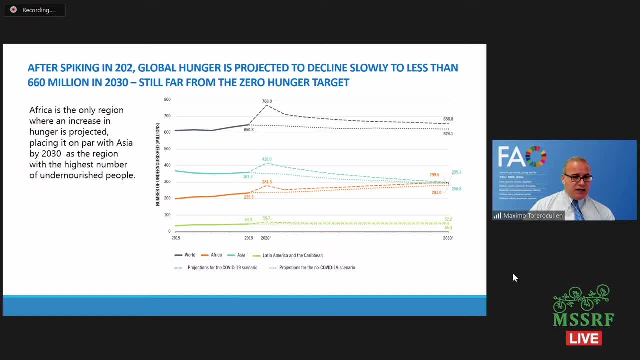 reduction in hunger is projected for asia by 2030, but a significant increase is forecasted for africa, and this will place africa on par with asia by 2030 as a region with the highest number of undernourished people. and hunger will not be eradicated by 2030 unless both actions are taken. 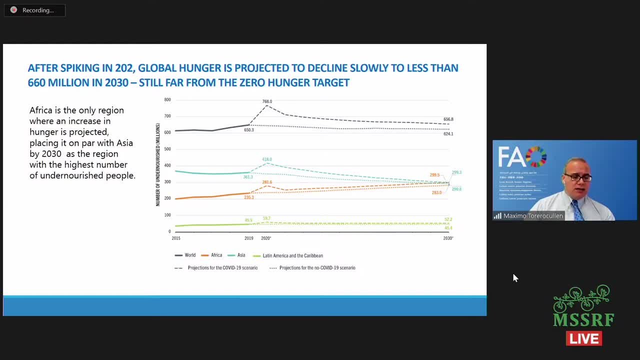 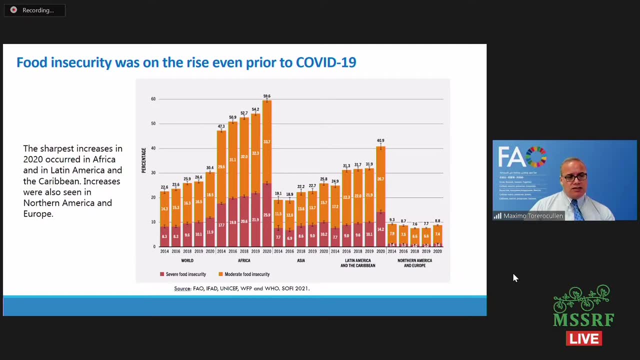 to accelerate the progress, especially actions to address inequality and access to food. now nearly one-third in three people- and this is the other indicator that we use, which is the fees- the food insecurity experience scale, and here we show that one in three people in the world, so two. 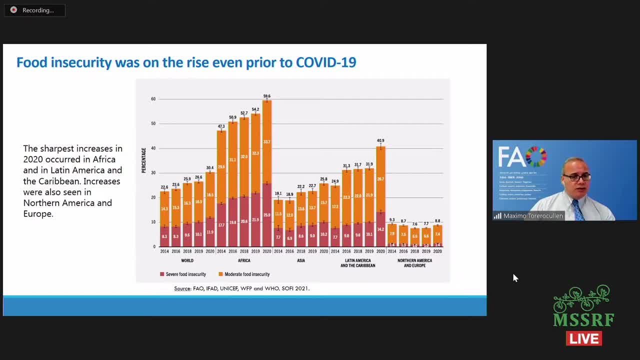 37 billion people did not have access to adequate food in 2020, including 60 percent of the population of africa. globally, this is an increase of almost 320 million people in just one year, and this is what we call the moderate and severe food insecurity. so together we had an. 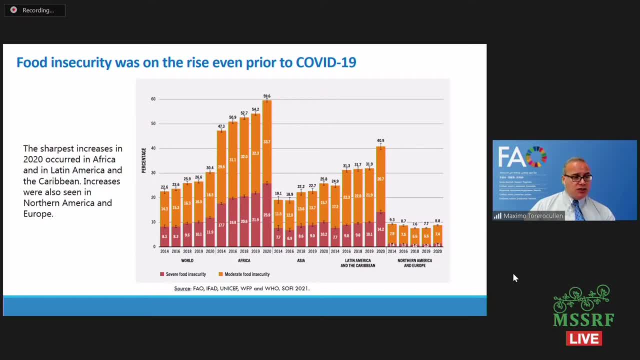 increase of 320 million people more in one year because access to diets could be lower quality of the diet or diets that don't comply with the minimum micronutrients that are required. prevalence of severe food insecurity also increased: close to 12 percent of the global. 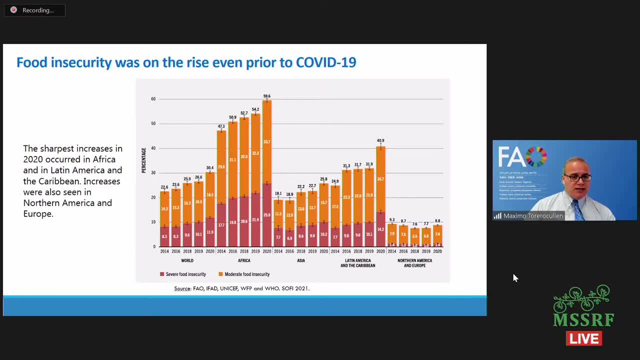 population was severely food insecure in 2020, representing 928 million people and 148 million more than in 2019, and the sharpest increase in 2020 happened in africa and latin america, and latin america was mostly affecting middle-income class, which move into poverty. but the gender gap- also of food insecurity- has grown even larger in the year. 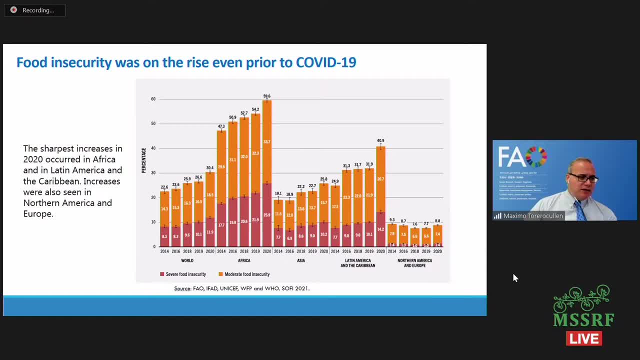 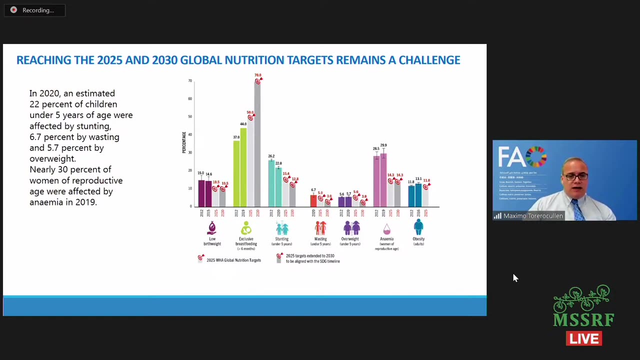 2019, because most of the jobs that were affected in the value chain were related to services, were related to packing, to transportation and other types of services, which are mostly concentrated by female labor. now, if we look at other dimensions, uh by 2025 of of nutrition targets, uh like low. 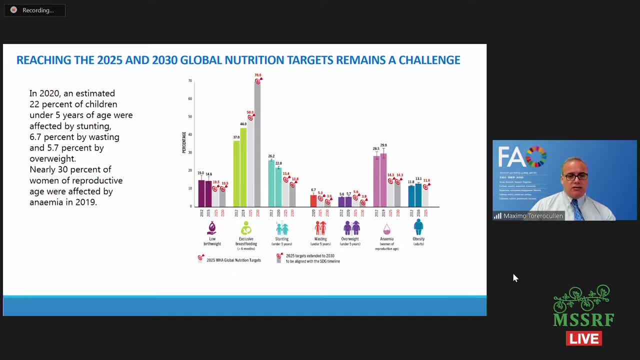 birth weight, exclusive breastfeeding. standing under five years, wasting under five years, overweight under five years. anemia. woman of reproductive age and obesity. although it is still not yet possible to fully account for the impact of covina gene pandemic due to data limitations, it is estimated that 22 percent, or 149 million children under 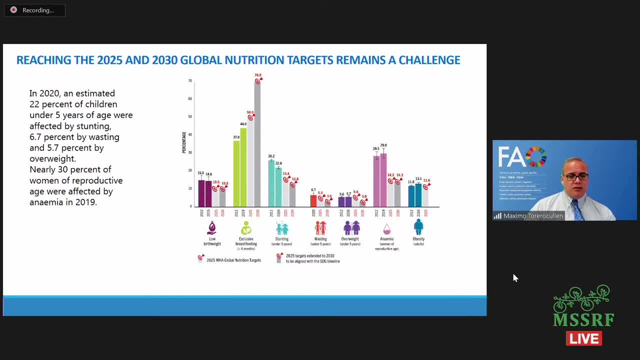 five years of age were affected by standing six point, seven percent by wasting and 5.7 percent by overweight. africa and asia account for more than nine out of ten of all children with stanting and more nine more than nine out of ten, more children with staining than children with staining. 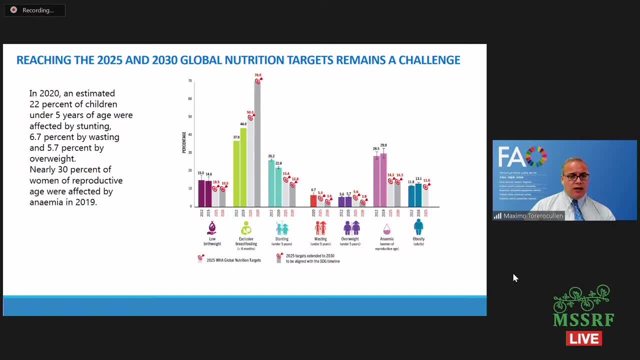 with wasting and more than seven out of ten of children who are affected by overweight worldwide. if i may just ask you to start coming to your country? yeah, i am already. i am 10 minutes, so i have four minutes more. no, that's what you. i have 15 minutes, up to what i understand. no, 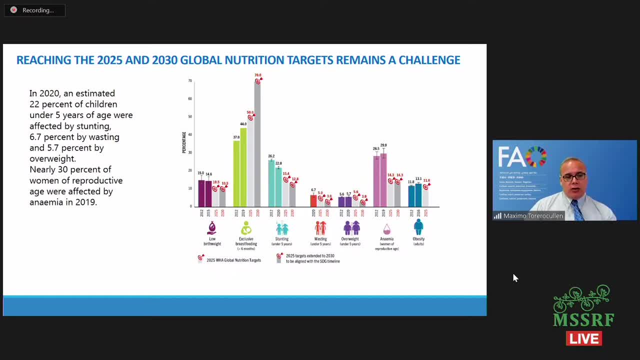 the organizer had said 10 to 12 minutes, so we can. okay, don't worry, so let me, let me, let me accelerate so that we can finish. so, basically, what i am trying to show is that the different indicators of nutrition are also affected. now this together is linked to increasing in prices. 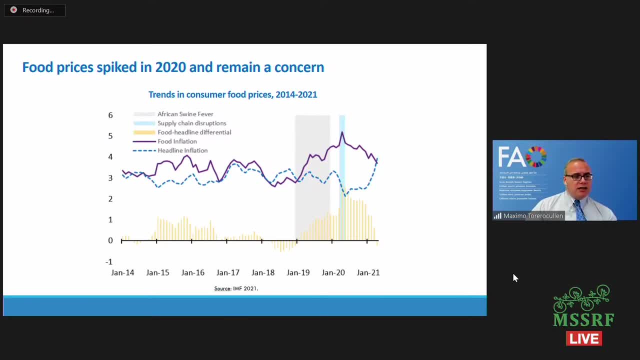 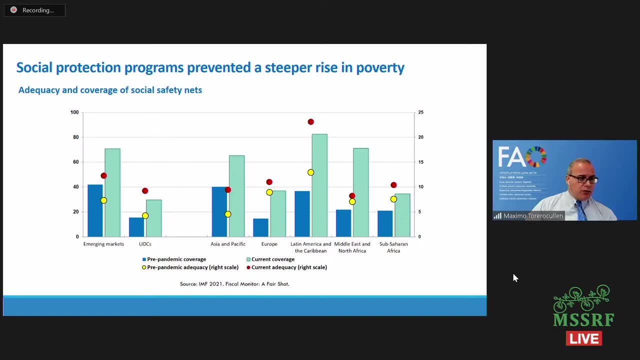 which have spiked and, as you can see here, this could lead into inflation in the world, which is something to to look at now. in this context, social protection programs have helped to minimize these, these problems, but again, one of the issues that we found in here in the blue bar you have the 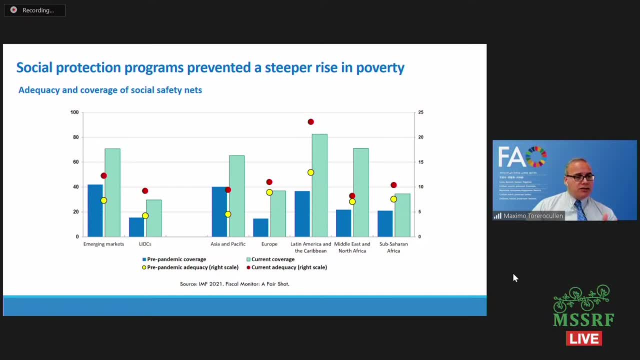 pre-pandemic coverage: light blue bar the current coverage and you can see how it has substantial impact on the health and well-being of the population and the health and well-being of the increase. but then you have on on the yellow circle, pre-pandemic adequacy. so it's the right. 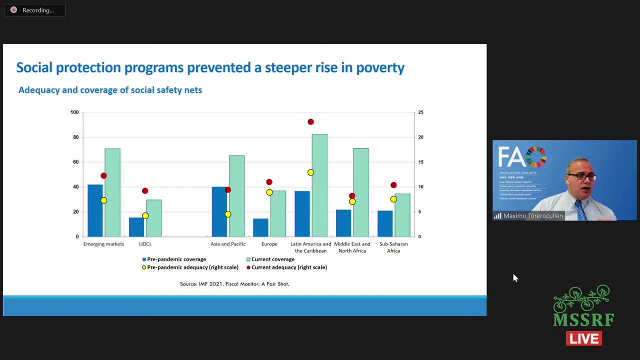 scale and the red circle the adequacy right scale. so how you increase in intensity- so it's not only coverage but also how you move from yellow to red- is how intensity of the program was done. one of the major issues we found in many of the regions is targeted. not all the regions were properly. 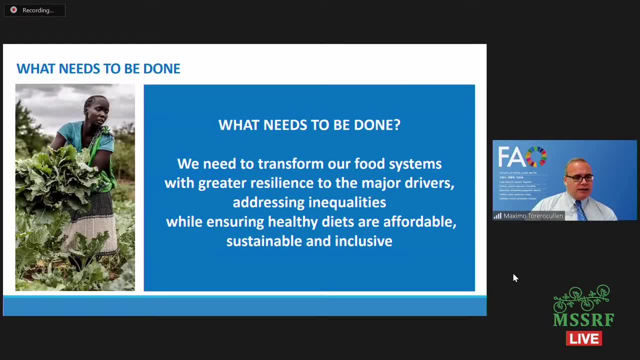 targeted, so that's something to look careful. so what needs to be done- and i am sorry, i thought i had 15 minutes, but essentially what we want is- is to increase resilience. okay, but increasing resilience will require two things. we need to increase the capability, so increase the 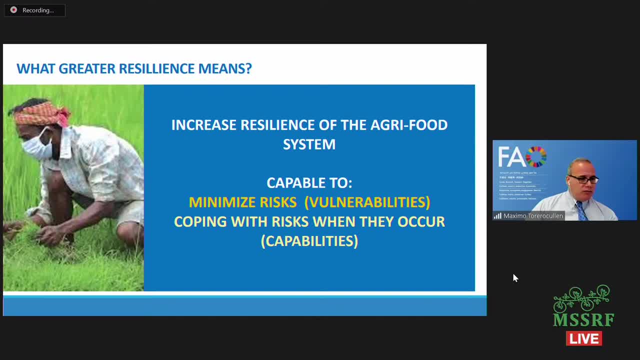 resilience of the agri-food system so that they are capable to minimize risks. that's vulnerability. for that we need early warning systems in place, but also we need them to increase how to cope with the risk when they occur, and that's capabilities now we have defined, after a huge process that we 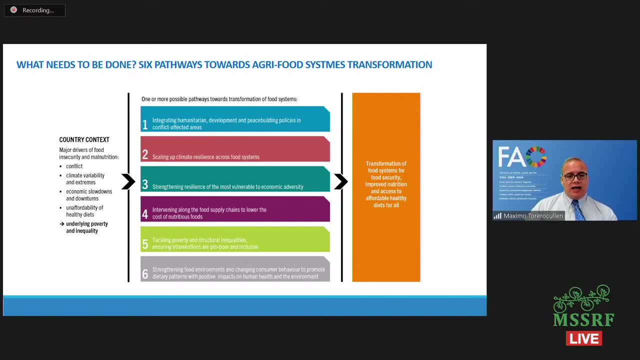 did for our sophie publication that, depending on the driver or combination of drivers confronting a driver, there are six pathways towards food system transformation that needs to be achieved and we list here the six pathways, and essentially every one of the pathways builds on key recommendations from an in-depth and detailed analysis and these transformative pathways are: 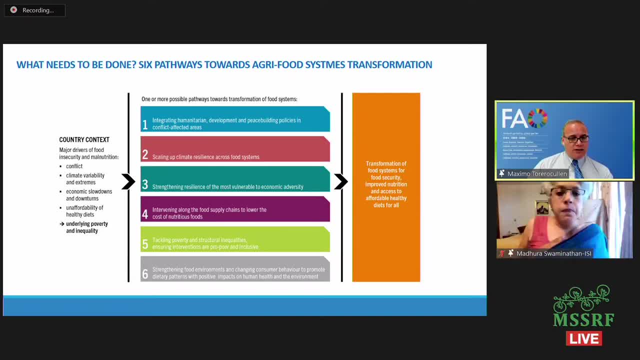 integrate humanitarian, development and peace building policies in conflict areas. scale up climate resilience across food systems. strengthen the resilience of the most vulnerable to economic adversity. intervene long supply chains to lower the cost of the nutrition of food so that we can reduce and improve the access to healthy diets. tackle poverty and. 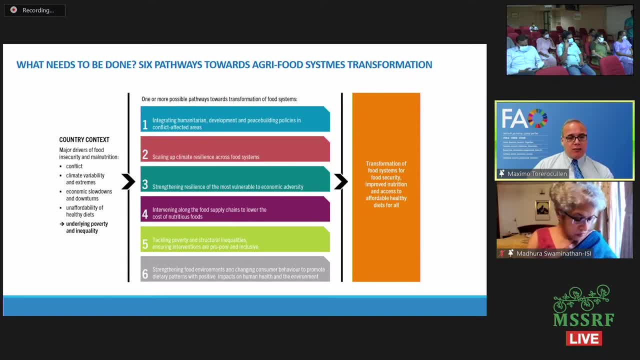 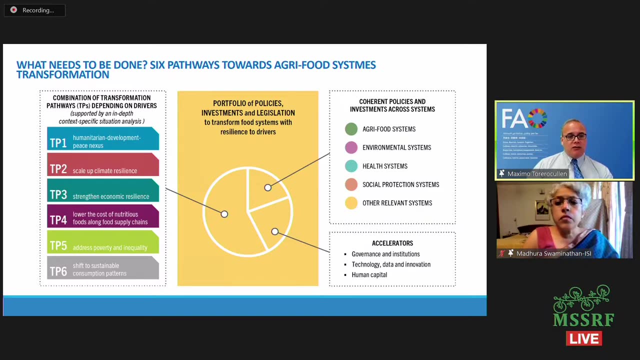 structural inequalities, like, for example, empowering vulnerable, marginalized populations and strengthen food environments and changing consumer behavior, promoting healthy diets. so also the behavioral part will be important, but the major lesson is that this cannot be done one by one in silos, but we need to find ways in which we can combine them. 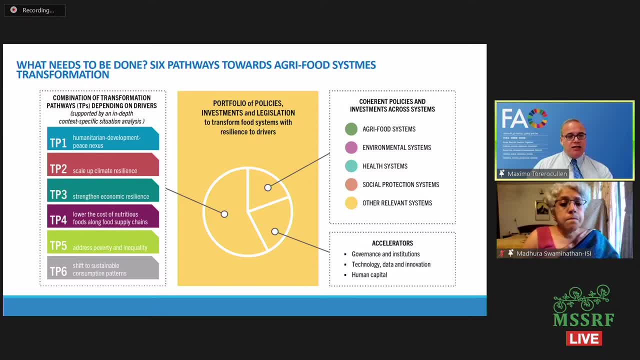 and try to bring compacts or packages of interventions that will give the highest return, because every country will have a different need and, based on the needs of the countries, we need to build coherent policies that will allow us to do that now. in that context, we believe that 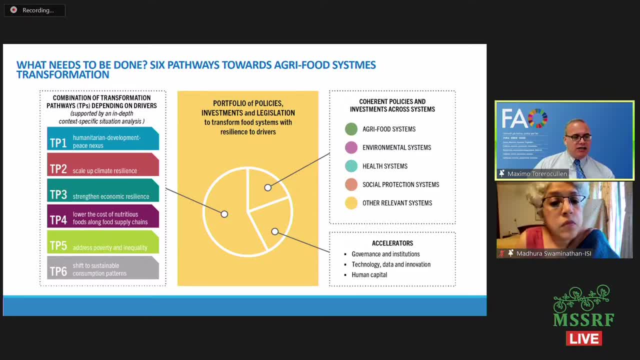 there are accelerators that need to be put in place, and these accelerators are in governance and institutions, technology, data and innovation. data has been crucial, especially for targeting and for giving proper information, but also human capital. we need to improve capabilities of human capital so that we can improve and get the benefits from this. 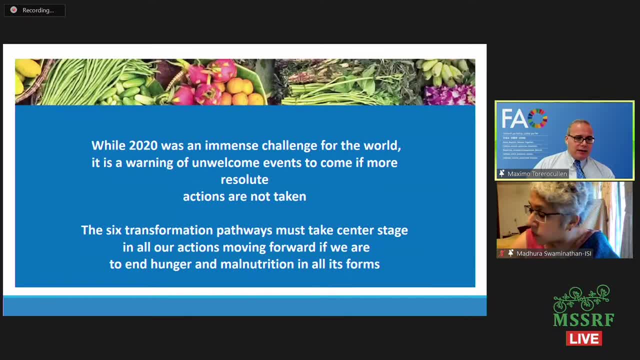 uh, different pathways. so at the end in 2020 was a huge challenge. it still is a huge challenge in 2021, but we need to figure out ways how, through these transformative pathways, we can make the change that we're looking for. apologies again for passing the time. thank you, no, no, thank you. 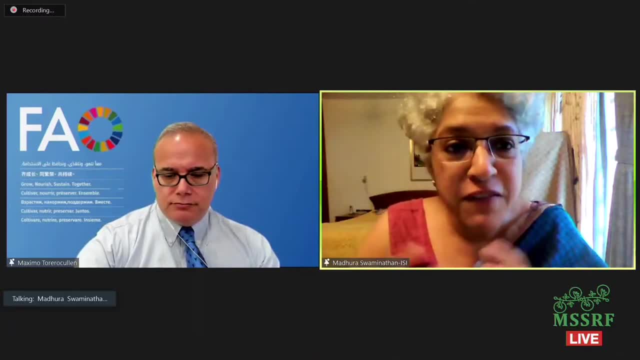 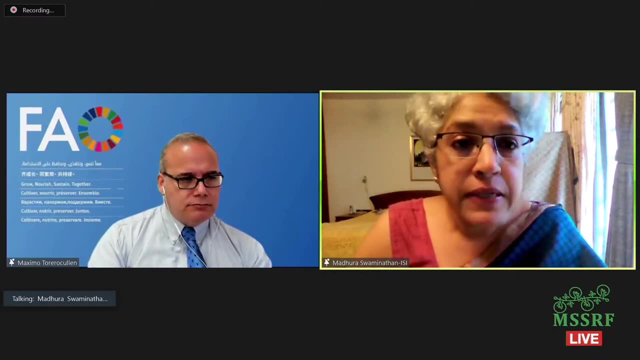 it's my mistake, and i think it was very useful, because you gave us, uh, not just the six pathways which we have been talking about since the morning, but uh how one combines those and what should be done in specific contexts, and i think that is a sets the. 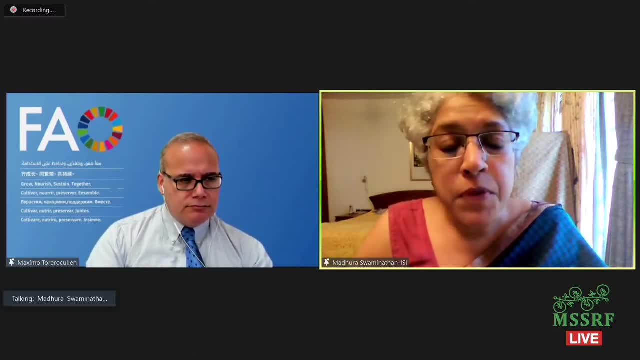 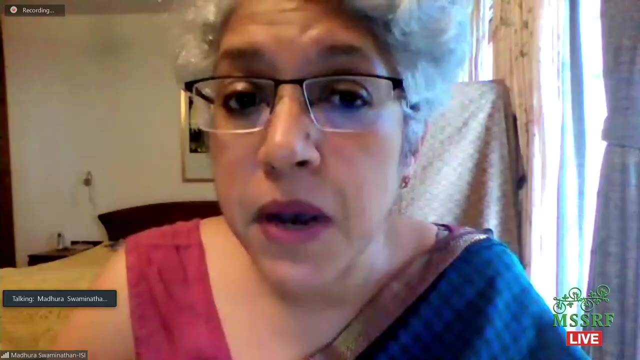 stage uh for the next speakers who perhaps will give a little bit more of country and regional focus to some of the uh issues that you have raised. i'm very happy to welcome next dr truan tuet mai, who is professor and vice director of the national institute of nutrition in vietnam. 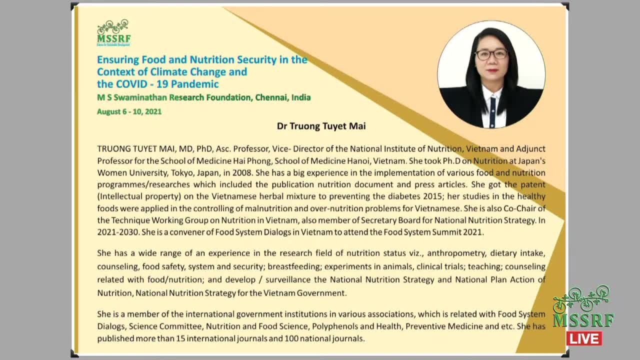 and she has been. she has had experience in implementing uh food and nutrition programs in for the government of vietnam, is a co-chair of their technical working group and is also a convener from vietnam for the food system dialogues that are part of the ongoing un food. 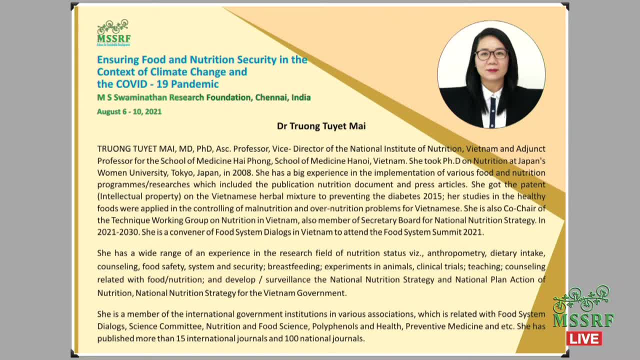 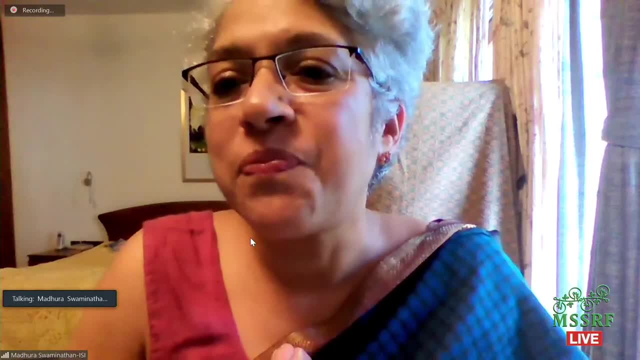 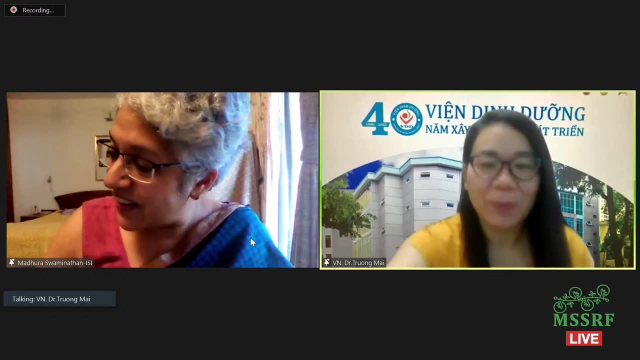 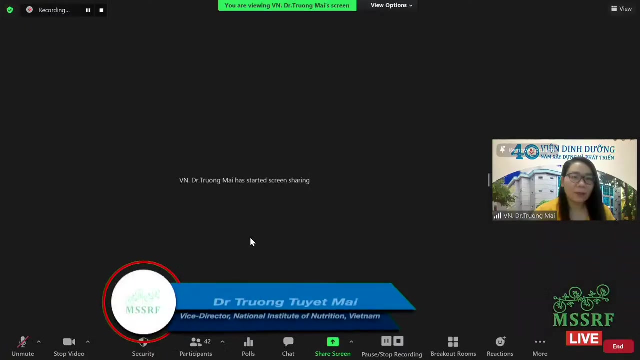 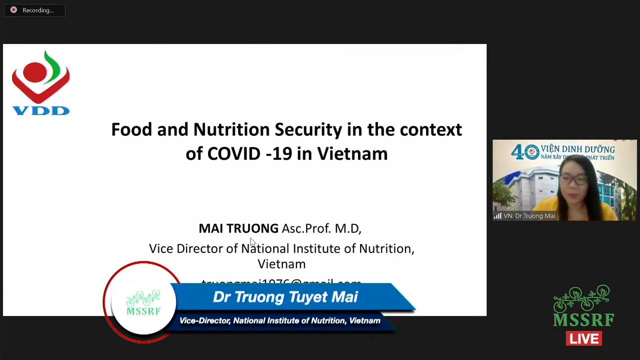 system. so i think we have a very appropriate person over to you, dr truan, and if you can try to give us your main points in about 12 minutes. thank you, yeah, good afternoon. yeah, everybody, yeah, sorry, yeah, oh, i can say in my presentation: okay, so i think i hope that i can do uh present, however, in the 15 minutes. yeah, okay. 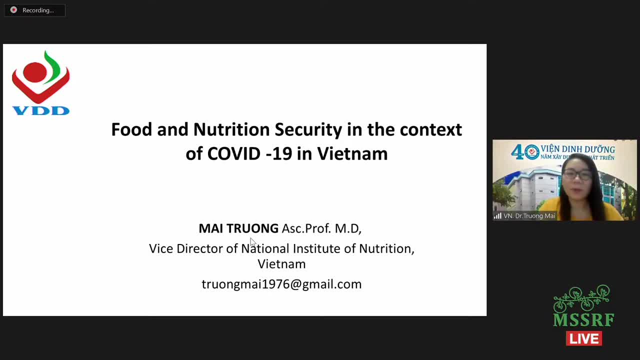 yeah, so is the first one i would like to thank you so much. in the mss, uh, i am in indian, uh, invited me to enjoy this decision. so, yeah, so thank you, madam chair. in the intuitive what, yeah, during the this morning and during this afternoon, i, i think it's a very night. 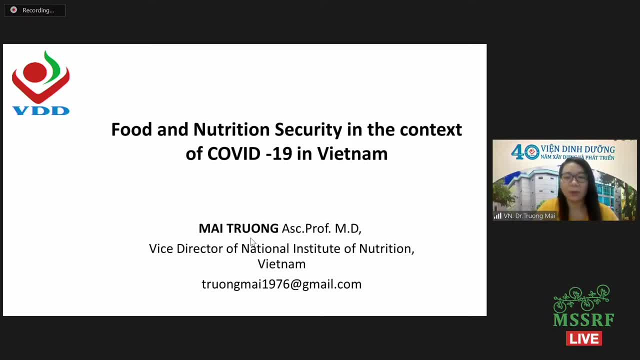 i heard uh from the many um um expert to talk about the issues related the food security and the nutrition security and almost the country and the one and has a concern, climate change, and also copy 19 uh epidemic with the effectively directly the agriculture production and food security and 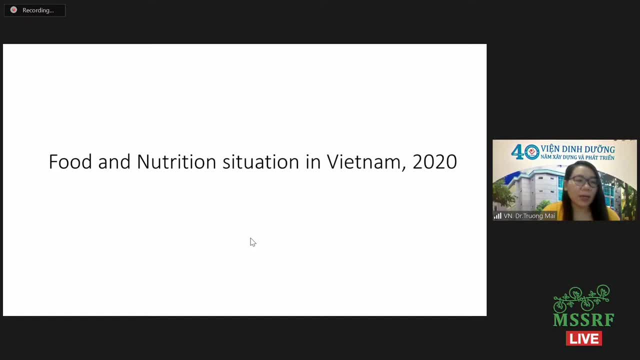 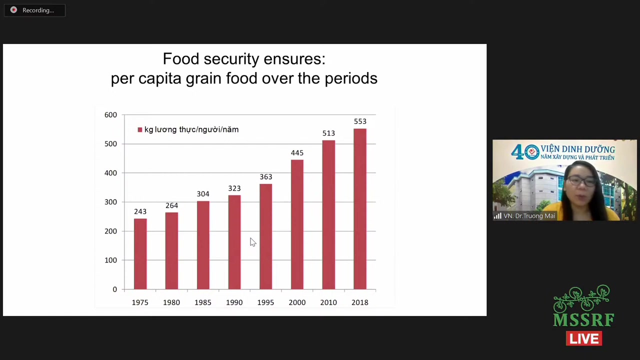 nutrition security. so i now i would like to say it use some the current food and nutrition situation in the vietnam until the 2020, especially during the coffee pandemic and climate change that has been taking place in the vietnam. so, as you know, vietnam population now it currently is a: 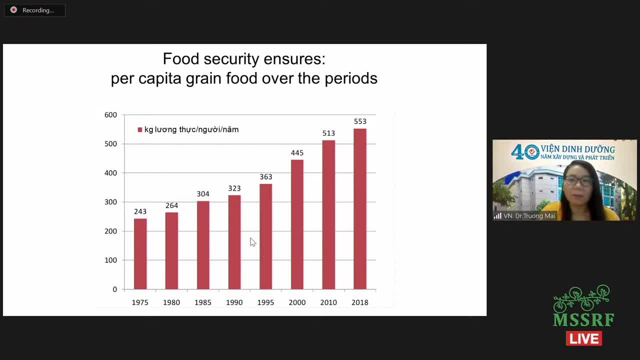 19, 7 million people, more than than 60 percent as a living rural area. in the vietnam food production uh has increasing by uh by year, uh in the cup. so now in the nearby the 600 kilogram food per person per day per year. 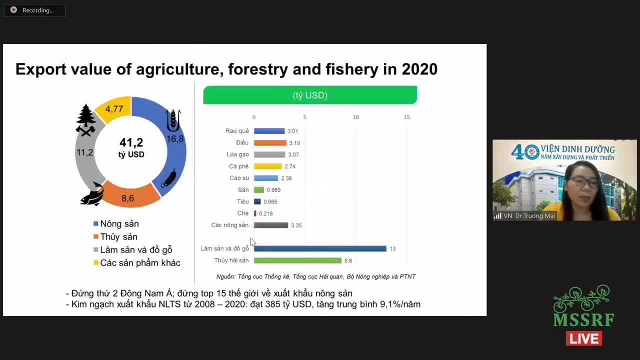 so i think uh, basically in the by uh 2000, 2020, the rate of the hunger is a very no, food security is almost guaranteed. basically, vietnam has also increasing by years the export a volume of the many agriculture foods, ranking second in the southeast asian ranking, the top of the 15th one for the agriculture products. 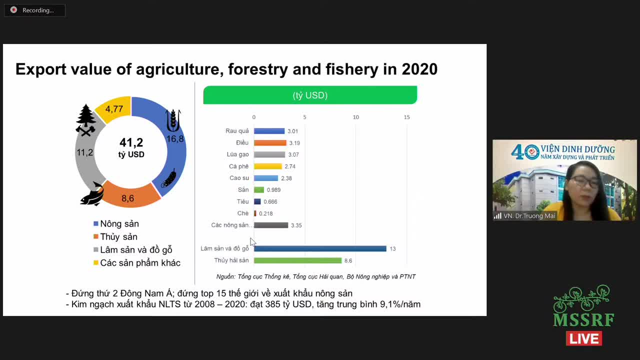 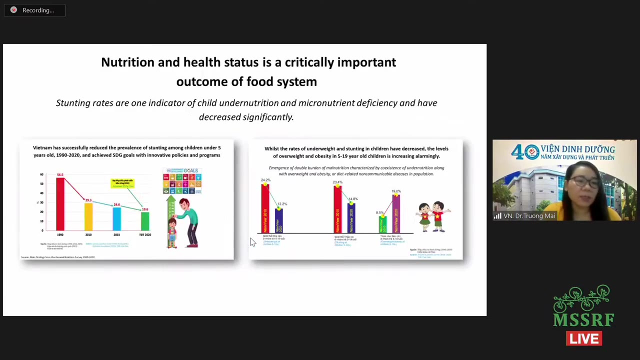 exports. so we turn over from the 2008 to 2020, reaching the model nearby the 400 billion us dollar and the increasing um by earlier, by the 10 percent. so, for the, in term of the logistics, and started in vietnam. now we have a facing uh double burden: nutrition, the rate of the malnutrition, uh, and standardWhen we are in vietnam side market situation, we're really considering for food networks, increasing food for theouting issue, no, China actually well, is going to. they were vinod world, uh, same thing you can understand. but oncology should, but probably be, was it hundred-ium system? but i mean it's like a little bit different here and it's a little different from um. i mean like um, the labor market, but um, they say itself. and exploration, um, uh, its. 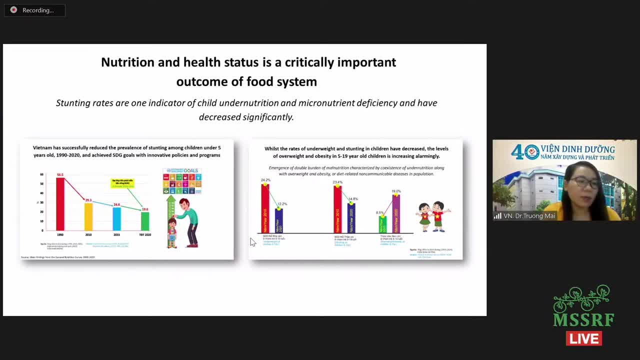 the還有 rồi m' ek phó. 12, Sri Lanka. what Type 1GI classimes already established a double-bard nutrition rate, more than 500 hundred billions below land battle nutrition um. right now we have increasing number of the nutrition level and from dribbling we have context quicker than sichuanтакkat. 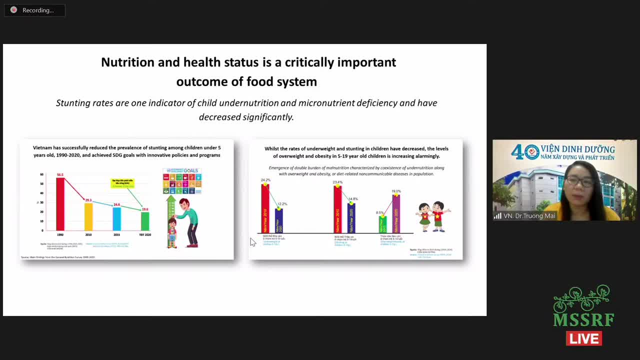 stunting children under five is about 20 percent, but the rate of the overweight and obesity in the children five to 19-year-old increasing by the two time after the 10 year and current about the nearby 20 percent. However, this poverty is a very big problem in Vietnam. 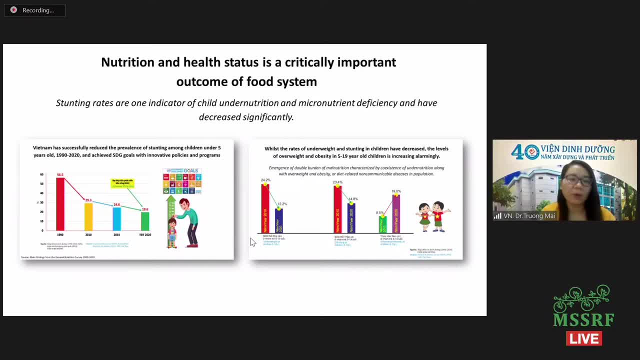 The rate of stunting among children in the ethnic minority and the mountain lot area is still very high, around the nearby 38 percent, but the rate of the overweight and the obesity in the school children increasing sharply in the city area about 40 percent. 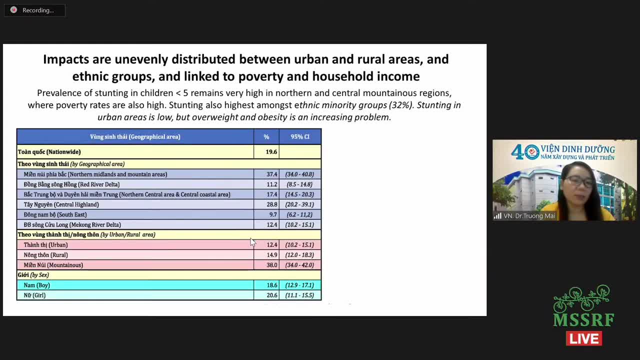 The problem of micronutrient deficiency and the sub-element and the sub-element and the sub-element drink deficiency and vitamin D deficiency is still very high, especially children and pregnant women in the mountain lot area, in ethnic minority. The prevalence and the overweight and the obesity. 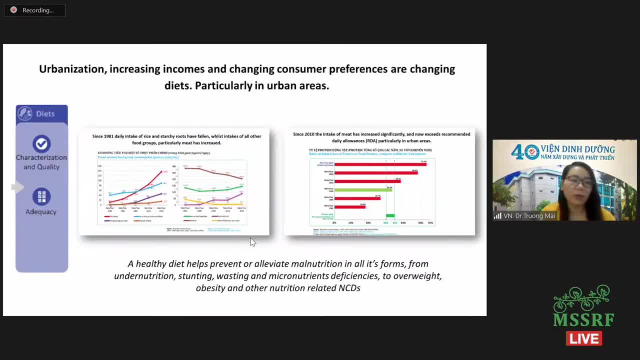 in the non-prevalent chronic lung communicable disease is rapidly increasing in Vietnam. So I So, besides that, the issue of the food safety is also a very big issue in Vietnam. So it's the government is to continue to control. 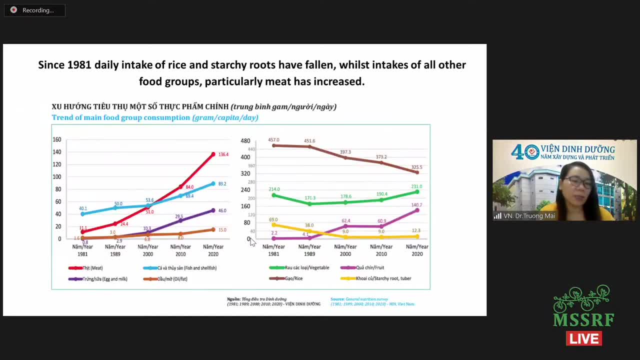 Deciding the food consumption. there have been reviews increasing the consumption of meat and seafood after the 10 year from the. from the, Especially in the urban area, the people consume more than 150g of meat per person per day. consumption of bread table and food increasing, but the consumption of rice has tend to go down. 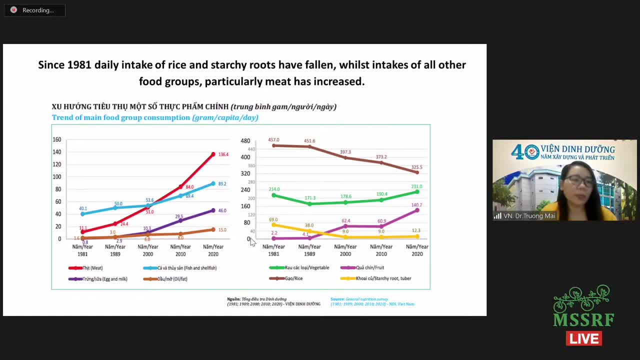 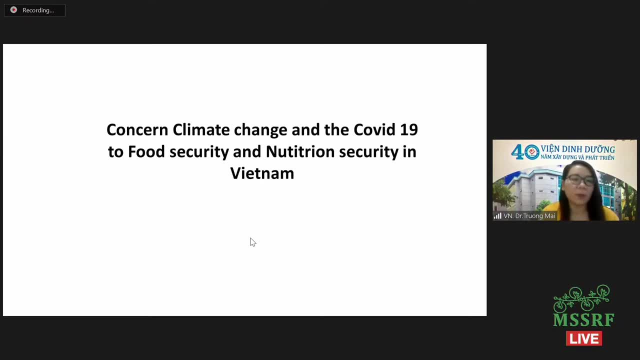 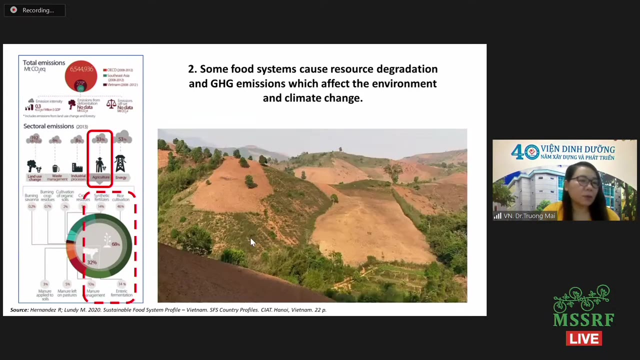 Now I would like to talk about some information about the picture of the climate change and the COVID-19 to the food security and the logistics security in Vietnam. Vietnam is located in the South East ASEAN. It is one of the countries in the world. 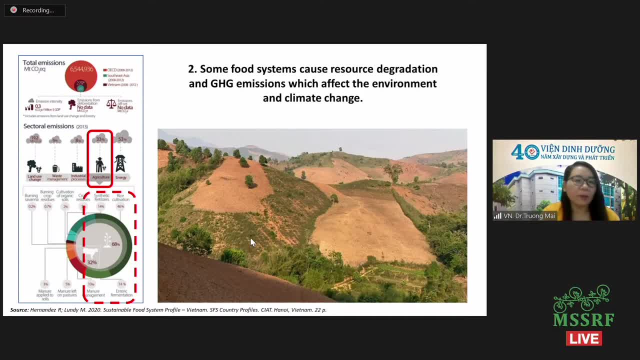 It is strongly affected by the climate change. Every year, Vietnam is affected by the many storms, floods and droughts During the period. the food security problem is occurring in many places. So you can see in the picture to talk about the problem of the soil: erosion and degradation of soil and saline. 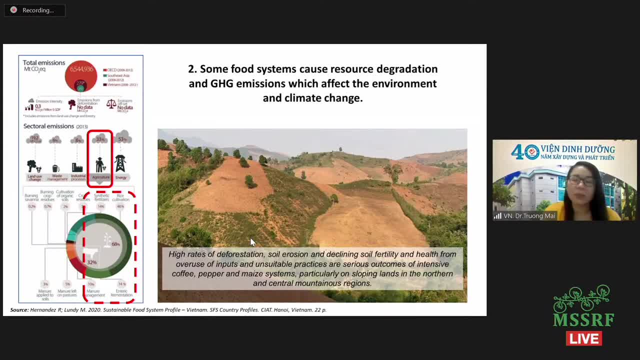 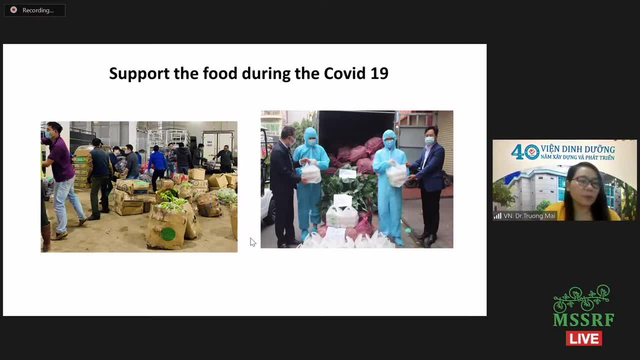 Saline in China. Saline has been affected by the agriculture in Vietnam, So now Vietnam has been facing a big wave of the COVID-19 outbreak. So during the three months until now we have had more than 200,000 cases. 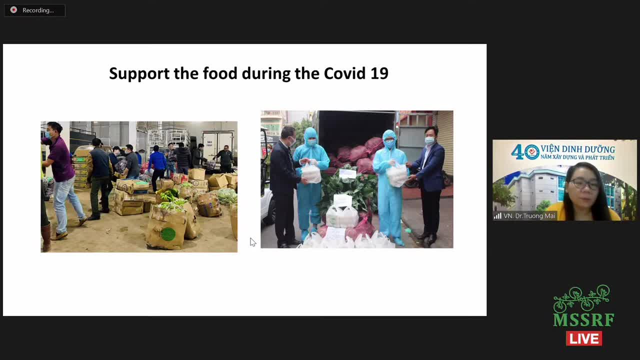 and more cases of COVID-19 and more than 3,000 cases of diabetes. So now more than 20 province out of 63 province in Vietnam is in lockdown, is very greatly affected by the product food and disrupting for the transportation of the food products. 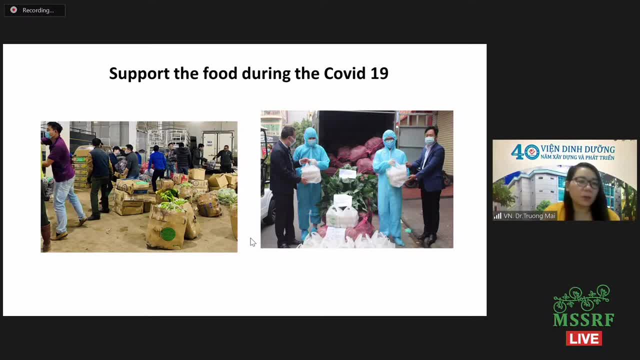 So the income and the living standard decrease by time. affected the access of food, affected the people's nutrition, So especially the children and women, especially in the poor area. so you can see in some picture I would like to show you to talk. 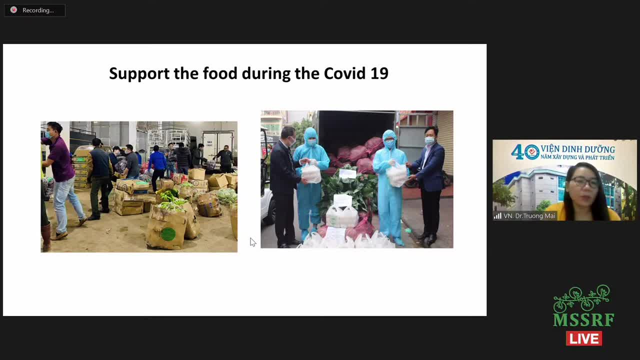 do you know in the Vietnam people now we have to how to transport for the food go to the lockdown area. So very difficult for us now to do the action, how to keep the food And the people do not hunger and to let the people do not lack of the food. 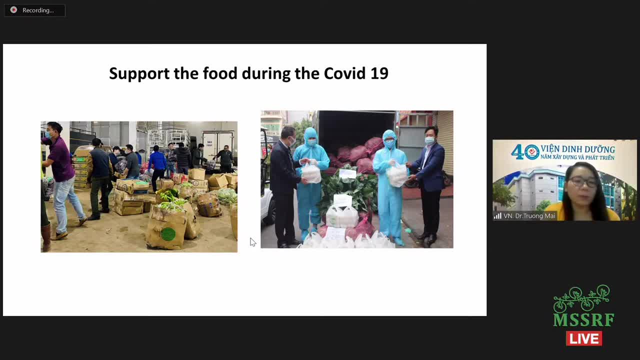 So if the block period is prolonged it means certainly has been impact in the food security and nutrition. So but now, until now we don't have any investigation, research for to talk about the how impact of the COVID-19 to the food security and nutrition security. 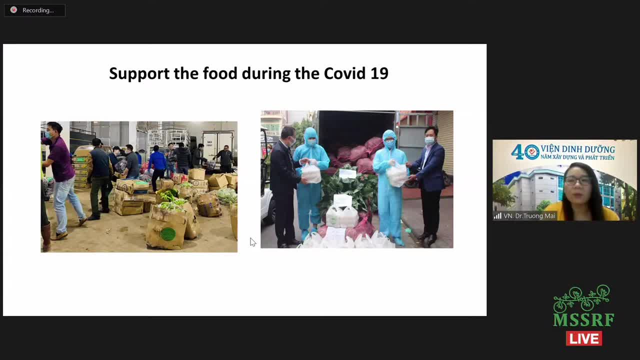 So but I think in the, if the continue in the, of course the Vietnamese people in the affected by the food security and the nutrition I think is going to have problem. So now in the Vietnam, so in the Vietnam government. 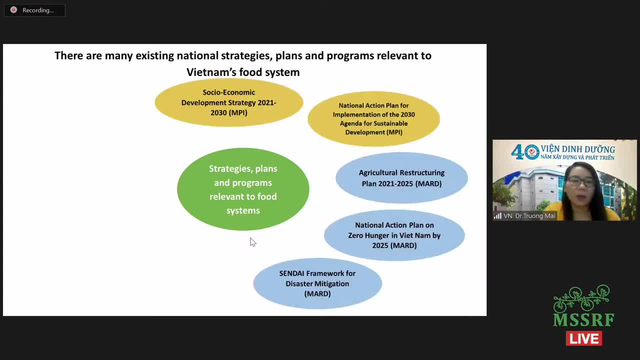 it has a many support package, food for the people. many place to provide the food support and the ensures the low one, low one people to hungry and the lack of food. So I would like to show you to some action for the Vietnam government. 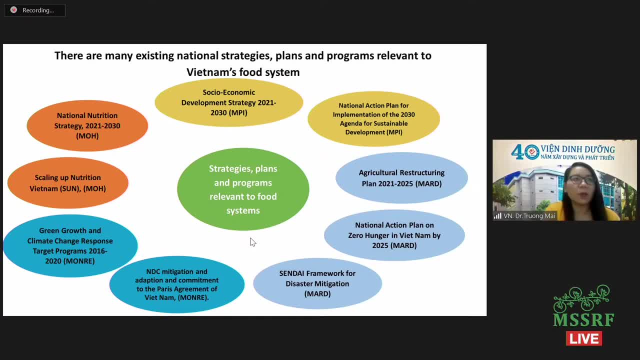 to continue to improving the food system in the Vietnam. So, as you know, in the this year Vietnam participates the UN for the food system, UN, UN food system submit. So the government has to make the commitment to address the issue and the gap and the channel in the Vietnam now. 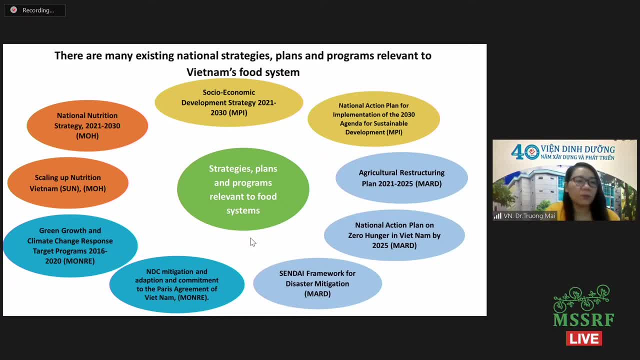 So in the move towards the sustainable and transparent food system in the Vietnam in the next 10 years. So you can see in the many statutory and action, in the coordination from the many ministry, from the government to action for the how to sustainable for the food system in the Vietnam. 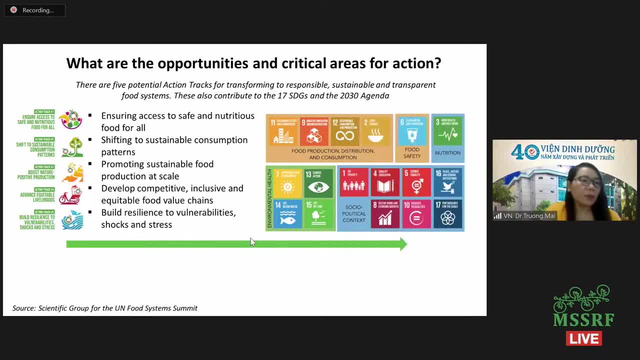 So in the, so the you can see in the some of the: what, the opportunity and the critical area for the action in the Vietnam, how to improving the food system in the Vietnam for the transformation and the two. two action for responsibility and the sustainability of the food system in the Vietnam. 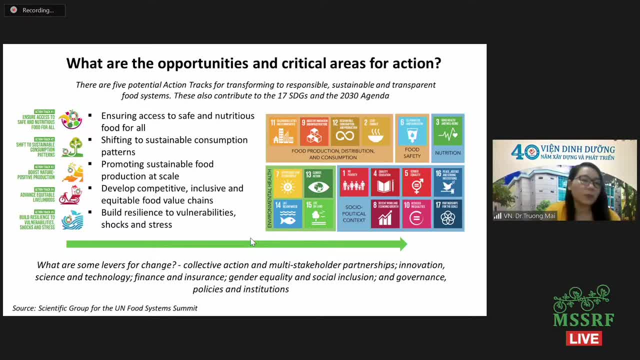 So we have to go to the to accept the SDZ in the 2030.. So but I think in the, maybe in the COVID-19, and the climate change is in the Vietnam, So we hope that the Vietnam government. 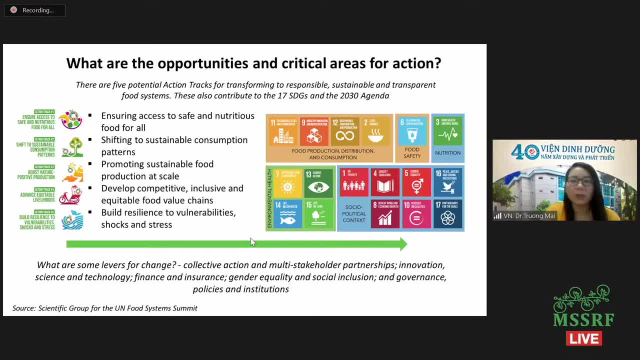 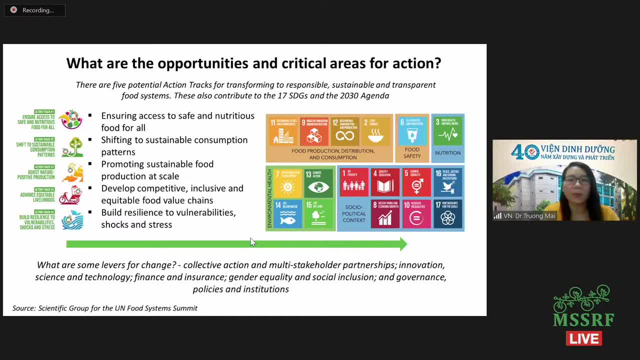 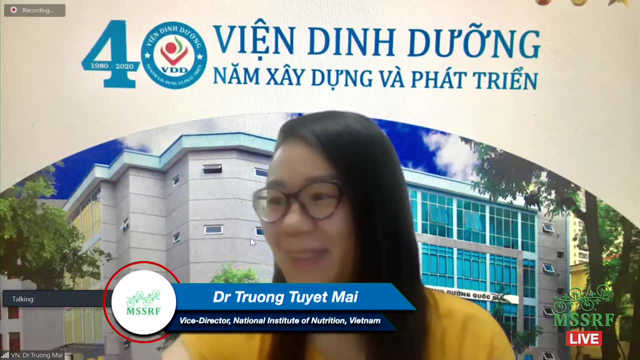 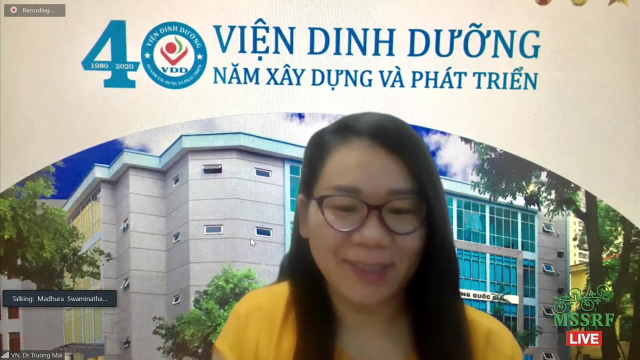 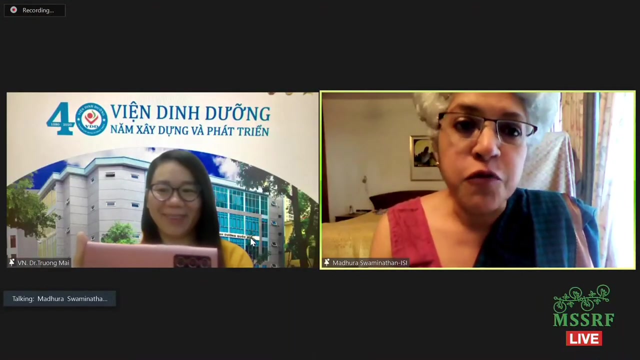 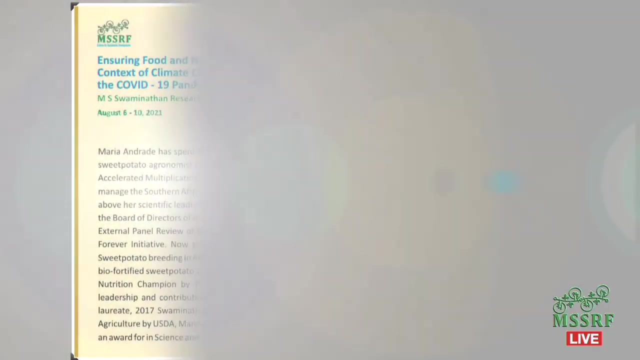 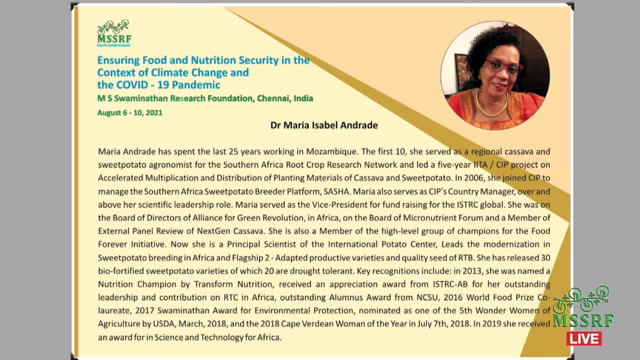 who would have been with us, I think, if it hadn't been for the pandemic? Maria Andrade is a principal scientist at the International Potato Center, SIPP, working based in Mozambique. We seem to have a Peru connection in the presenters today. She has been a pioneer in 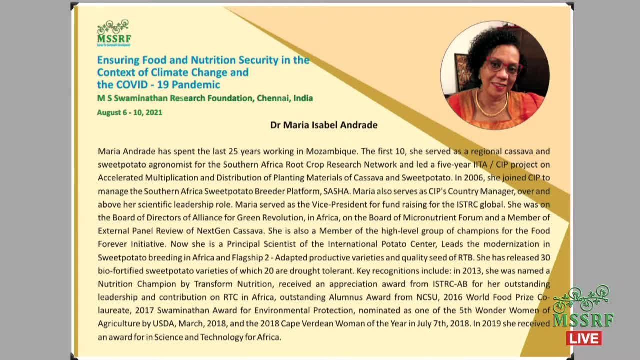 and a major propagator of biofortification and, in particular, a leader in sweet potato breeding in Africa, elsewhere, and has been recognized globally for this work. in 2017, she won the world food prize. uh. she has won the swaminathan award, which is given every year in chennai at the same day, august. 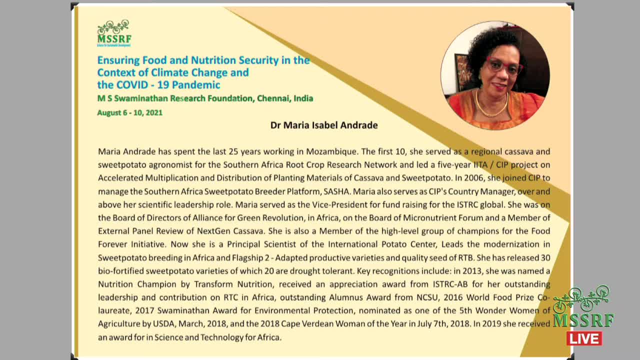 7th as our founders day. uh, she was the woman of the year in 2018 and has received award for science and technology in africa. she's on many committees and commissions now, uh, which uh mean i will not go into in detail, uh, because i want to give more time to hear what uh maria andrade has to say, so welcome. 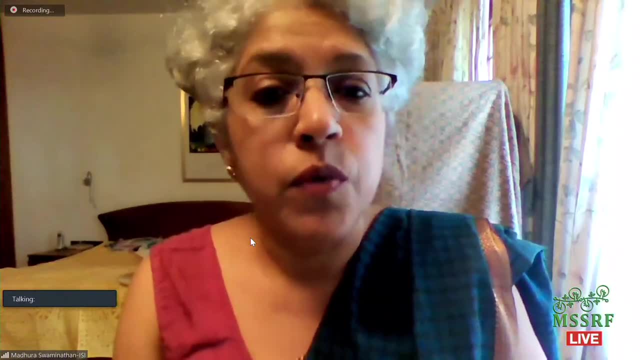 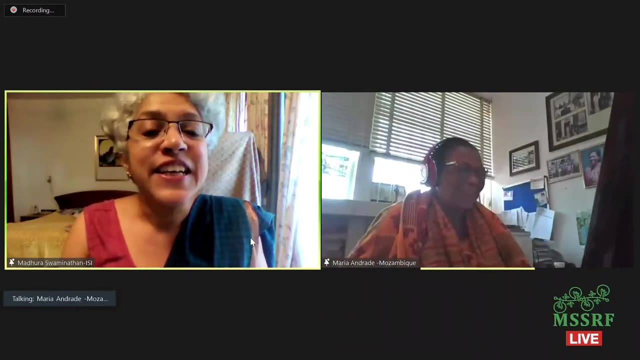 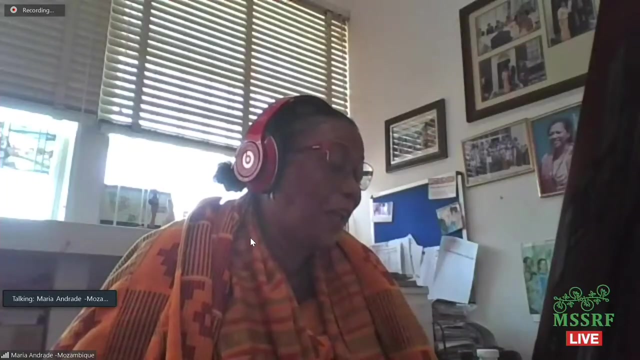 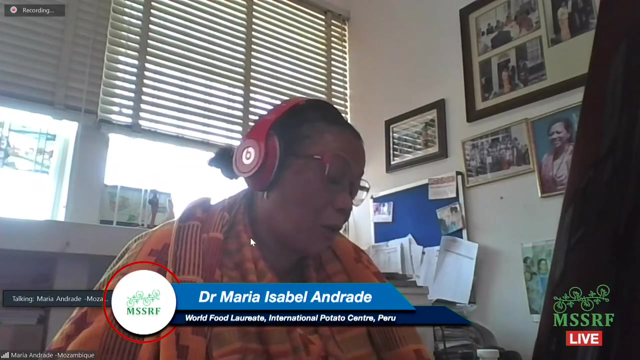 uh, maria and uh, where is she? we can see you in your bright orange welcome. yeah, thank you. thank you, madam chair, for this very beautiful introduction, and also i would like to thank you for this opportunity to be able to give my view on this conference. i ask somebody to help. 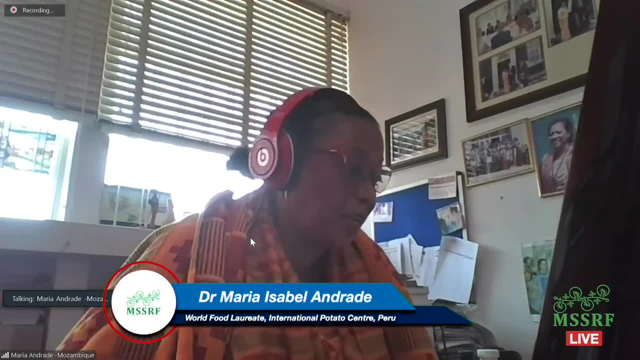 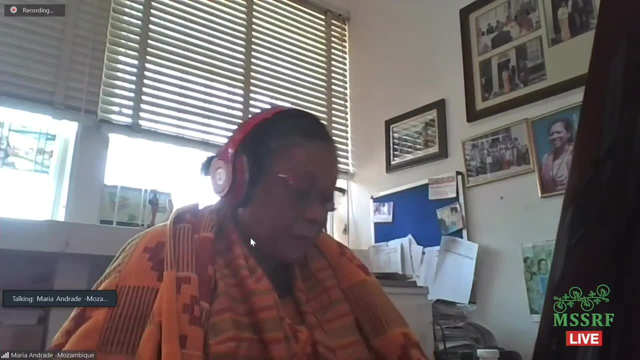 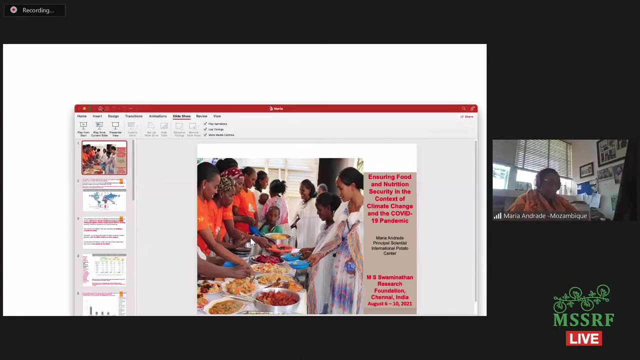 me out with the glue the presentation, because for my side in the net i have been very slow, so can i help to get my presentation on? we are sharing them, we are sharing, thank you, thank you. so, like i said, it is a pleasure. can you put it in the slide mode please? 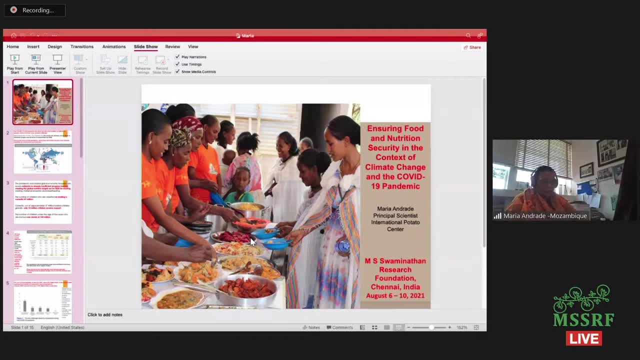 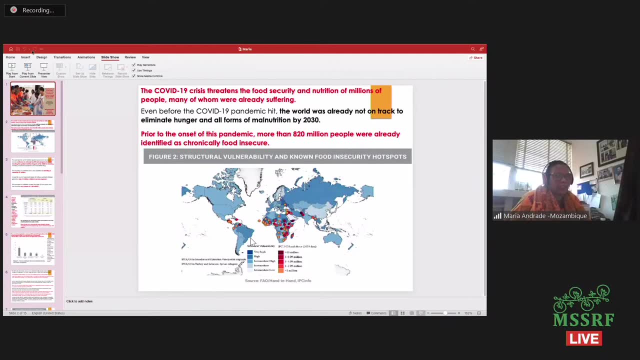 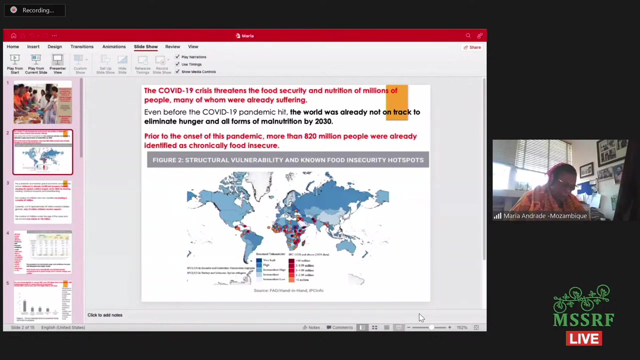 okay, let's let it show a slide show mode, please, please. thank you. so so this is all about ensuring food and nutrition security in the context of climate change in the convict comedy pandemic. So we heard very much through the first speaker, a very outstanding presentation. As you know, the COVID-19 threatened food security and nutrition of millions. 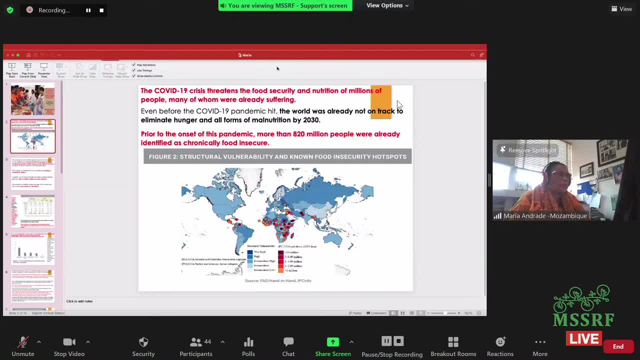 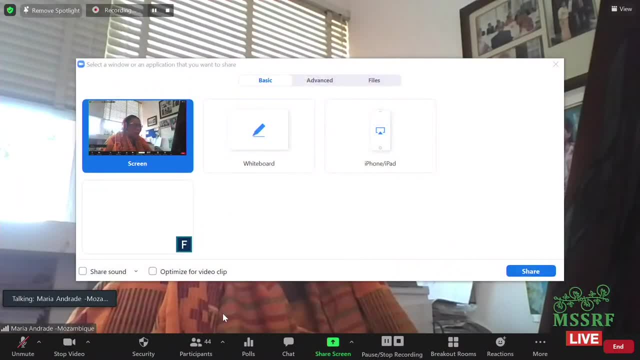 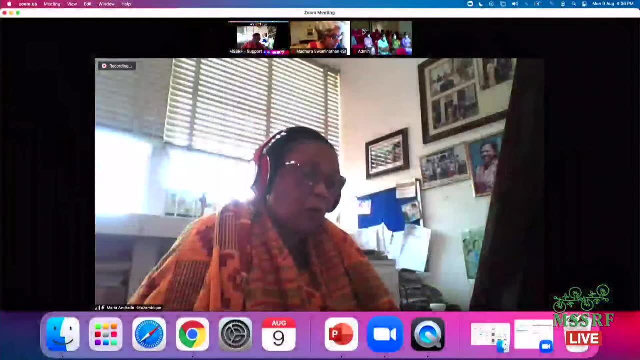 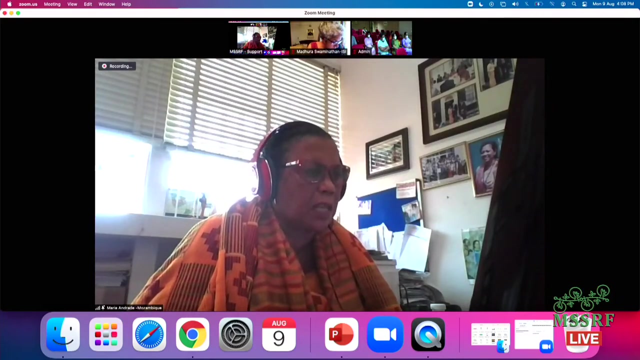 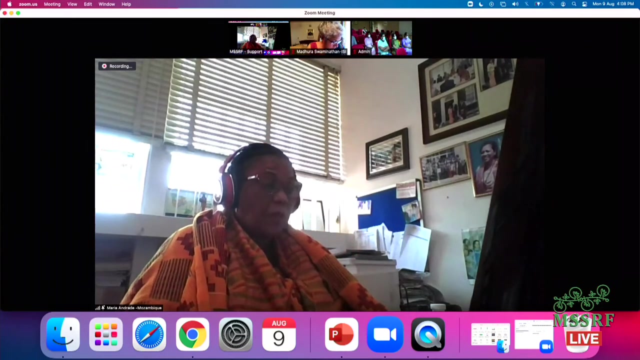 However, when COVID-19 pandemic hit, the presentation went off again. But when COVID-19 hit, the world was already not on track to reach what you call the Sustainable Development Goal 2,, which was to end hunger and all form of malnutrition. 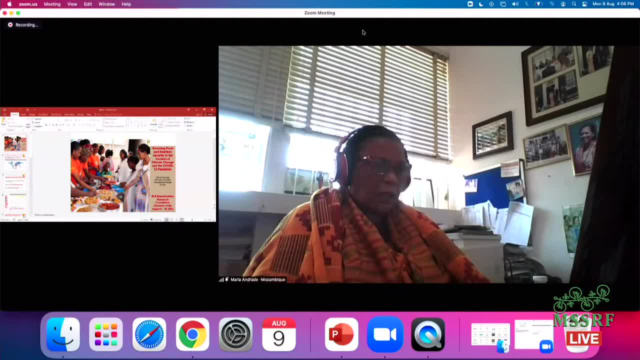 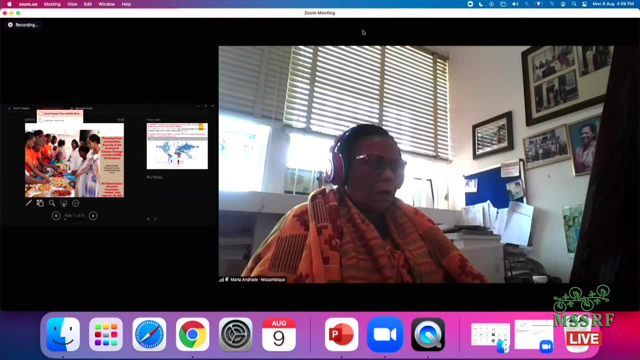 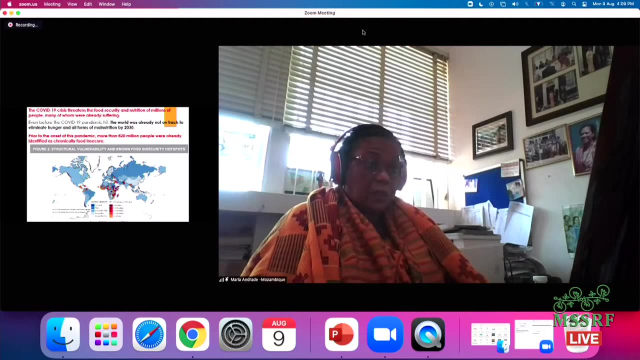 I cannot see my slide. Is that okay? Okay, They have just come back on again. They have just come back on again. Yes, Next slide, I think Yeah, Next slide too, please. The second slide, Please. 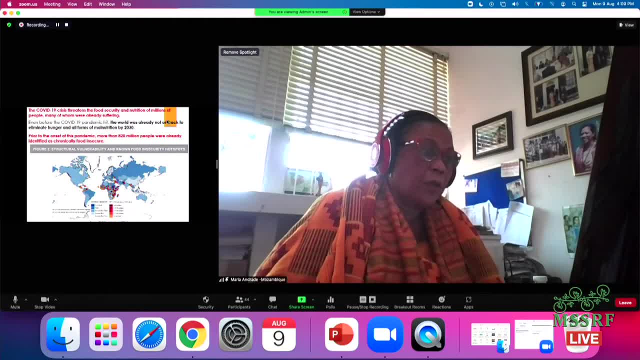 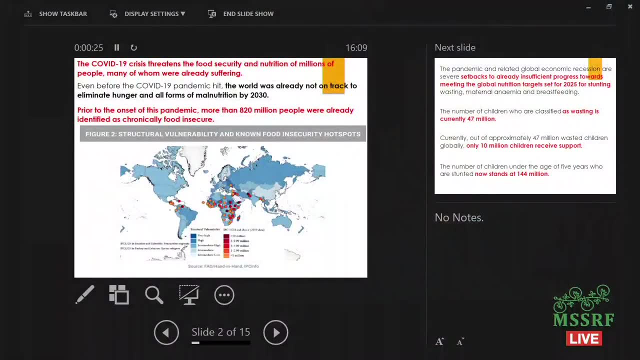 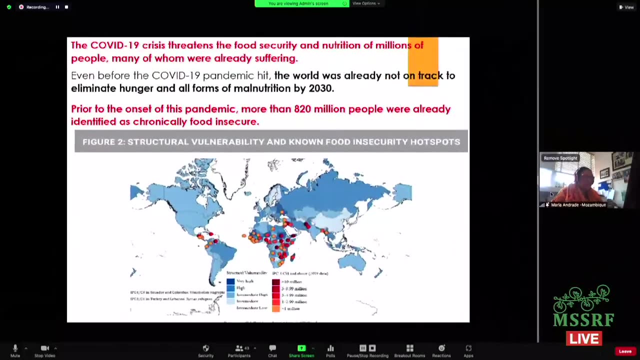 Can you move the slide? Okay, Okay, Second one. So, if you see, prior to the onset of the pandemic, more than 820 million people were already chronically food insecure. And if you see through this graph, Okay, most in Sub-Saharan Africa and South Asia are the places where were more affected. 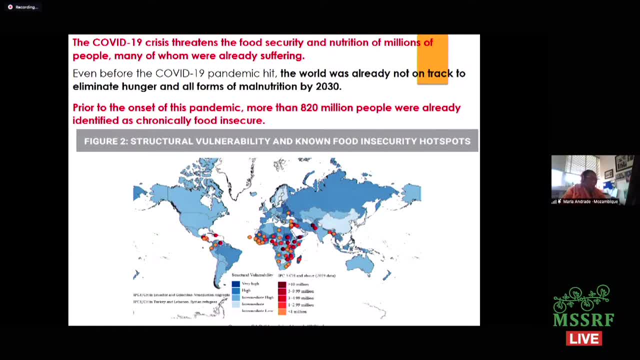 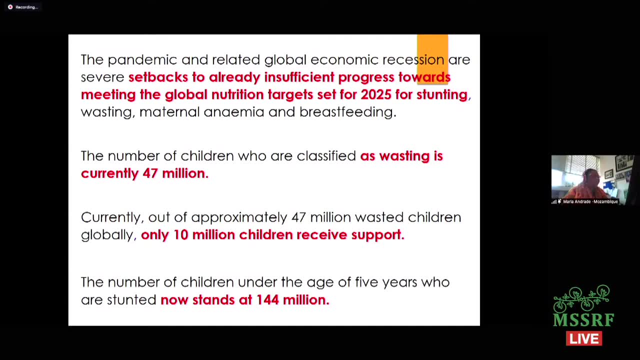 They were more vulnerable for food insecurity and malnutrition. Next slide, please. So if you see also the COVID-19 through the first presentation are a very severe setback towards global target on nutrition. So if you see also the COVID-19 through the first presentation are a very severe setback towards global target on nutrition. 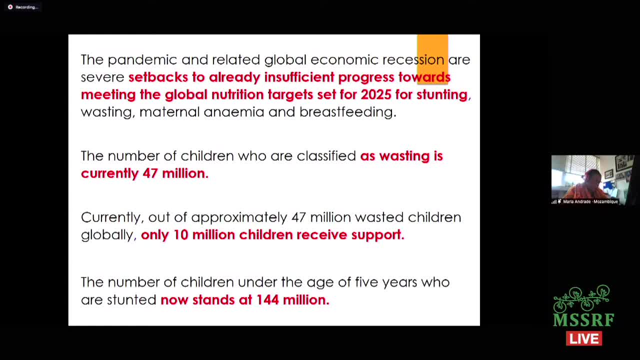 Again for 2025, which has something to do with stunting, wasting and anemia and breastfeeding. If you see, the number of children who are classified as wasting is currently 47 million, But only 10 million children receive support. The number of children under the age of five who are stunted are 144 million. 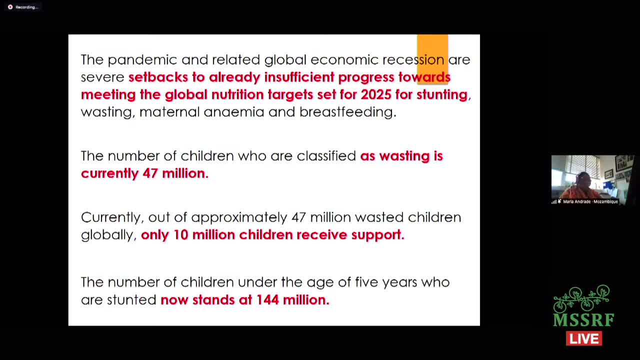 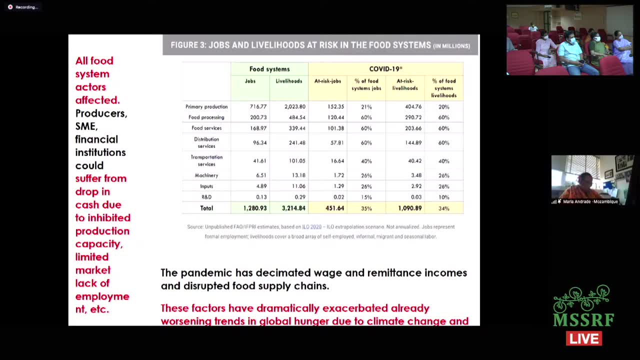 Next, please. So if you see, with COVID-19, all food system actors are affected. Job were affected, livelihood were at risk, Food system, food production, processing, transport, they were all affected And the pandemic has decimated wages and remittance of incomes. 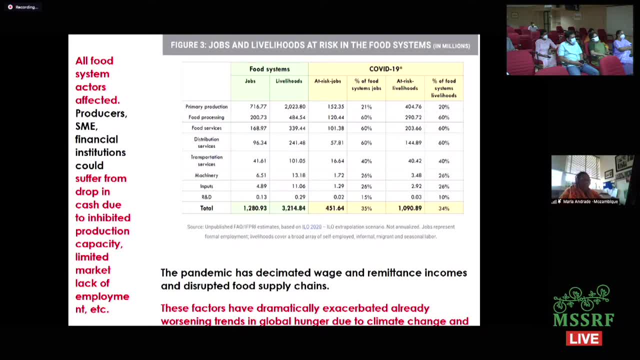 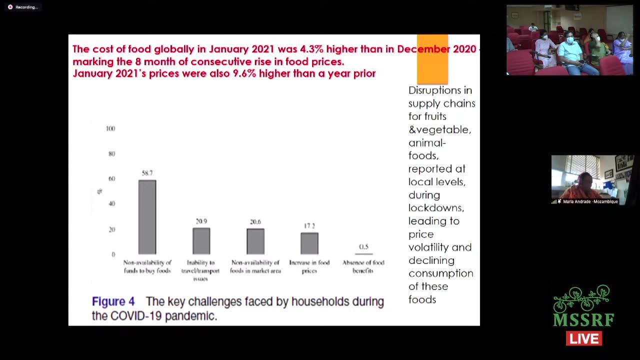 The whole food supply chain. This has already dramatically exacerbated what was already in place. Next, please. So if we look into this graph, we can see that with COVID-19, availability of funds to buy food, availability to travel and the transport was also an issue. 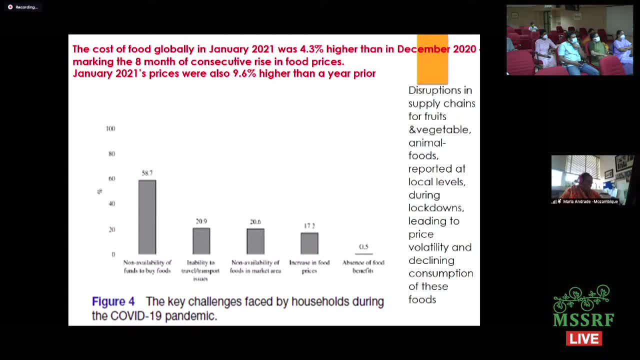 Also, food in the market area was very limited And, to make it even worse, there was even an increase in food price And in some countries also there were also absence of benefits. So we can see that the cost of food globally by January 29 was 43% higher than in December 2020.. 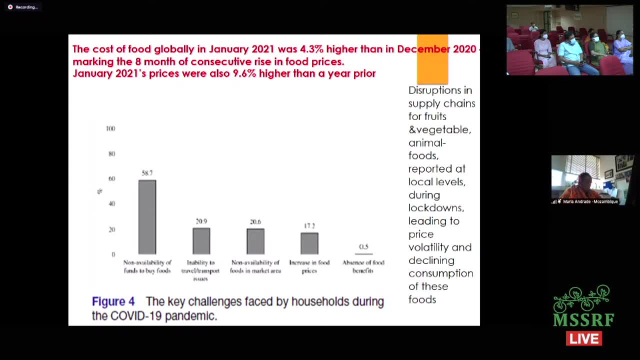 And also, if we see, in January 21, the prices of food was 9.6% higher than the year before And this is a real problem because the whole supply chain is disrupted. Fruit and vegetables and animal food source at the local level were very low during the lockdown. 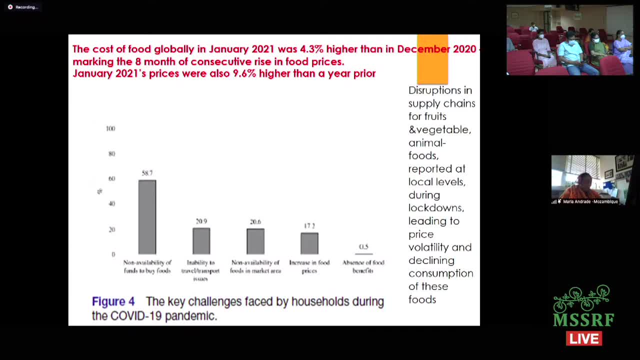 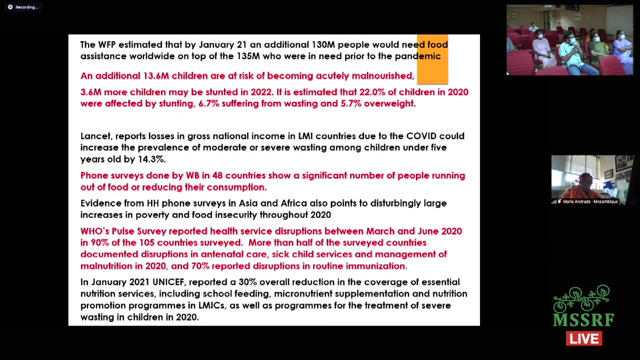 And this is leading. this has led to the viability And declining on consumption of this food, which is a problem. Next slide, please. So all these confirmed in the report- you have the report of World Food Program- that there is an additional 130 million people who need food assistance worldwide. 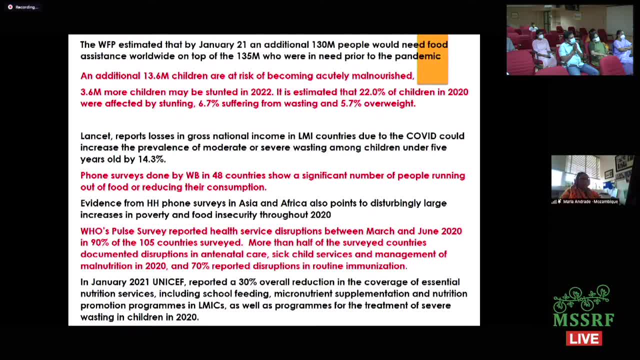 on the top of the 135 million that were in need prior to the pandemic. 13.6 million children are at risk to become acutely malnourished, 3.6 more children may be stunted in 2022. And it is estimated that 22% of children 22 in 2020 were affected by stunting. 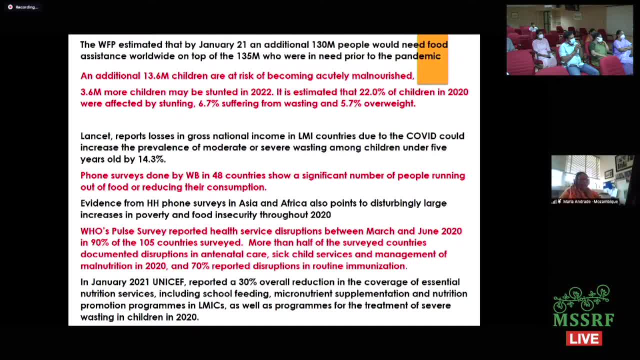 6.7 suffering from wasting and 5.7 overweight. This is a real problem And around you see. the Lancet is also saying that the prevalence of moderate of severe wasting among children under five years old at 14.3% is very big. 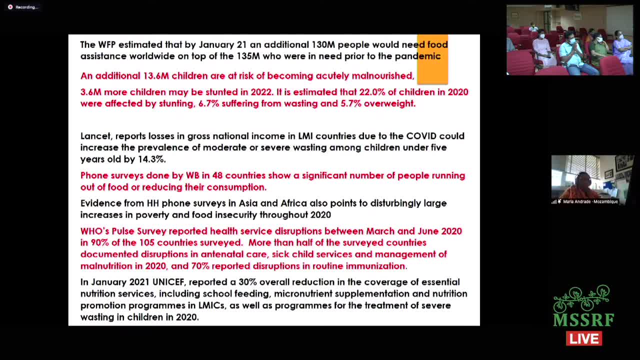 Surveys done by the World Bank in 48 countries show significant number of people running out of food or reducing their consumption. The survey done in Asia and Africa also show increasing disturbance, large increase in poverty and food insecurity. Survey with all the health organizations I mean give you in 105 countries. 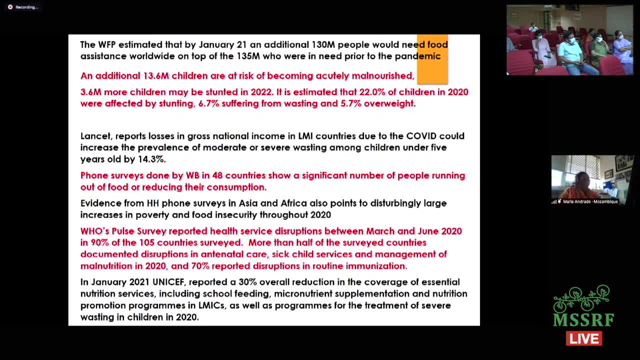 show you similar picture, But on the top of this, disruption of the health system and anti-natal care, sick child service and management of malnutrition in 2020, and 70% report disruption in routine immunization. UNICEF also is telling you the same thing. 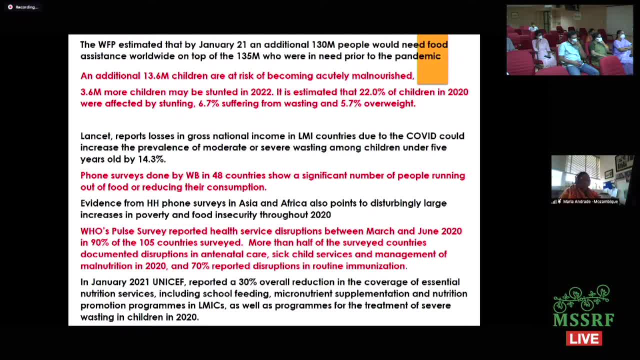 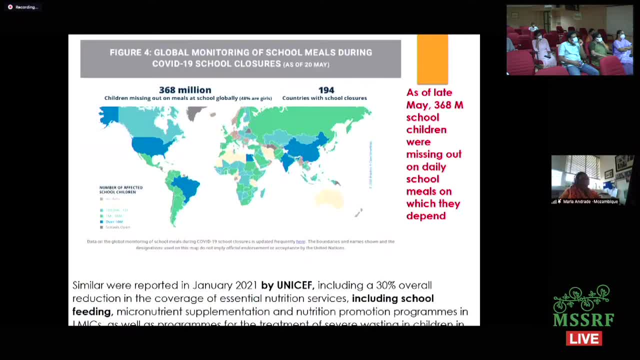 But what is quite interesting is the close of the school feeding program. Next, please, If you see, for example, on the school program in 194 countries they assisted 368 million children, But as of late May the school was closed. 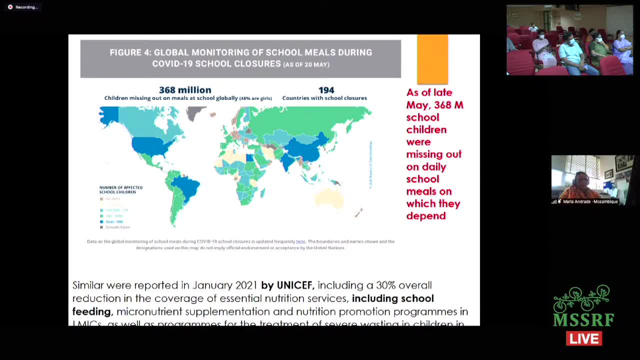 and a lot of these children who depend on this meal could not do that, And the same thing is also reported by UNICEF. And this is a problem, because if you want to develop nutritious people from the beginning, there is a problem. Next, please, 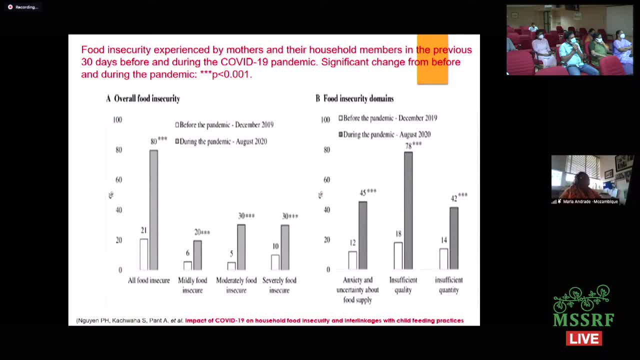 The same thing goes for children, The same thing goes with food insecurity for mothers and household members. in the previous 30 days before and during COVID-19.. There is a significant change from before and during the pandemic. If you see, before the pandemic there was food insecurity. 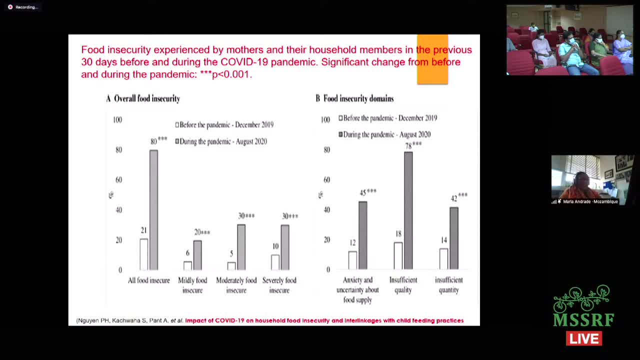 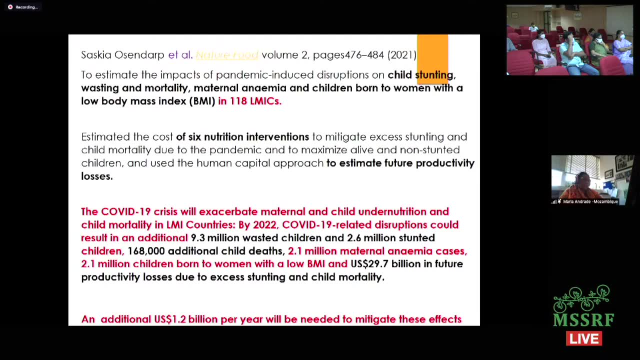 but it was much less than after the pandemic. Next, please. So a very interesting article that was written by Saskia. She's the executive director from the micronutrient forum and is published in Nature Food, The study that they conducted. they estimate the impact of pandemic. 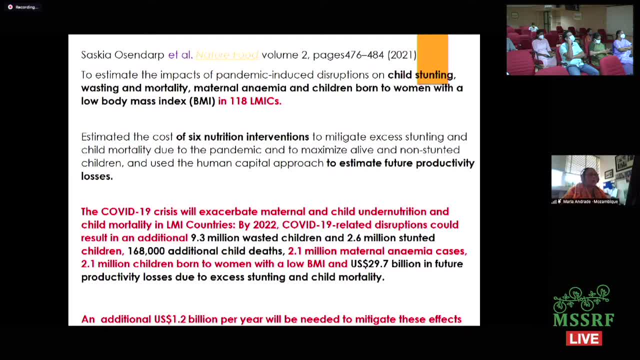 induced re-disruption on children, On child stunting, wasting and mortality. maternal anemia in children born to women with low body mass in 118 low to middle income countries And they estimate, for example, sick nutrition intervention to mitigate the excess of stunting and child mortality due to pandemic. 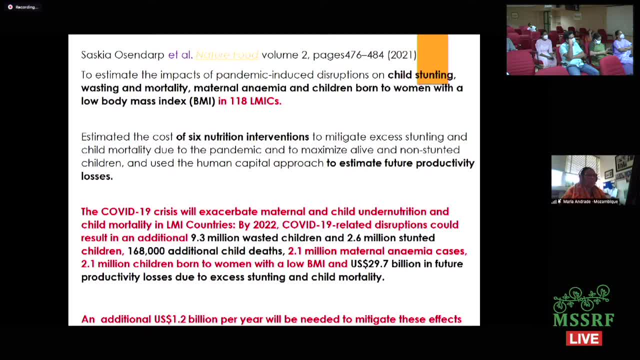 And, what is very interesting, they look into how they could estimate the future for productivity loss. The results show that the COVID-19 crisis exacerbate maternal and child- and the nourishment and child- mortality in this country, And that by 2022, COVID-19-related disruption could result in an additional 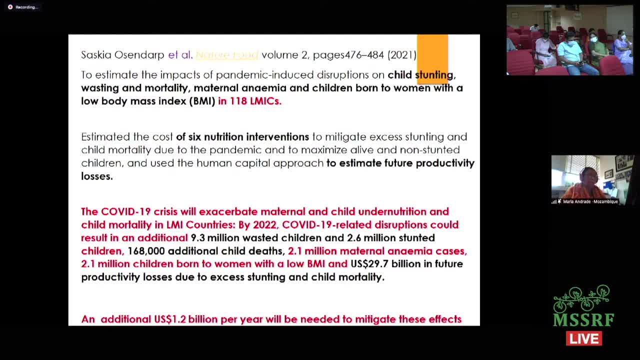 9.3 million wasted children and 2.6 million stunted children and 106 million children. That's 168,000 additional child deaths, The 2.1 million maternal anemia cases, 2.1 million children born to women. 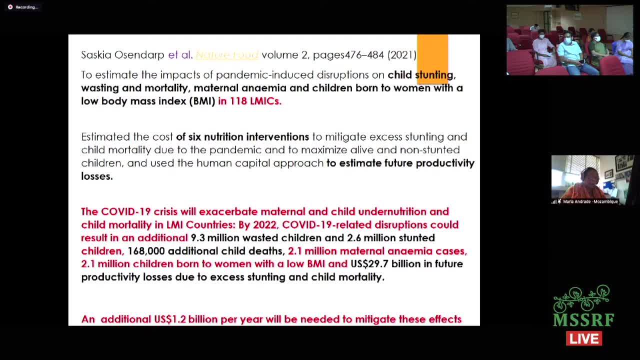 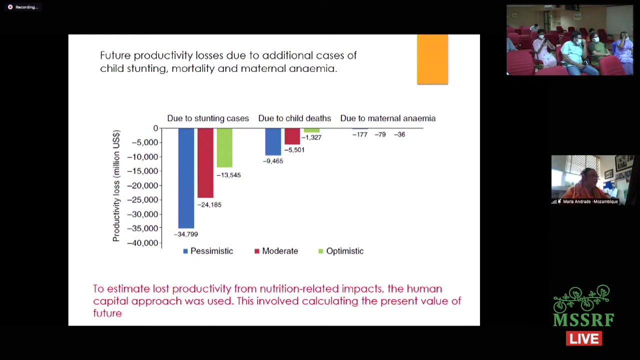 with low and 29.7 billion in the future, productivity will be lost due to the stunting and child mortality. These are not very good. Next, please. So, Maria, if you could focus on- you know- the suggestions. I think that's what we alluded to. 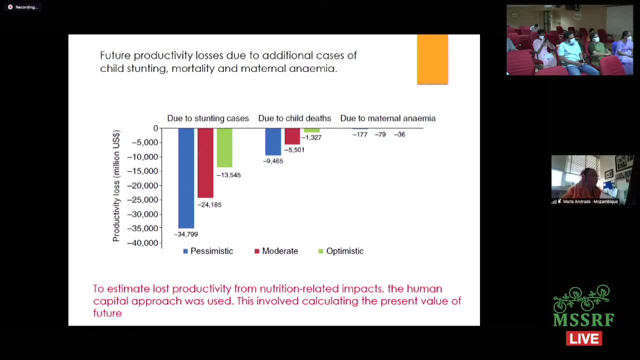 Yes, I'm almost there. I'm almost there. The future productivity. if you see, this is what I mentioned. they have three. they model it with pessimistic moderating and all this and they find out the loss in US dollar due to stunting child death. 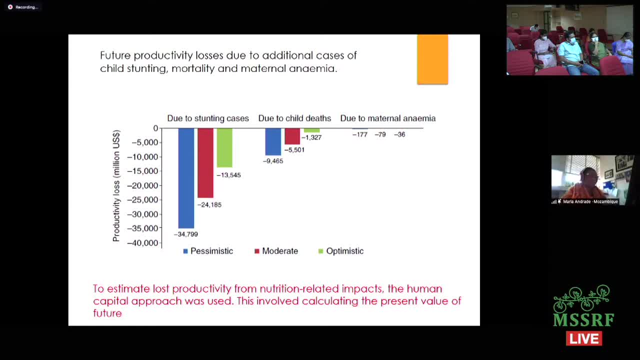 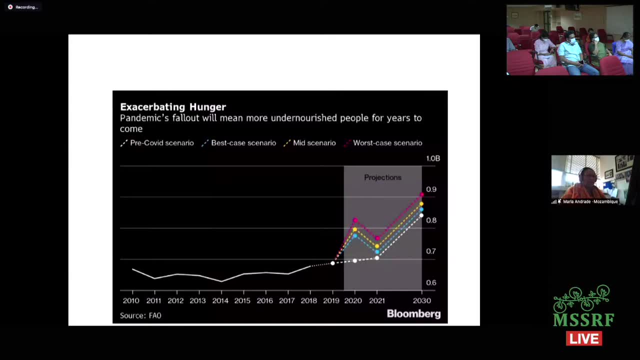 and to maternal anemia. Next, please, Next, please, The same thing. with this graph, The situation is not very well. This thing can project very in a very until 2030, if we don't take immediate action. 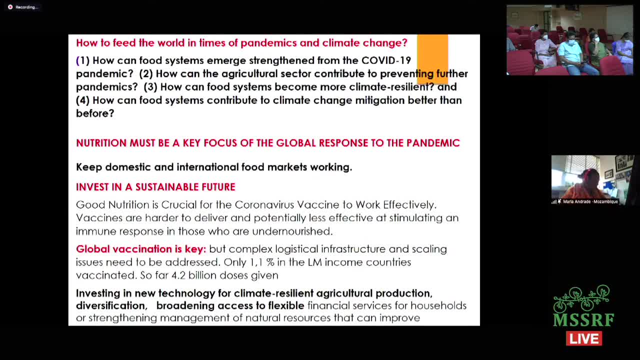 Next, please, Next, please, Thank you. Next, please, Next, please, Next, please Next. Ms IrASC's presentation: Next, please, Next, please, Next, please, All right, Next please. 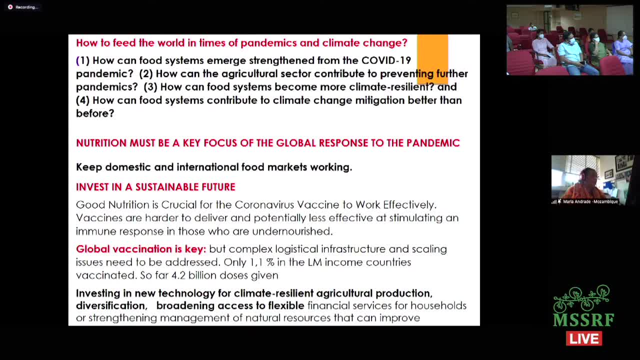 Next, please, Please, response to pandemic. We need to keep domestic and international food market working. We need to invest in a sustainable future, sustainable agriculture, looking into biodiversity, looking into other species that has not been explored And also, as we know, good nutrition is crucial. 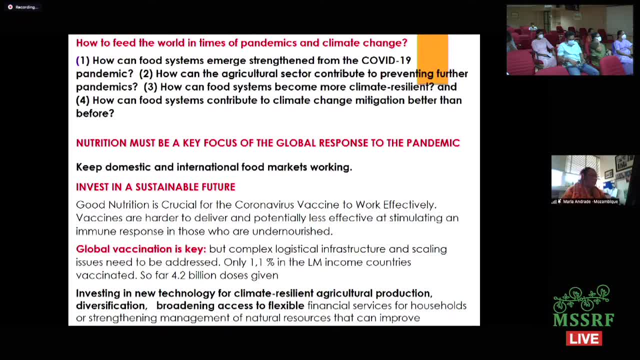 for coronavirus vaccine to work effectively. As you know, vaccine at the moment are harder to deliver and you need to have a good nutrition for very good immune response. And Diya was saying only 1.1% of the population in low and middle income countries were vaccinated. 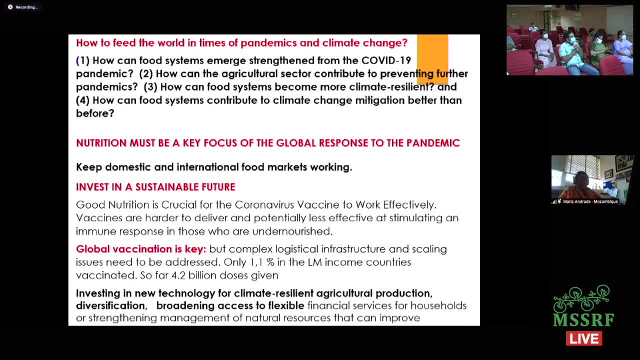 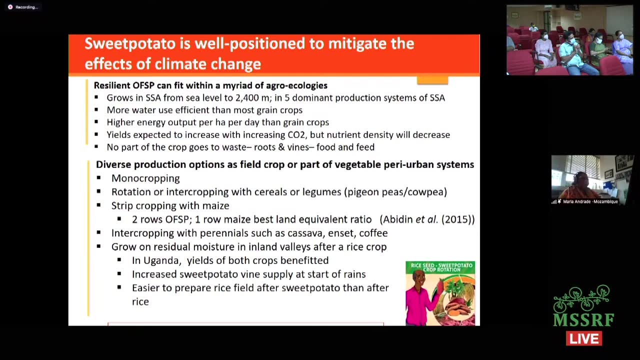 And again investing in new technology for the future, Thank you. We need to invest in the future and I think that's the key to making our country more resilient. Agriculture production diversification. financial service is the clue Next, please. So again, I work in bio-fortification. IC Sweet Potato is well positioned to mitigate the effect. 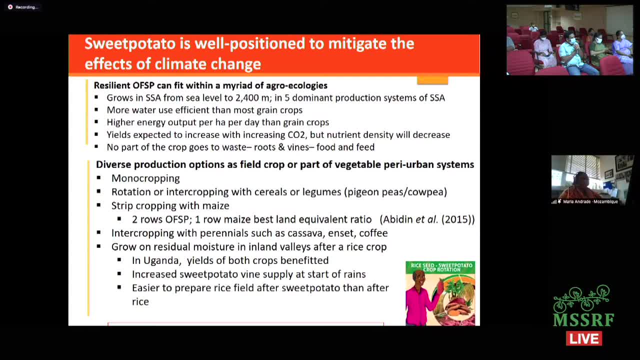 of climate change, all the characteristics of their agronomy, And also there was a time where I was in the country and I was in the US, and in the US, and in the US, and in the UK, and in the US and in the US. So we need to invest in the future, We need to invest in the future And again investing in the future. We need to invest in the future, We need to invest in the future And again investing in the future, And again. 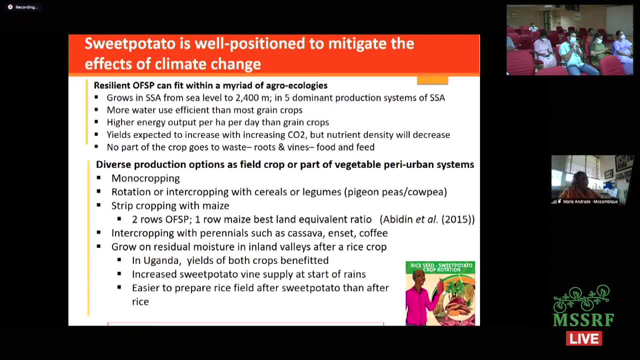 I was calculating, to produce one kilogram of beef how much water you need and this water how much sweet potato you produce. I found out for one kilograms of meat you could produce 200, 300 kilograms of sweet potato. So we need to probably go veggie. 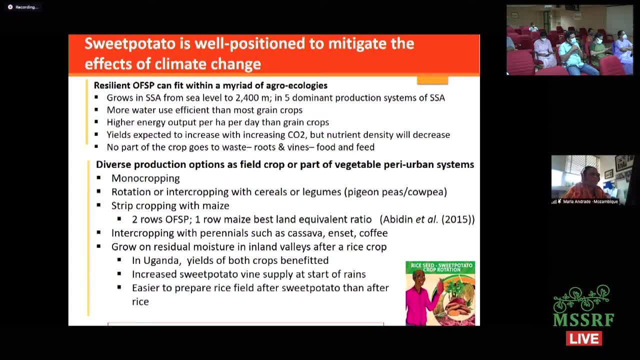 and try to maximize what you have to be able to use food to feed the growing population. Looking at those other aspects, intercropping rotation with maize, with pulse, with cassava- it all applies for sweet potato Next, please. 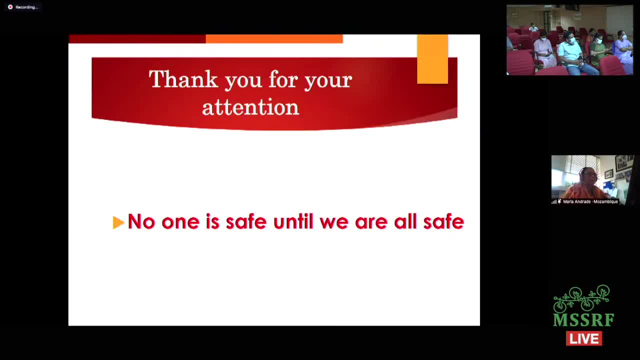 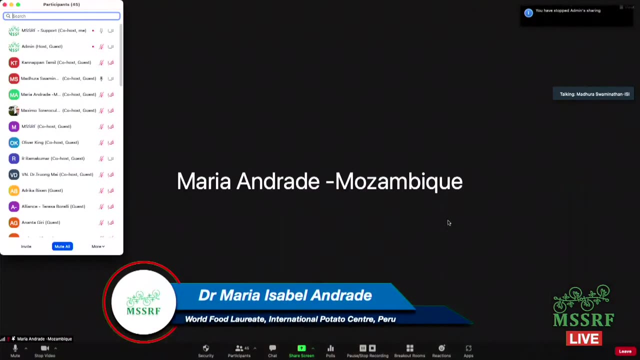 Next, please, The product development and diversification. Thank you for your attention And I think no one is safe until we are all safe. Thank you so much for your attention. Thank you very much, Maria Andrade. We listened a lot this morning in earlier sessions. 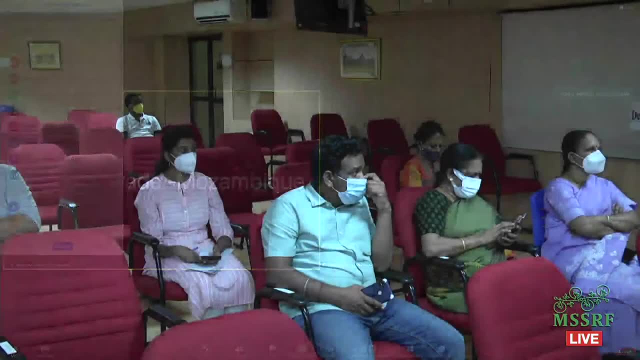 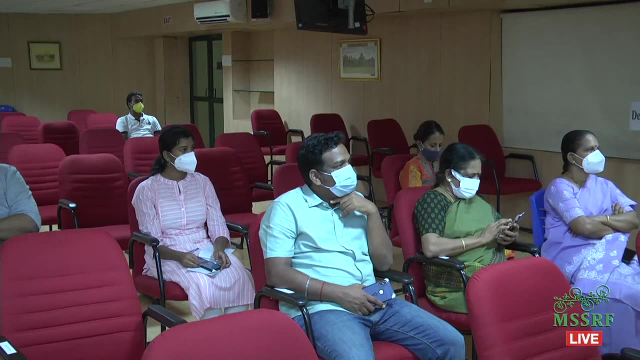 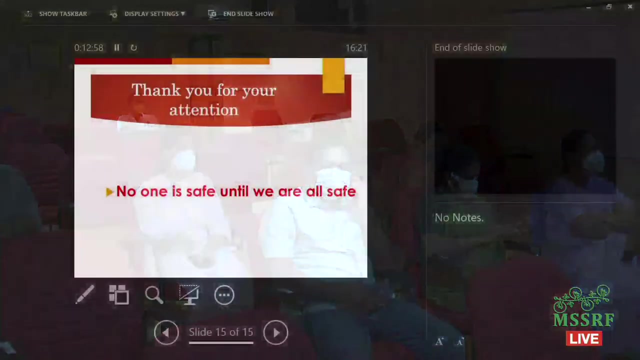 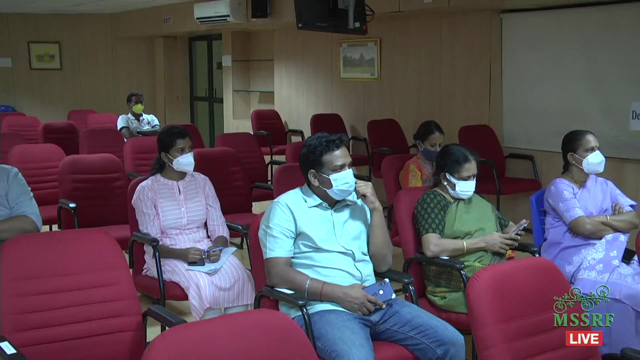 to animal protein, and so she has brought back the importance of vegetable. I mean either sweet potato and bio-fortified crops such as sweet potato. The last speaker for this session is Professor Ramkumar from the Tata Institute of Social Sciences, Mumbai, who, being an old student, 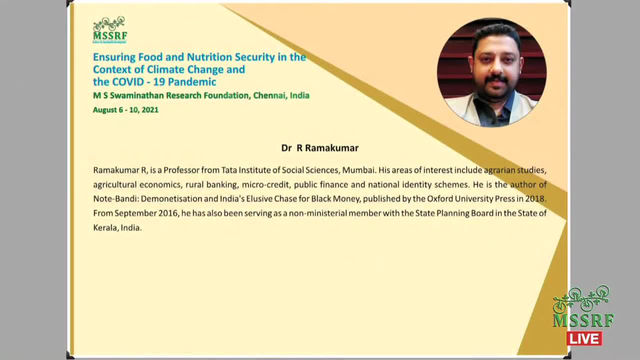 I don't know how to introduce him here, but he is somebody who is not only an academic researcher but very engaged in policy discussions on a range of subjects in India, starting from, you know, labor issues to questions of public policy, food security. 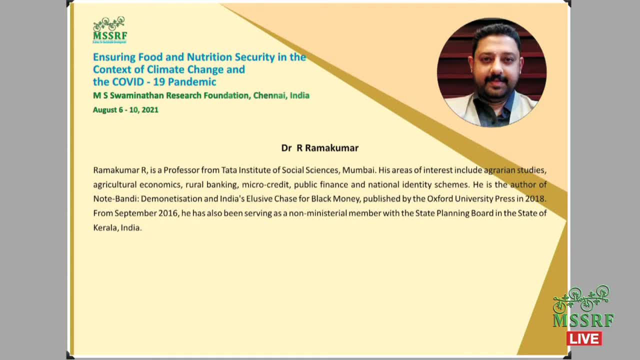 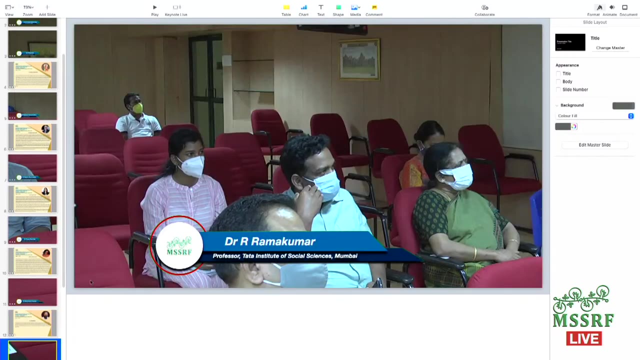 very recently vaccination policy and has been for the last five years a member of the Kerala State Planning Board. So, Ramkumar, I hope you're going to give us a flavor of the specific problems in India and what can be done to address them. 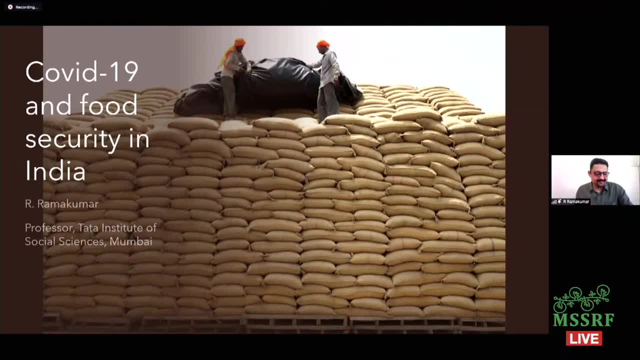 Over to you, remember? I will get you on the time. yeah, Yeah, Thank you. Thank you, Professor, Professor Madura, and thank you to MSSRF for having invited me to this panel. I shall speak over the next 15 minutes. 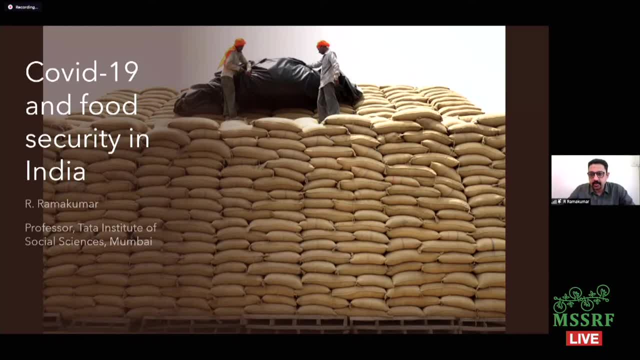 on the topic COVID-19 and food security in India, And in doing so I'm going to keep things very brief. I'm going to summarize the major points that have come up in this debate and not get deeper into issues, so pardon me for that. 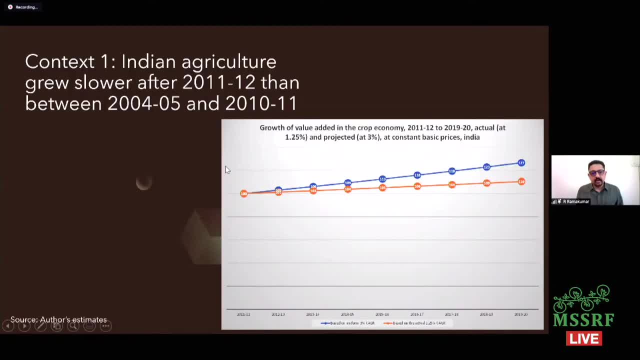 Basically, I shall begin with two important contexts vis-a-vis agriculture and COVID-19.. Indian agriculture. the first context is the following: Indian agriculture has been growing slowly for a very long time now. for over a decade now, the growth rate of Indian agriculture has been lower. 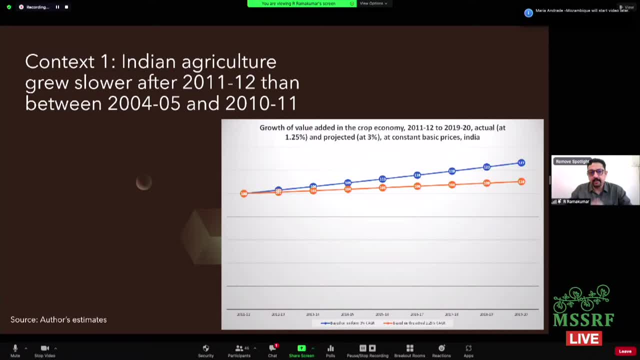 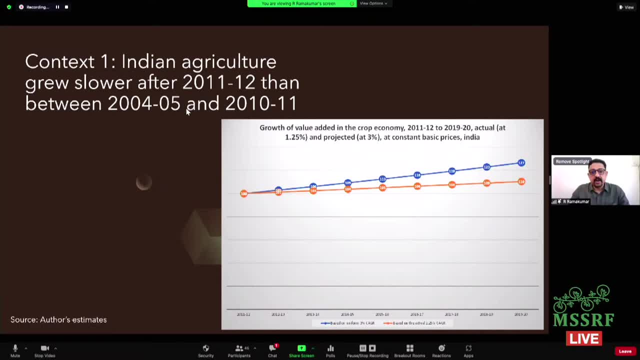 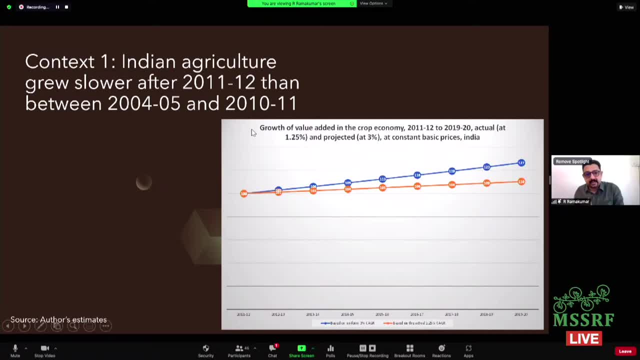 at the same 3% rate in the 2010s as well, then you would be where the blue dot ends in the graph. But because you grew only on an average by about 1.25% per annum, you are there at the orange point at the end of it. 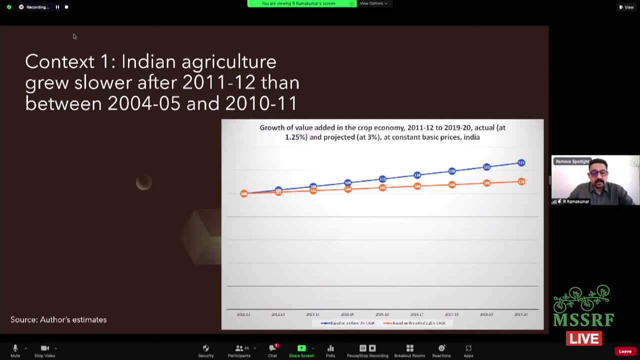 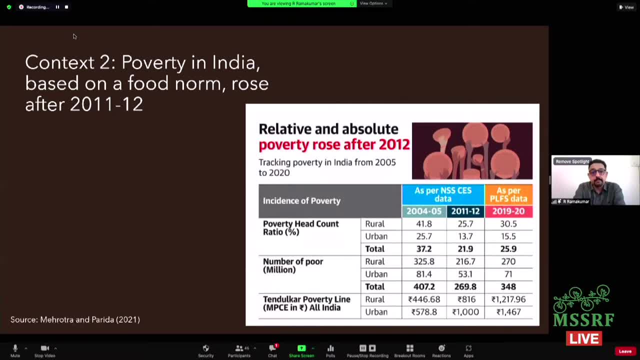 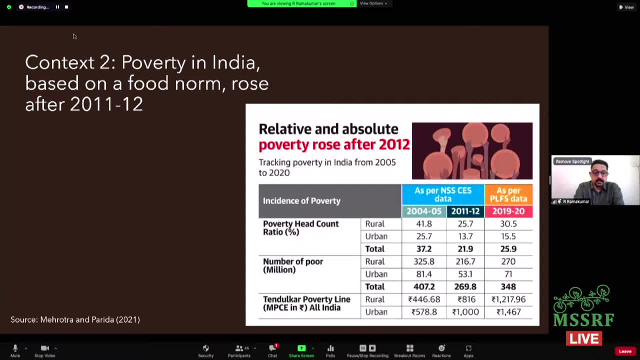 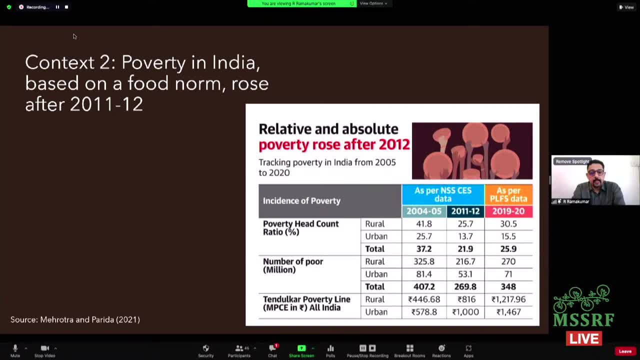 So your growth rate has been very poor compared to the previous decade. in India is measured using a food norm in India. To begin with, it's important to understand that the poverty line that is used in India is very controversial. It is supposed to be not a poverty line but a destitution line, as Professor Madhura calls it sometimes. 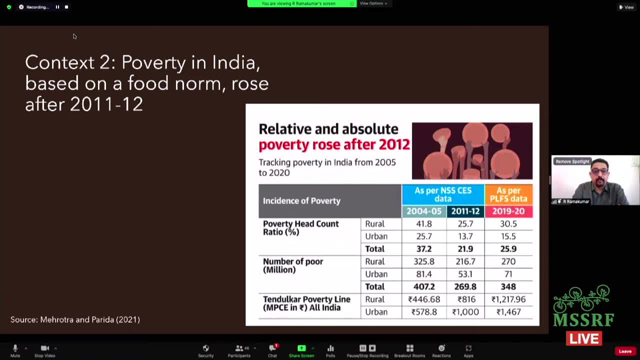 And you see that even when we use a very low poverty line of that sort, you will see that between 2011-12 and 2019-20, rural poverty rose by about 5 percentage points. From about 25.7 to about 30.5 percent is the increase that you see in this period. 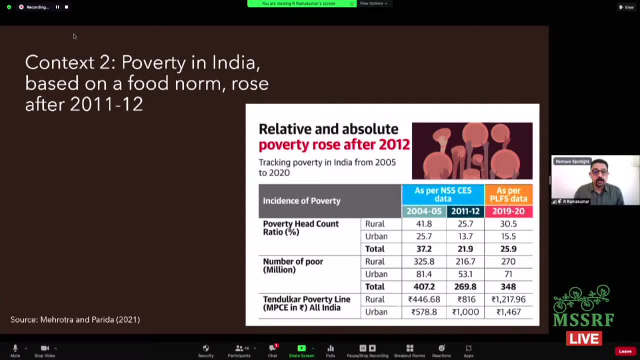 That's actually a rise of the number of poor in rural areas from something like 216 million to 270 million. So that's another context in which we are entering this discussion. All this is prior to COVID, and COVID hit on top of this. 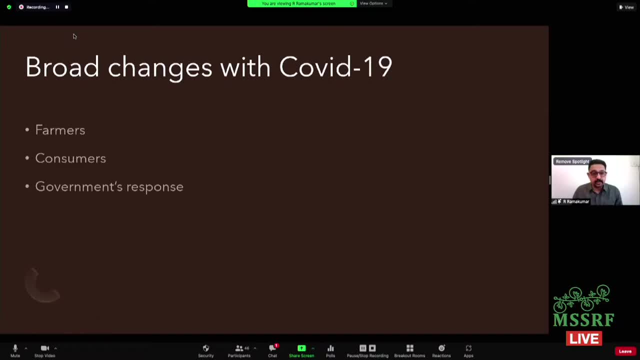 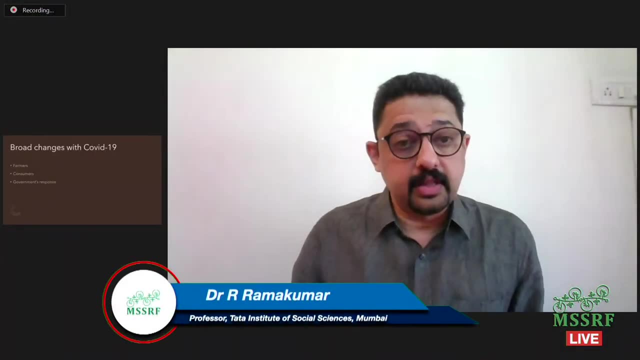 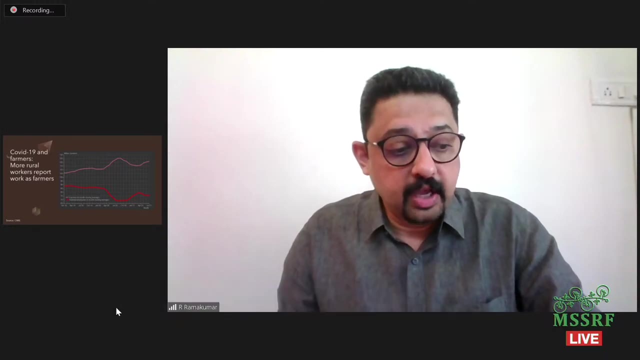 So in this remaining part of the presentation, I shall focus on three broad themes: How did it affect the farmers, How did it affect food consumption, that is, consumers, And how did the government respond to this problem? To begin with, if you consider the question of COVID and farmers, 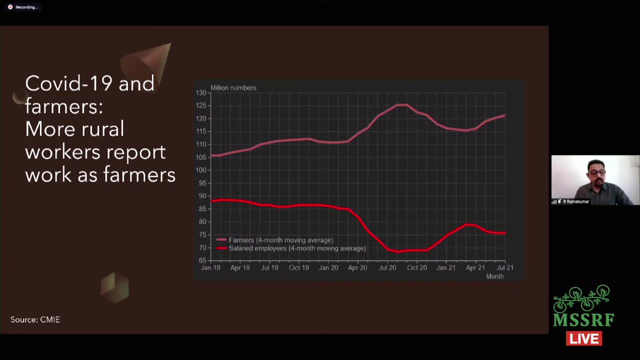 one important point that comes out from one of the surveys which is conducted by the Centre for Monitoring the Indian Economy, which has monthly data on employment, is that more people are farming after the pandemic began. If you look at this graph, which shows what is happening to the number of salaried employees in million numbers, 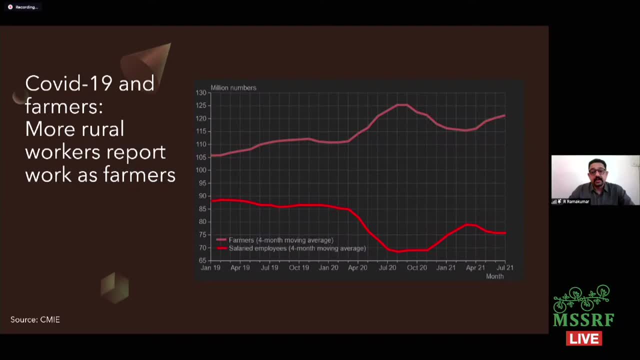 and what is happening to those who engage in farming. you will see that there is a very inverse relationship. after the pandemic began and as the pandemic proceeds, The number of farmers are actually rising. More people are cultivating, and that's primarily because there are no jobs in the urban areas. 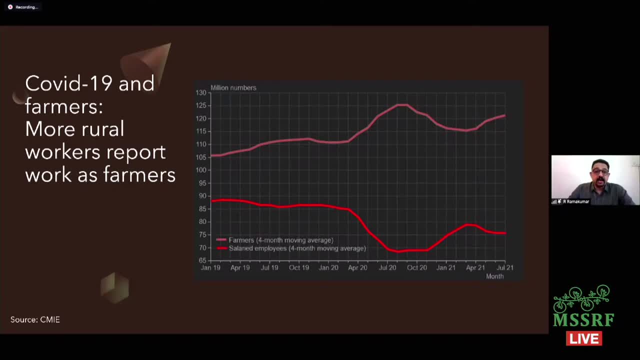 A lot of migrant workers have returned to rural areas and are cultivating the small plots of land that their families may have, and primarily to ensure some amount of food security over this period of the pandemic and the lockdown. So what is happening, however, to this enterprise? 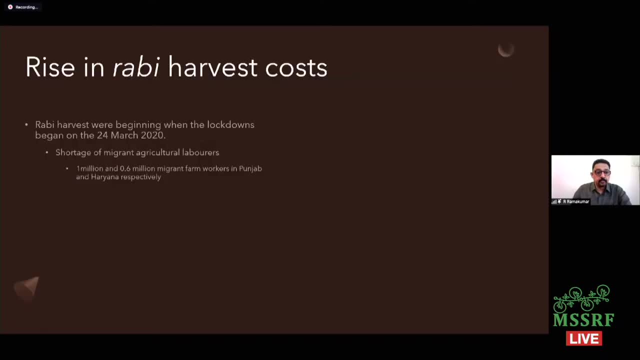 into which more people have entered into after the pandemic. The first point to note here is that when the pandemic began after the March month of 2020, the lockdown was very severe and labour mobility was severely affected. farmers faced a severe shortage of migrant agricultural labourers. 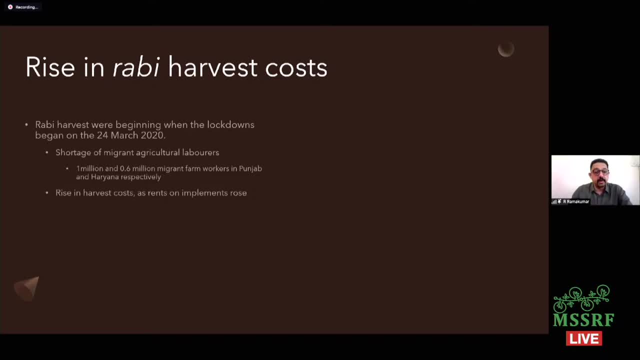 particularly in the agriculturally prosperous regions of Punjab, Haryana and so on. There was a rise in harvest costs. there was postponement of wheat harvest as a result. there was some amount of staggering of wheat procurement in that period which affected the farmers adversely. 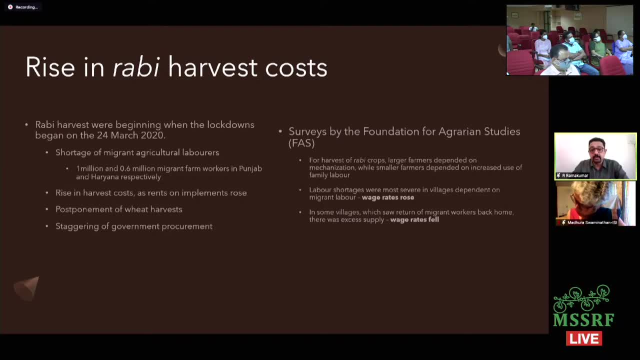 and other surveys which are conducted, for example, by the Foundation for Agrarian Studies or the Azim Premji University in Bengaluru. both in Bengaluru show that large numbers of farmers were unable to harvest, Many farmers even when they harvested. 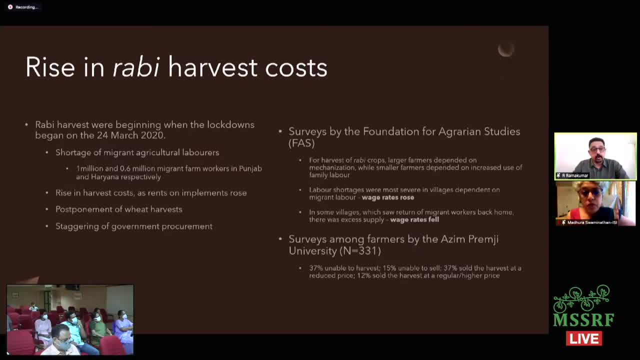 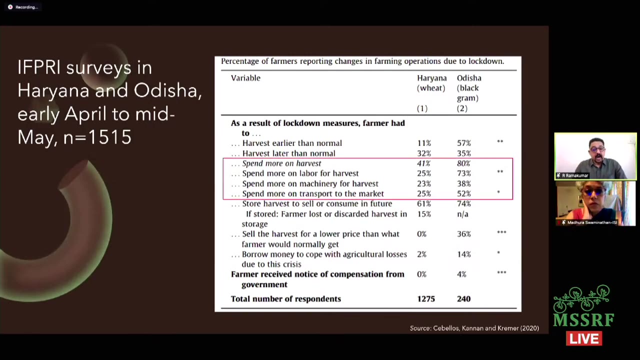 had higher costs to incur in harvesting because of higher wage sometimes or higher rents for agricultural implements sometimes, and so on. So this was something that most studies have noted: costs of harvesting severely going up and affecting profitability of cultivation. Other surveys, for example: 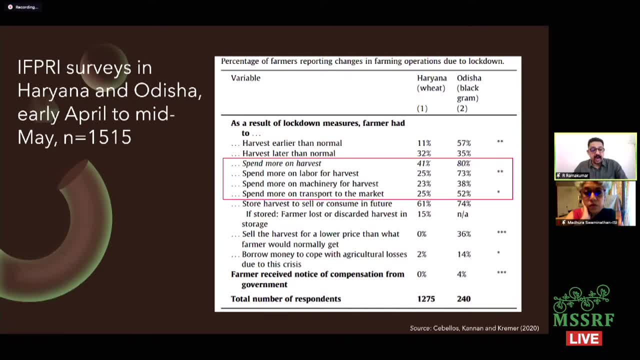 this survey by IFPRI in Odisha and Haryana actually also shows that farmers ended up spending more on harvest, more labor, more spending on wages for harvest, more on machinery for harvest, more on transport to take the commodities to the market, and so on. 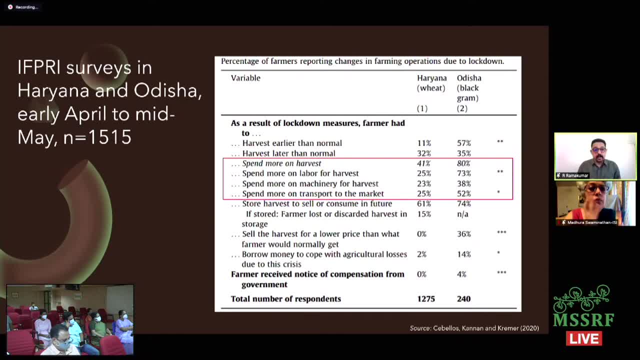 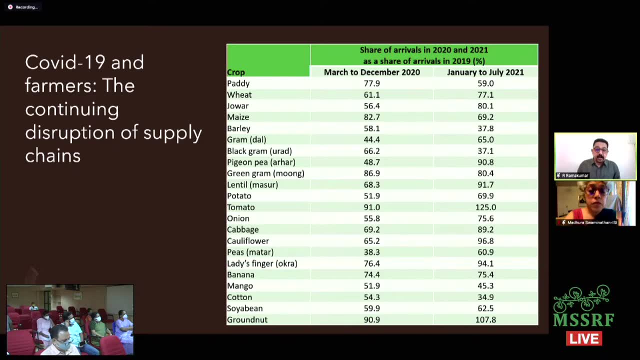 So clearly, costs of handling the produce and costs of harvest went up. This has adversely affected profitability. An attendant important adverse impact of the lockdown was the very major disruption of supply chains that happened during this time. I think this table is very important. 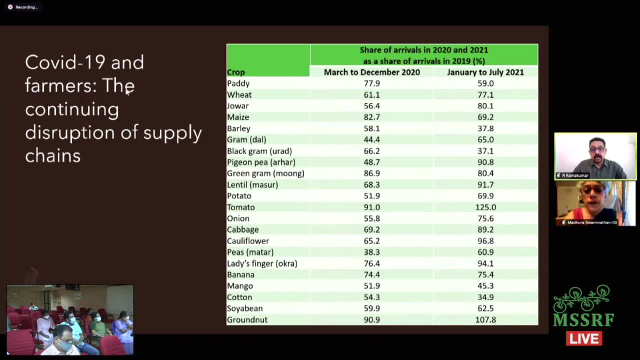 and this basically shows how much commodities arrived in the Indian markets during the pandemic. This first row here, March to December of 2020, the numbers here are percentages of percentage of arrivals in March-December 2020 as compared to March-December 2019.. 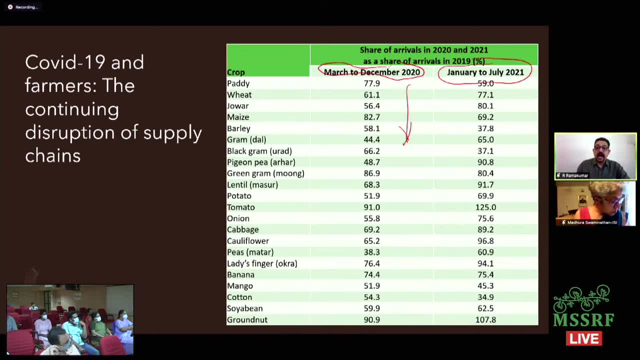 And here January to July of 2021, means as compared to January to July of 2019.. So 2019 is the baseline here. If you see in most of the commodities except one and two, you will see that the arrivals 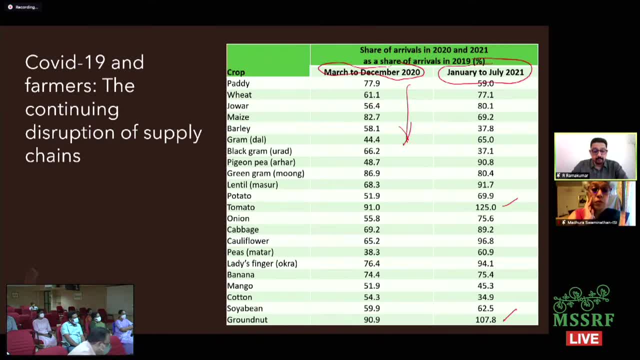 even during January to July of 2021, that is, after many months had passed and since the lockdown had been lifted. supply chains remain disrupted In many crops, like paddy, for example, only 59% of the commodities have arrived in the market in 2021. 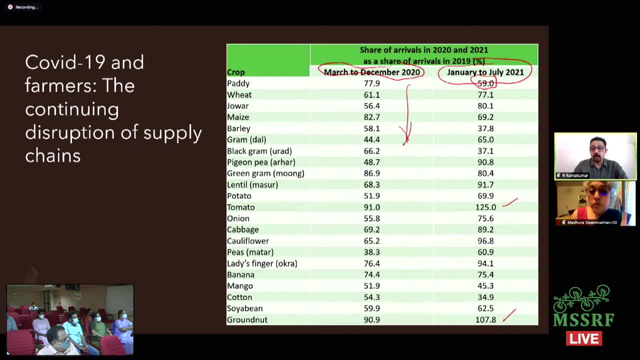 as compared to 2019.. In many other crops- in wheat it is 77.1%, and in most other commodities, you will see that the percentage of arrivals have been lower than the baseline that we have chosen for 2019.. So supply chain disruptions continue. 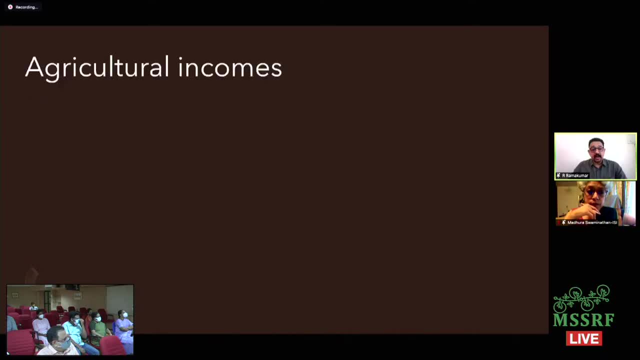 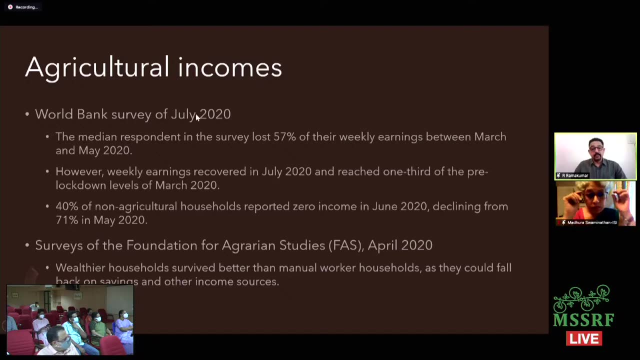 even after 2020 has passed And this has affected agricultural incomes in different ways. The World Bank survey of 2020 in July shows that the median respondent in their surveys had lost 57% of their weekly earnings between March and May, And 40% of the non-agricultural households. 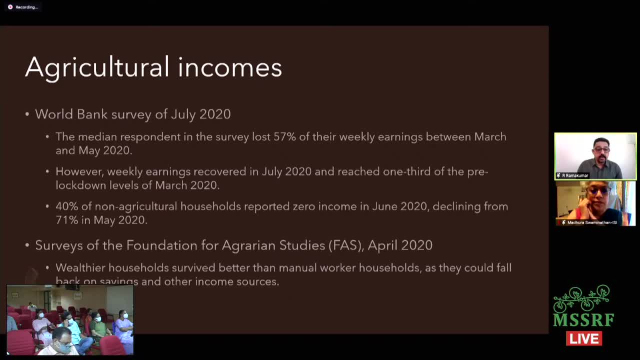 reported zero income in June 2020, which was actually a decline from 71, but nevertheless was a substantial number. Foundation for Agrarian Studies' surveys in April 2020 show this has affected rural households differently: Wealthier households have survived, while poorer manual work households. 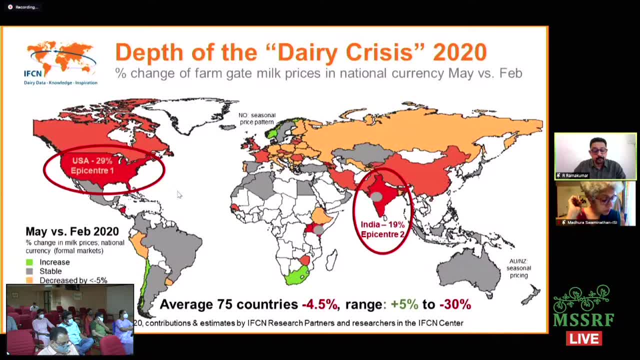 could not fall back adequately on savings and other income sources. Milk was very important in the sense because India and the United States are called as the two epicenters in terms of the crash of milk prices in 2020.. These are the only two regions in the world. 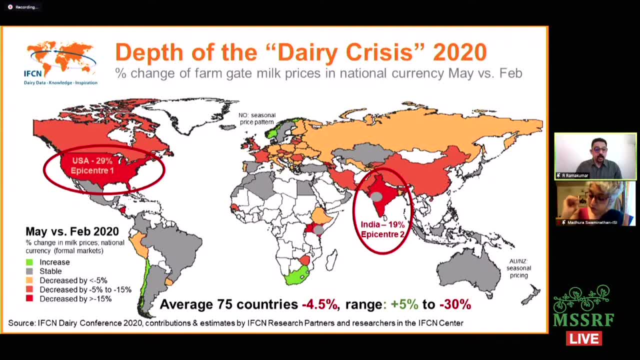 where there was such significant fall in prices of milk. In USA it fell by 29%. In India it fell by 19%. That's substantial because milk per liter was 35 per liter in many regions And by the time the pandemic crossed two months. 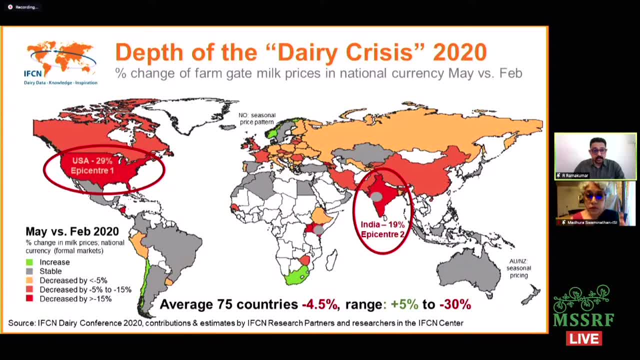 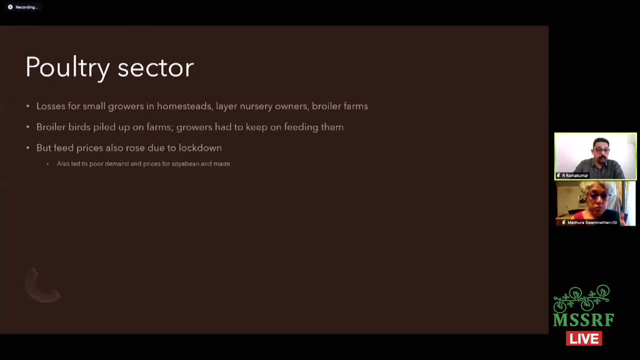 the price had fallen to something like 17 to 20 rupees per liter. Same with respect to poultry growers. The losses have been substantial for all kinds of poultry growers. Broiler birds piled up on farms. Farmers had to keep on feeding them. 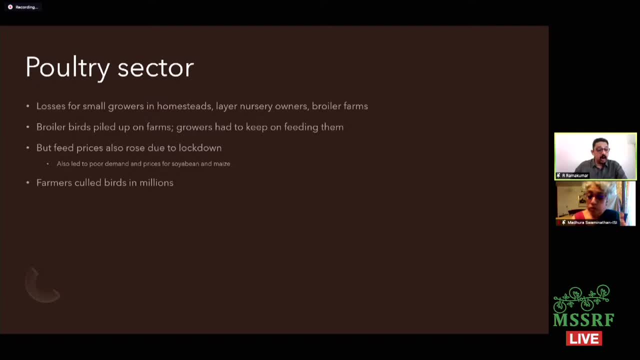 And because they couldn't keep on feeding them. they culled the birds in millions And the losses have been substantial, because not just of this culling, because eggs also started to pile up in the farms, Chicken prices falling from 85 rupees per kg. 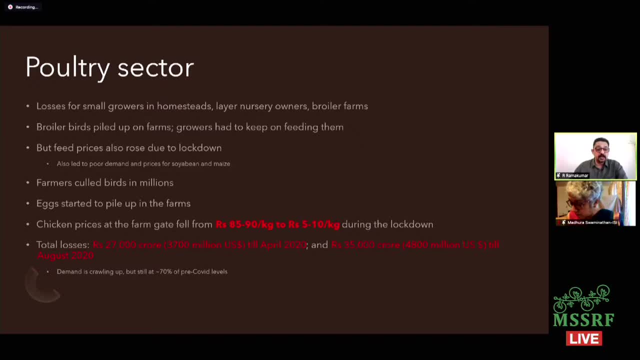 to 5 to 10 rupees per kg, And the total losses for this sector have been estimated to something like 27,000 crore for the two months of the pandemic. in 2020 itself, Demand is still 70% of the pre-COVID levels. 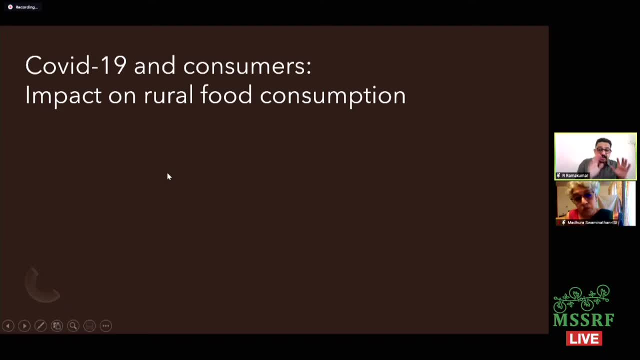 So this is something that the summary of what has happened on the farmer's side, What has happened on the consumption side. Here again, the impact has been adverse. The World Bank surveys of 2020- July show 47% of the households showed signs of food insecurity in May. 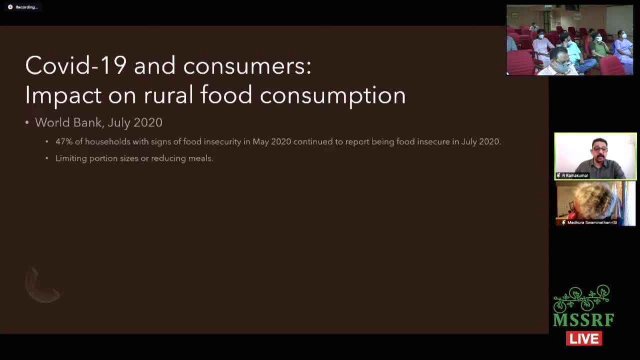 And many households were limiting the portion sizes or reducing the meals. The Foundation for Agrarian Studies surveys in April showed that household consumption fell. There was also a decline in the diversity of food that was consumed. And here again, as would be obvious, 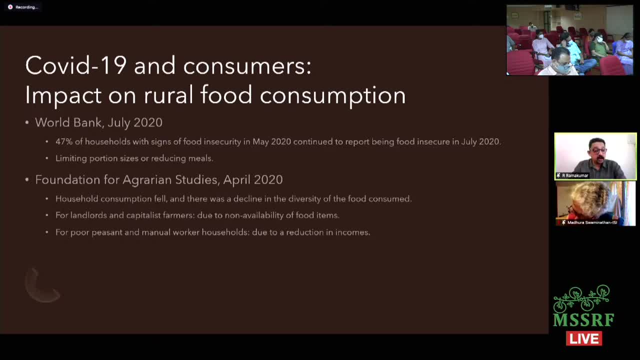 the impacts were different for landlords and large farmers on the one hand, and poor person and manual worker households on the other. Surveys by IFPRI in Haryana and Odisha and surveys by Azim Premji University in April-May 2020 also show very similar results. 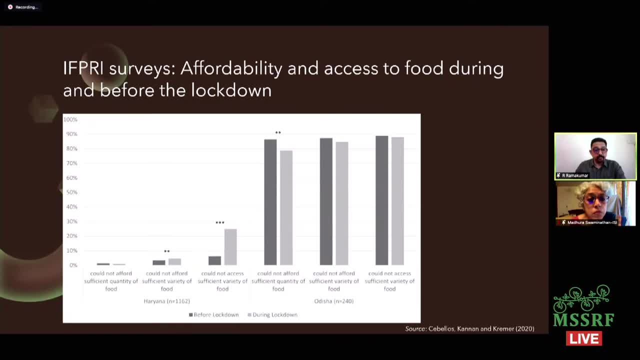 I shall quickly show one slide each from the IFPRI survey which shows the high numbers of households which could not afford sufficient quantity of food or could not afford sufficient variety of food or could not access sufficient variety of food. All these will show in Odisha and in Haryana. 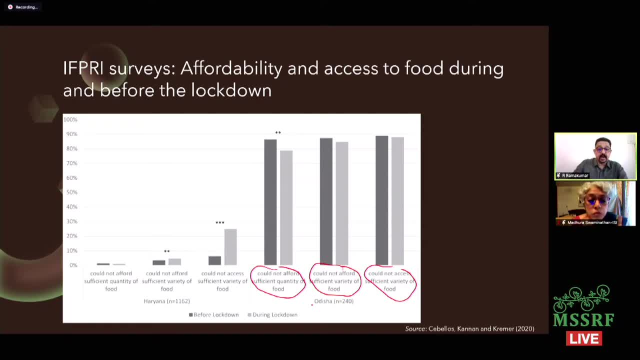 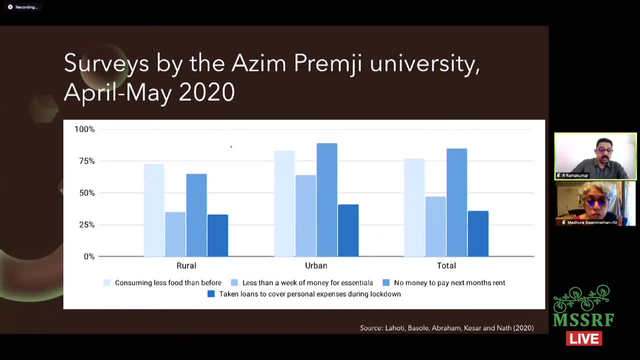 You will see, particularly in Odisha, more than Haryana, the impacts have been very high in terms of food consumption, Same with respect to the Azim Premji University surveys. This is the households consuming less food than before: Up to 75% of the households. 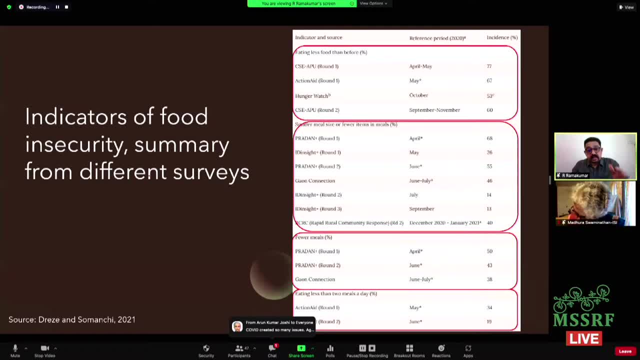 were consuming less than before. This is another summary. I borrowed this from John Grace's and Anmol Samanchi's review of the work. You will see more than 60-70% of the households in the different surveys that have been conducted in this time. 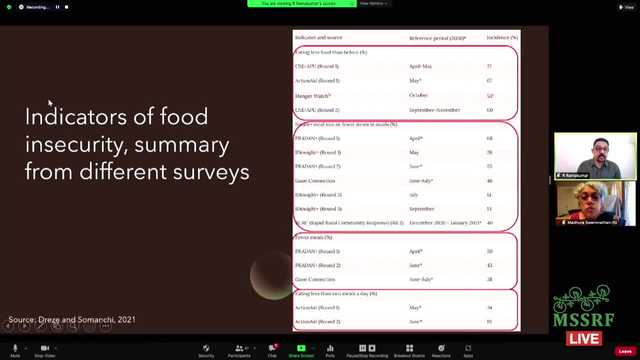 have been affected by different kinds of food insecurities. Either they did not have enough meals or they had a smaller meal size. In whatever survey you take, you will see that substantial numbers of the households have actually been affected by this kind of food insecurity. 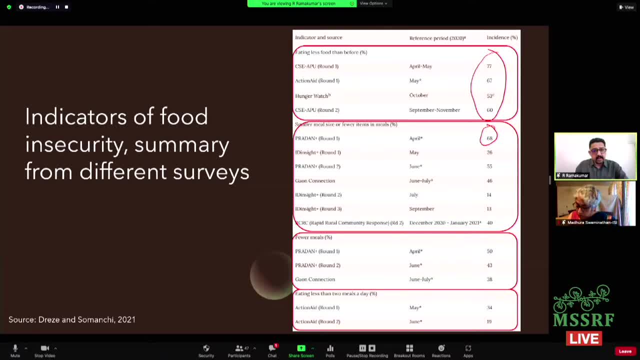 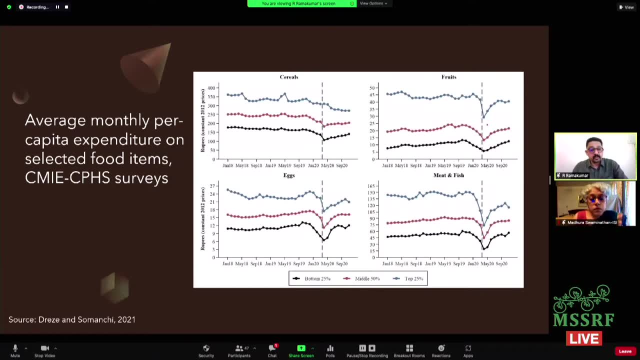 And that is consistent over many surveys that you see. This is the average monthly per capita expenditure on selected food items, as shown by the CMIE surveys. You will see, of course, the vertical line is the lockdown. when the lockdown began And you can see the sharp fall of food expenditures. 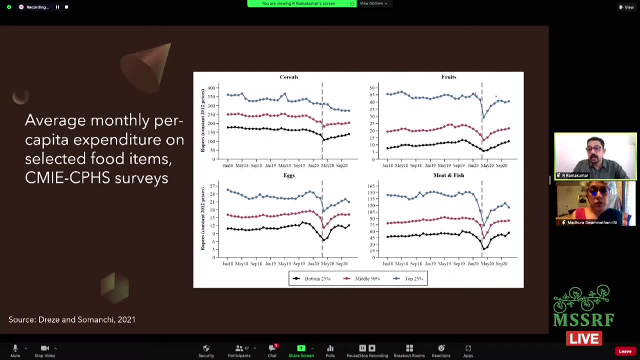 which still have not picked up. You will see, here, here, here, You will see, none of these have picked up to the pre-pandemic levels, even after many months passed, And more so, the decline was sharper for fruits, for eggs, for meat and fish. 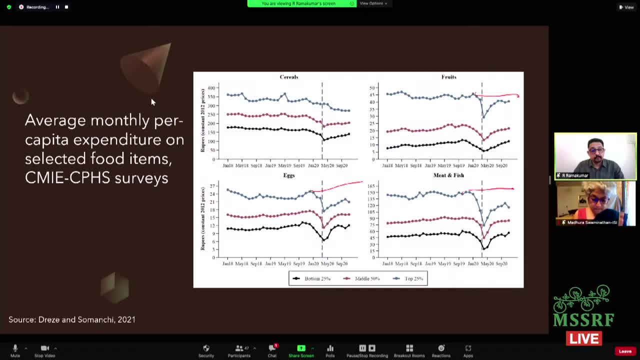 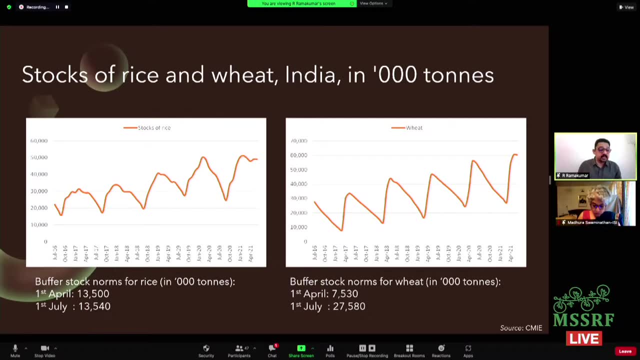 more so and less so for cereals, So this affected the nutrition also in different ways. Now this has happened. What is unfortunate is this has happened even when the government has very high record levels of stocks of rice and wheat in the godowns of the Food Corporation of India. 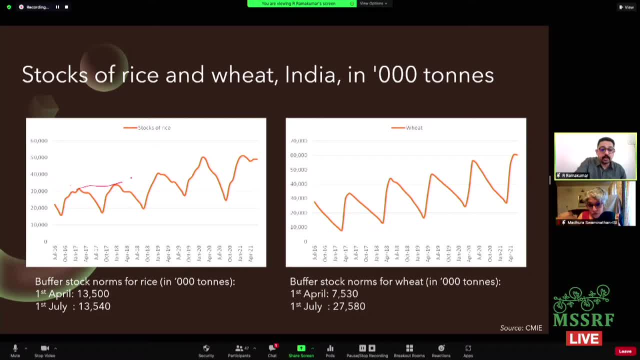 As you can see, the peaks of the stocks of rice and the peaks of the stocks of wheat have risen over the years from 2016 to 2021.. However, the hunger has persisted even as these stocks have risen over a period of time. 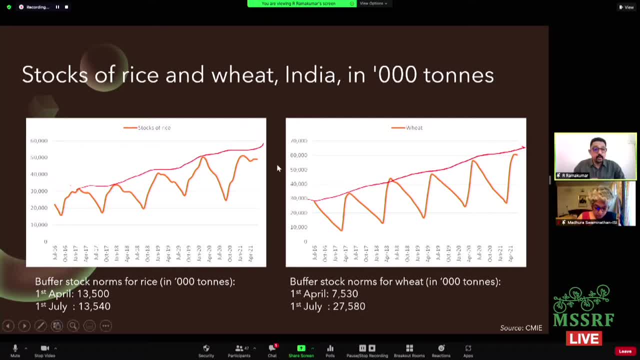 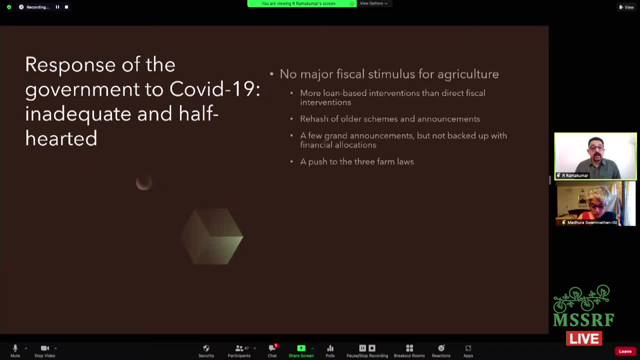 And that actually brings us to what the government did during this time. If you look at the response of the government to COVID-19 relief, we'll summarize it in the form as inadequate and half-hearted. The government did announce a stimulus package for the economy. 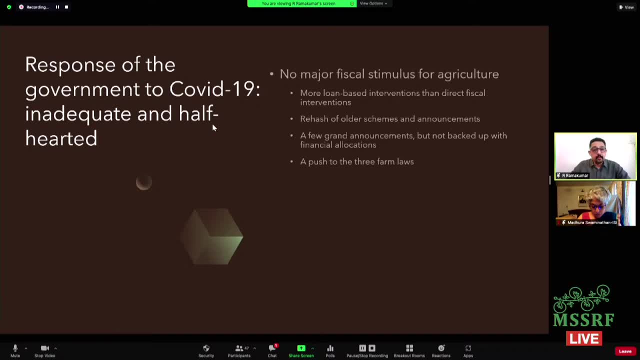 but there was absolutely nothing in it for agriculture. to be specific, The interventions were more loan-based interventions rather than direct fiscal interventions, and that has been the problem with the package as a whole. Most of the announcements were more a rehash of older schemes and announcements. 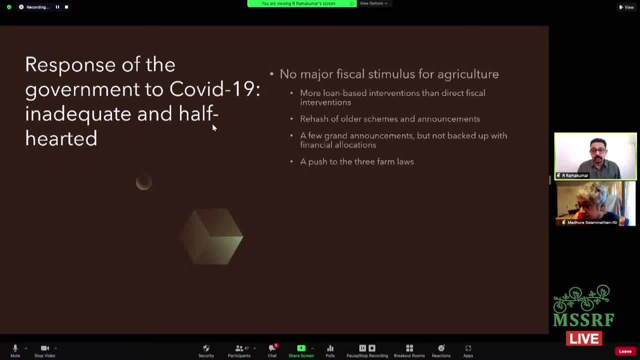 rather than anything new and innovative. The government also tried to help farmers during the lockdown. There were a few grand announcements, like spectacles, but they were not backed up with adequate financial allocations. And on the top of it, the government tried to give. 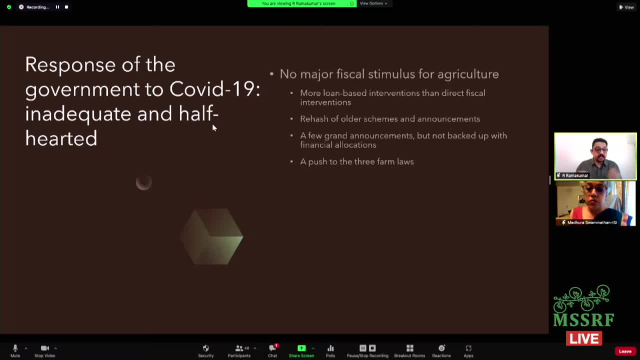 neoliberal reforms in marketing a push by passing the three farm laws, which has led to a large farmer's agitation and that is still continuing. The most important point- and I think this came as a relief for many- is that the presence of the PDS helped. 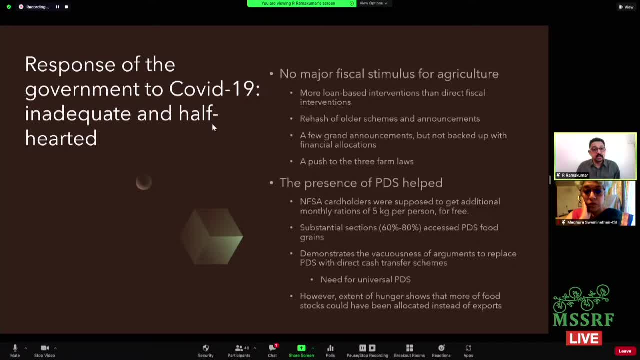 If the government had listened to many neoliberal economists in the past, India's PDS would have been wrapped up by now and converted into a direct cash transfer scheme. However, because of the agitations of large political parties, civil society organizations, etc. 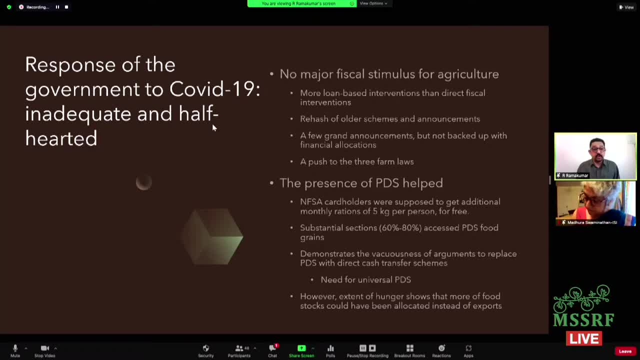 we have been able to protect the PDS from collapse and that has actually come in very handy. during the pandemic, Households were provided 5 kg of food grains free of cost during this time, with 1 kg of pulses, and surveys show that substantial sections 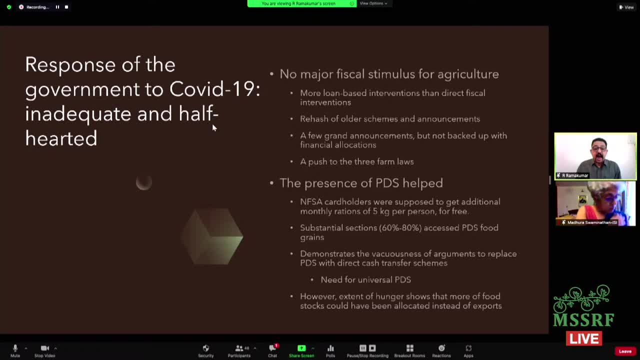 of the population, somewhere between 60 to 80 percent, accessed the PDS food grains And that is the only relief during the pandemic and that's because the PDS survived. It demonstrates the wackiness of arguments to replace the PDS with direct cash transfer schemes. 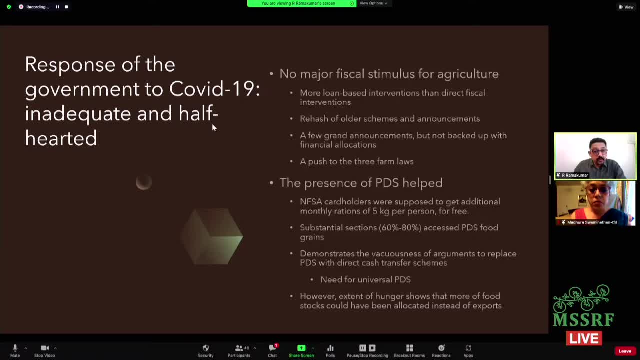 and this actually underlines the need for a more universal PDS in the country. However, the extent of hunger that has persisted even after this provision of 5 kg of grains free shows that government could have actually distributed a lot more food, grains and pulses. 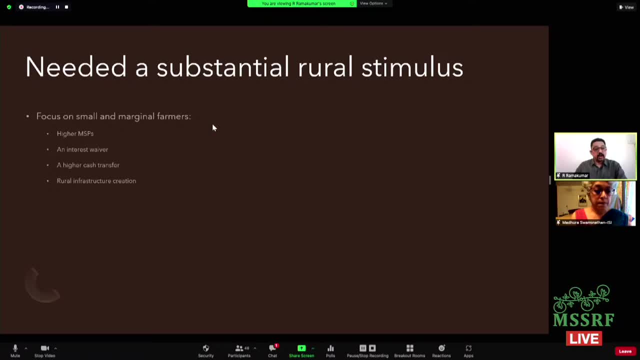 through the public distribution system. Now I'll come to the last slide. what is needed to be done, and I think what has been lacking over the last one year, is a large rural fiscal stimulus. I think the government needs to consider this on an urgent basis. 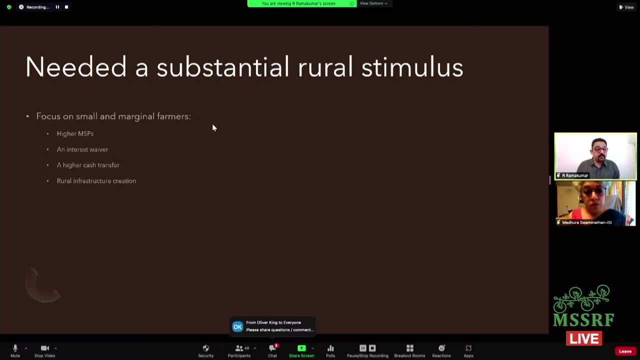 and the focus here, given the differentiated impacts that we have seen, has to be on small and marginal. We need a combination of higher minimum support prices to farmers, which has persistently not risen over the last few years by any substantial rate. We need an interest waiver. for the loans that farmers have taken. We need a higher cash transfer to farmers. We need an emphasis on rural infrastructure creation, including irrigation and so on, which will also contribute to rural employment. We need sectoral relief packages. This has been sorely lacking. 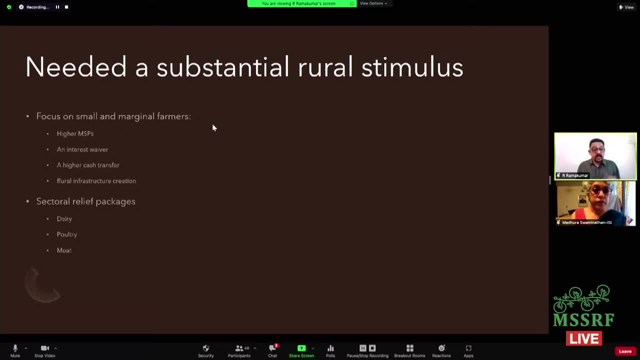 in every intervention of the government. These three sectors- dairy poultry and meat- have been very severely affected by the pandemic and the lockdown and the government has done almost nothing here. Very little has been done except the announcement of an animal infrastructure fund. 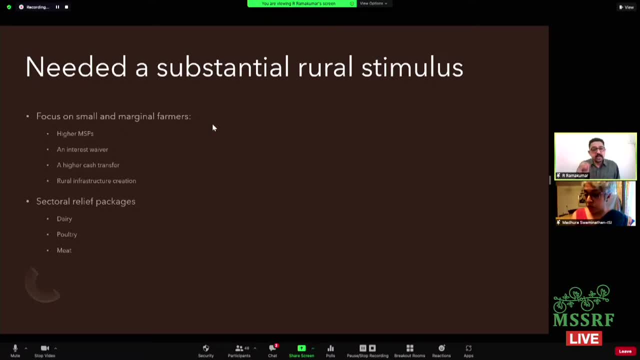 or something like that, but which is largely a loan-based scheme which is to be staggered over the next five years. We need higher investments in rural land, rural health, which is very poor in quality in rural India, And we also need something. 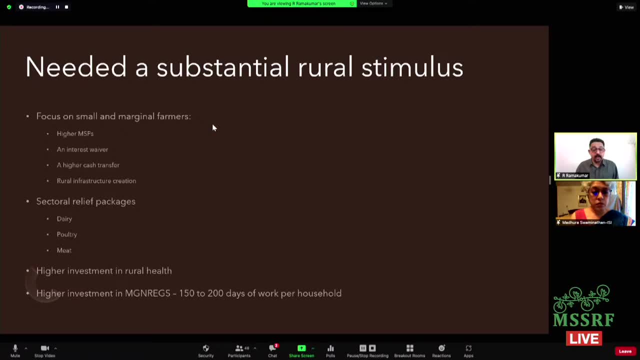 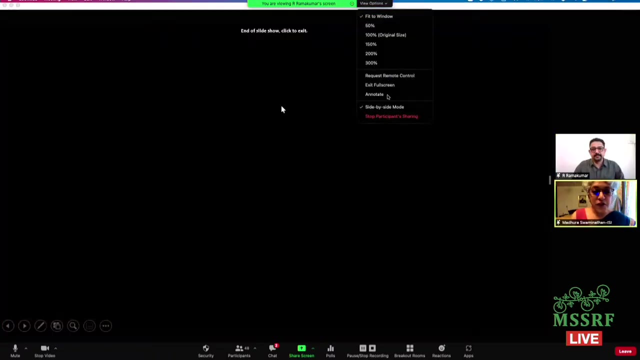 I have not discussed in the presentation: rural employment. We need a higher focus on the Mahatma Gandhi Rural Employment Guarantee Scheme, with 150 to 200 days of work assured per household in rural India. Thank you, Thank you, Dr Ramkumar. 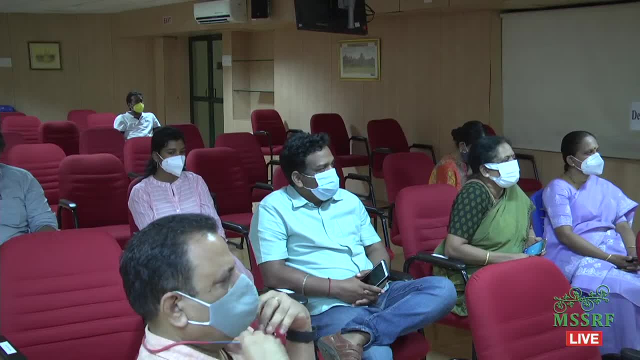 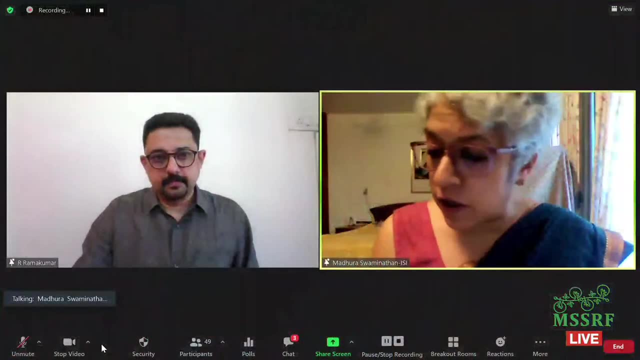 I think that, as we're going to the discussion, four speakers have complemented each other And you know, starting with Dr Torero. I think that setting the context- and I think Ramkumar has done that- for India. 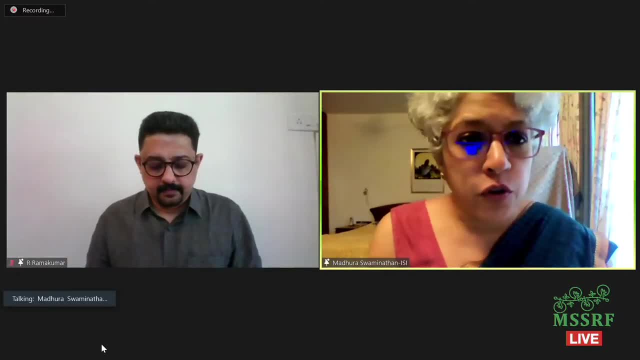 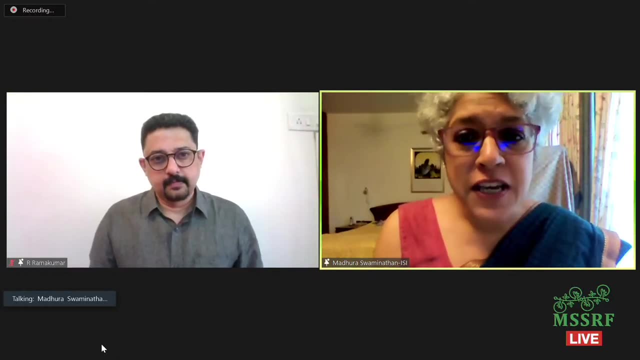 what was the trajectory of agricultural growth, of economic growth pre-pandemic and in many parts of the world The picture was not very rosy even before the pandemic, and the pandemic has really hit the economy And I think the point that it is not a short term. 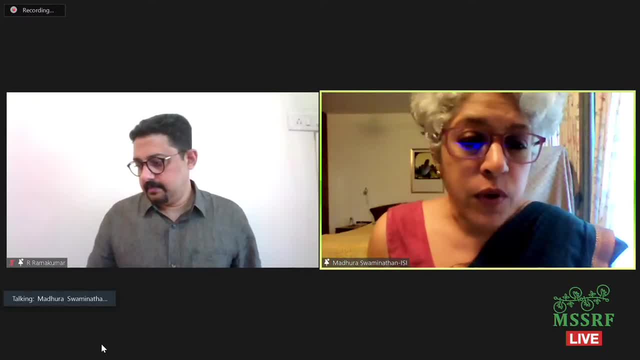 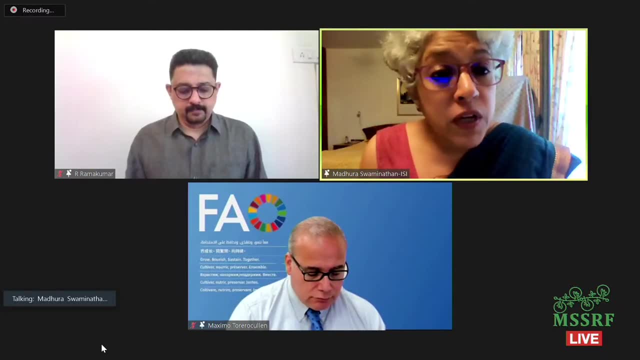 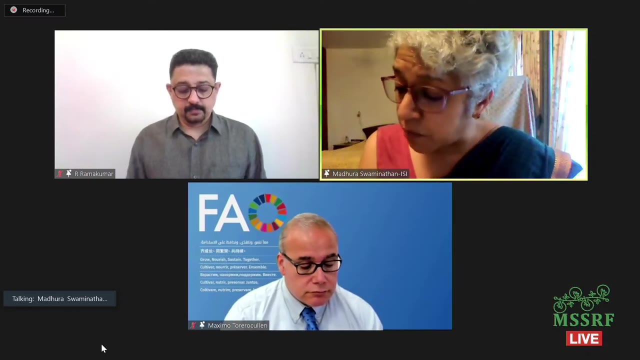 it's something that's going to remain for the next couple of years. So when we plan, the immediate response was relief measures of different kind, but we really need to start thinking about major investments, major changes in policy. The second point, I think, which has come out: 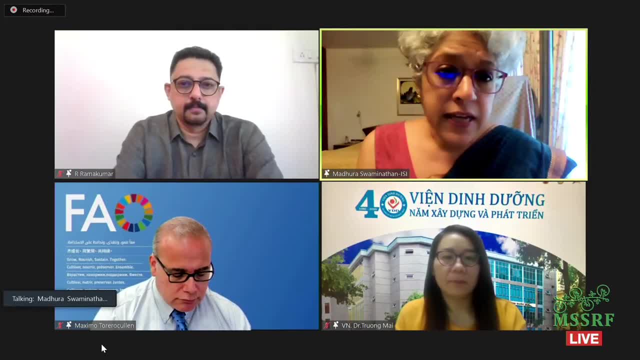 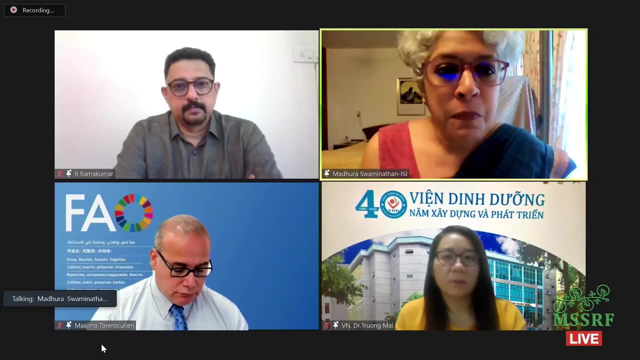 of all the presentations is that in some sense, you know, agriculture was resilient because the crops didn't start growing, you know, so we had, in terms of production, agriculture perhaps was the only sector where production continued during lockdowns and other restrictions. 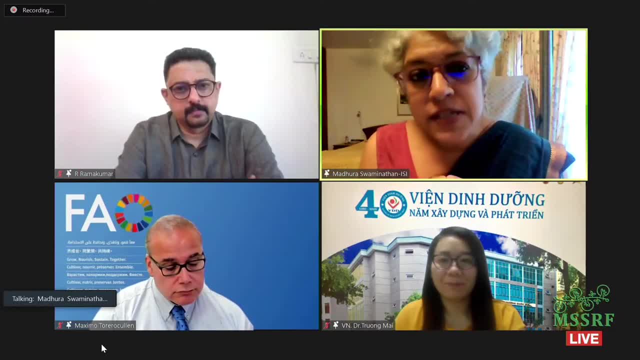 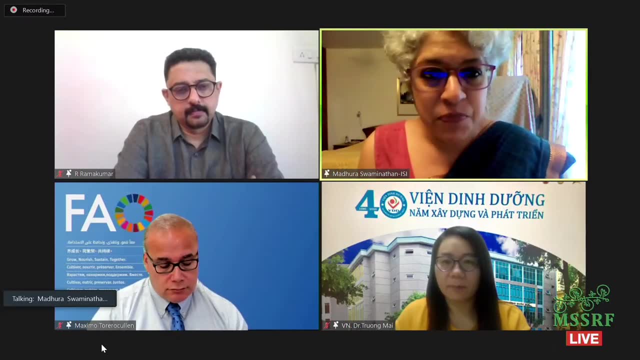 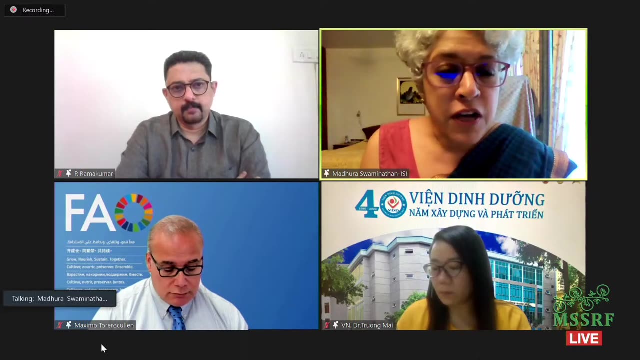 So this really, I think, brings out how very important it is not to focus only on production but on income. So, whether it is because of the, you know, export barriers, whether it's because of road transport problems or crashing prices, 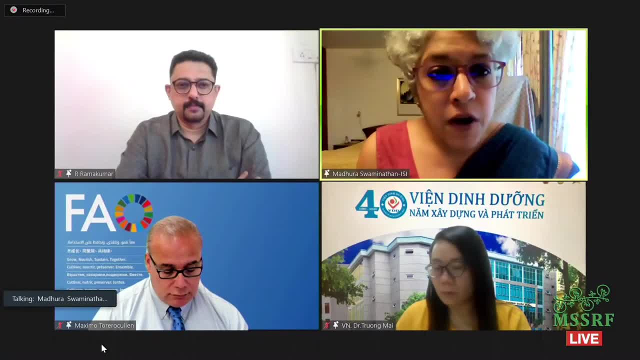 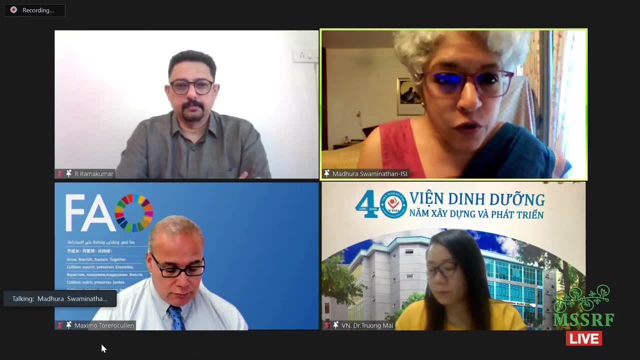 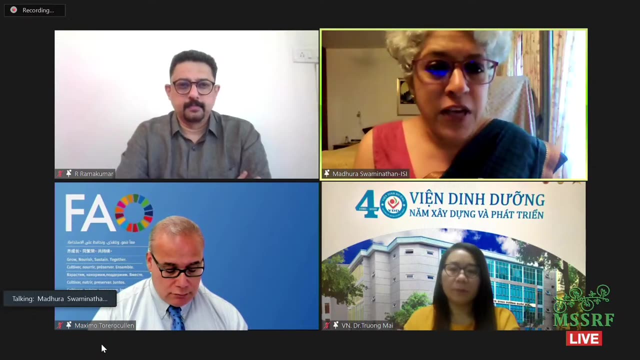 what is the income of those who are farmers? I think that I mean it is, while we do not lose our focus on production. I think this: how, even with good production- we had, for example, last year in India- 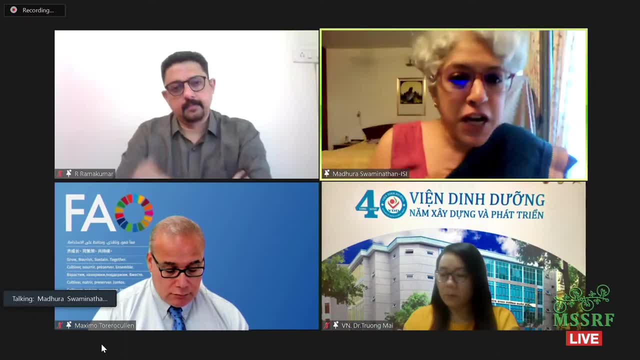 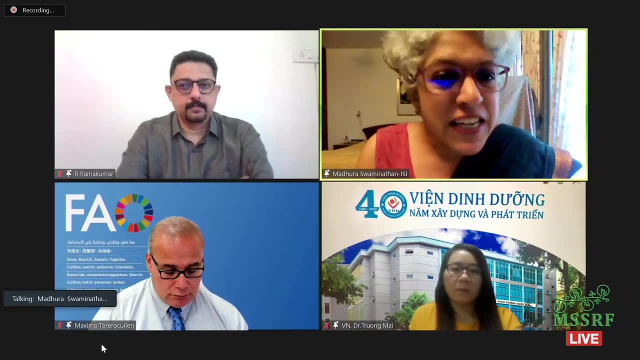 record area cultivation and record production of food grain under Kharif season, our first monsoon crop. But that is not reflected in incomes, particularly of small farmers. And of course, the third link, which has also been made by the speakers: 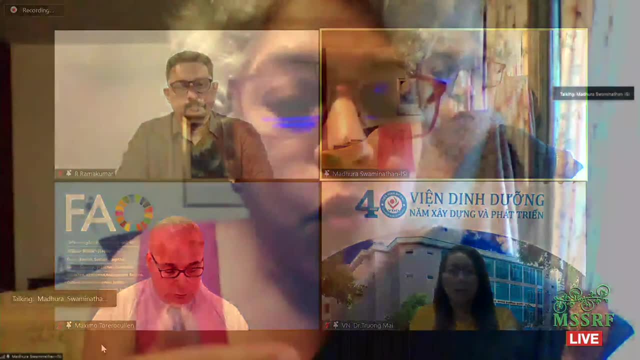 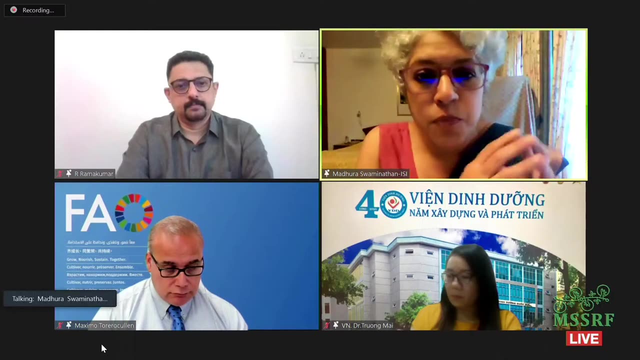 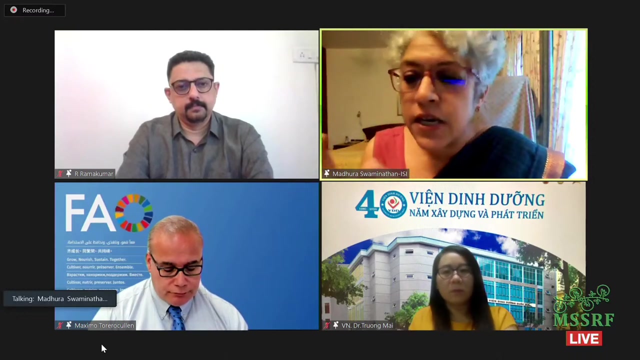 is that you have a collapse of incomes. What is the link with nutrition? And so I think that these three sort of pillars, as it were- production, incomes, and different names were used: capacities, capabilities- people use different terminologies. 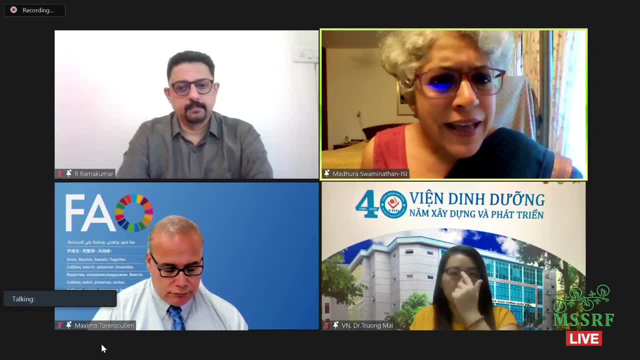 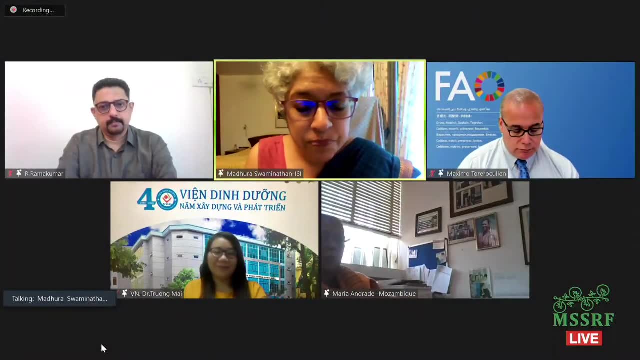 and then final outcomes in terms of health, wellbeing, nutrition. So I think we've had a very diverse set of presentations but actually coming together, And one question that has come from Arun Kumar Joshi and I think is a very relevant 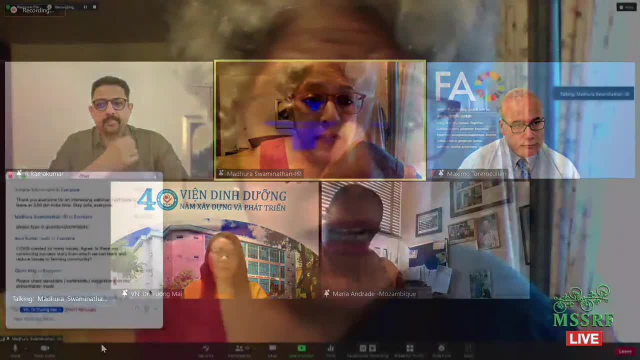 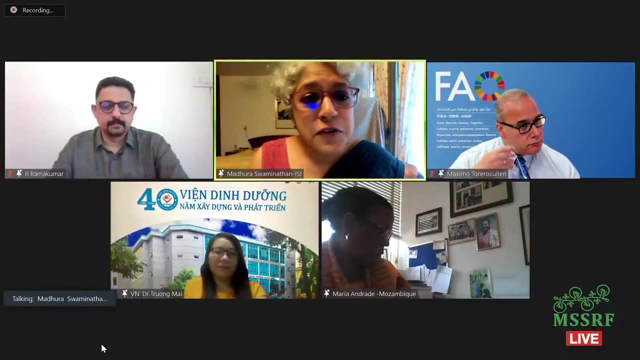 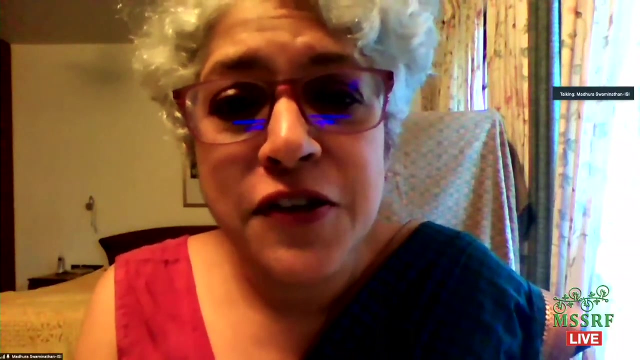 if any of you can, any of the panelists could comment. is there any success story in terms of reducing losses to the farming community? So let me start. Dr Torero, would you like to, from your international experience, any country or any experience? 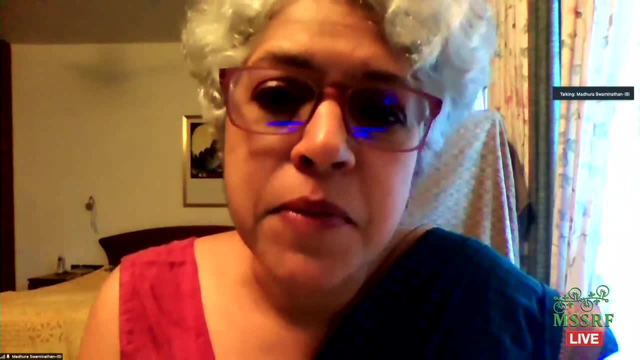 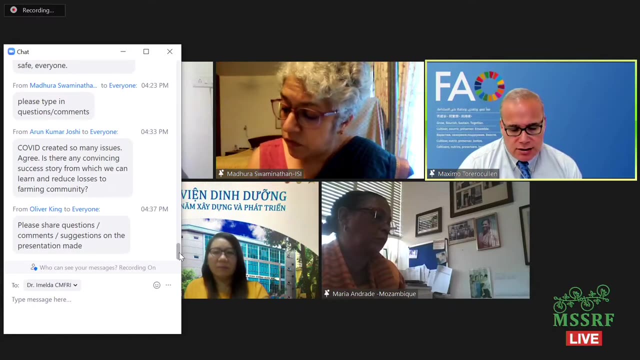 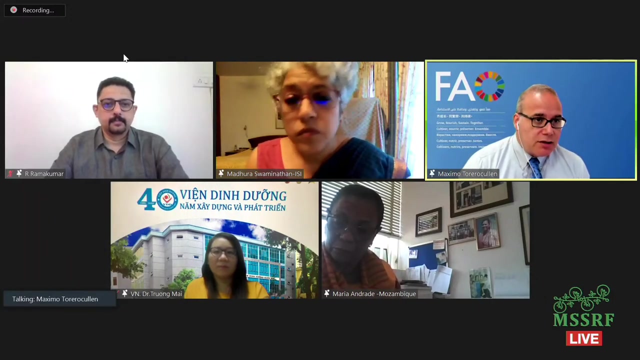 of addressing the problems of farmers in the pandemic. Thank you, Thank you so much. Look, there are several things that show positive results. First, the agricultural sector became more resilient, as Dr Ramakumar has mentioned, If we look at the supplies from India. 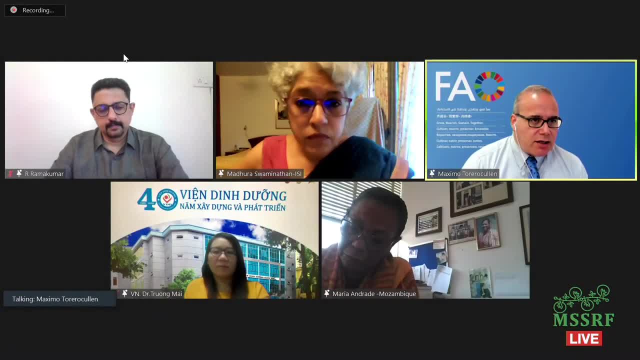 you have a bumper crop right now because of the more labor in harvest and so on and so forward. Of course that doesn't mean there's hardly more access to food, which is a challenge, But the second element that has shown to be pretty important. 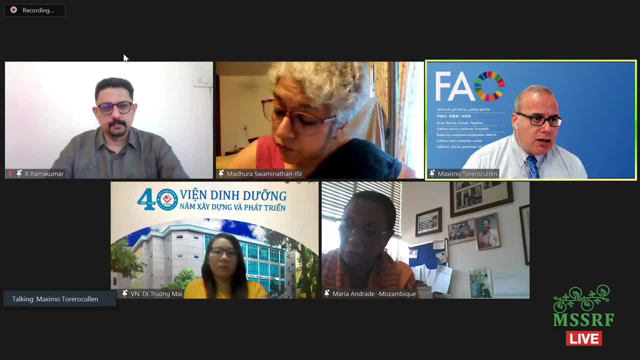 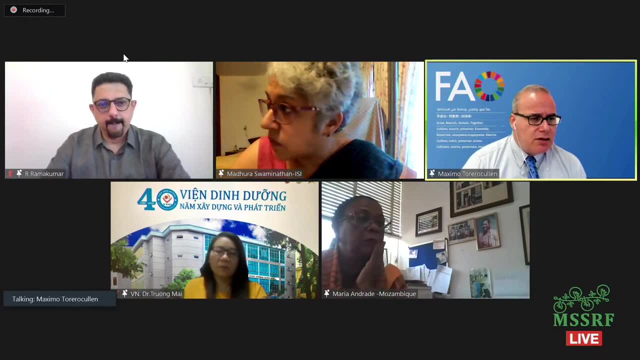 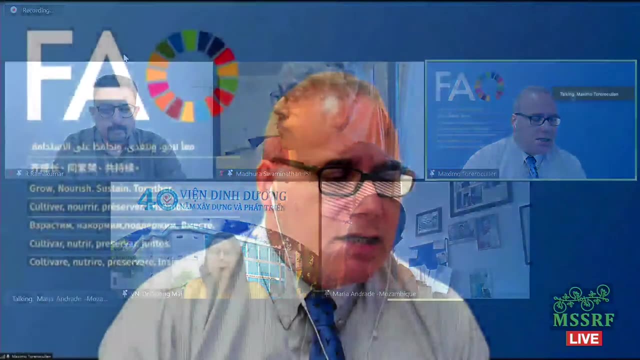 is digitalization and e-commerce, Although that has worked only in countries that comply with certain conditions. So it's not just the digital platform, It's not just the mobile money, It's also having the supplies to do the e-commerce, but especially having the capacity. 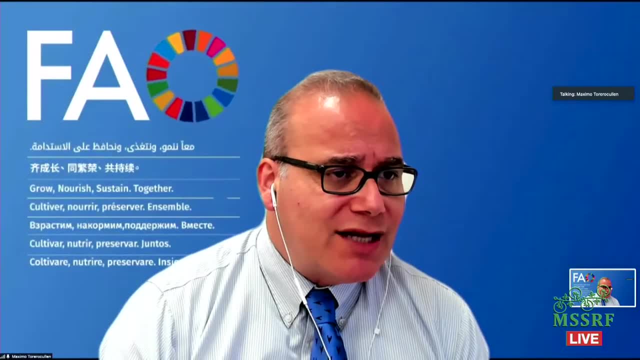 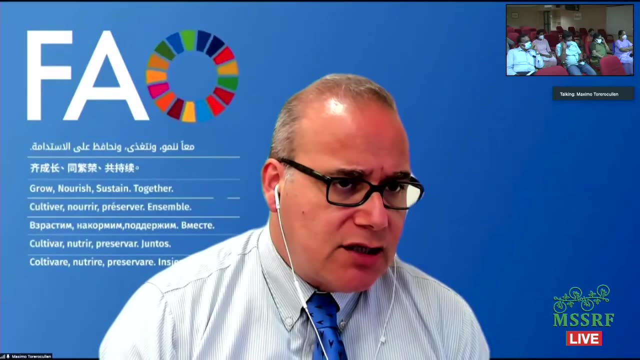 to move commodities, And that's where infrastructure matters a lot. So people talk about e-commerce, but e-commerce requires those four conditions. China had that advantage and they were able to profit from that substantially. And other countries have shown that, But I think in India. 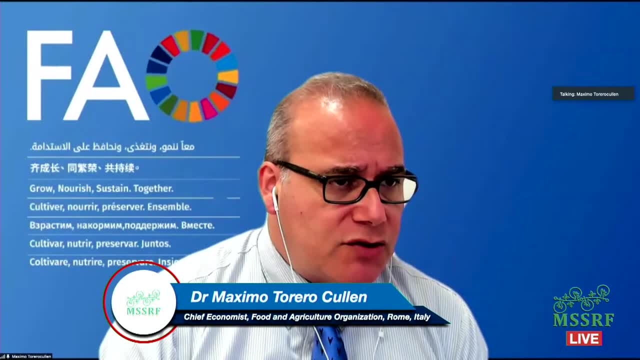 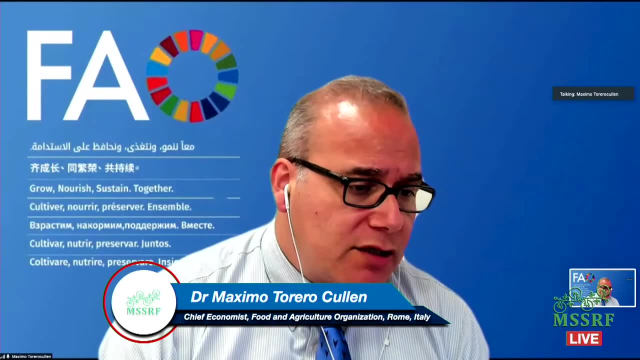 there is a lot of opportunity to do that, But again, the value chain infrastructure will be central and the communication infrastructure to be able to make that a significant reality and to profit from that. Why so important? Because it closes the relationship between markets and farmers. 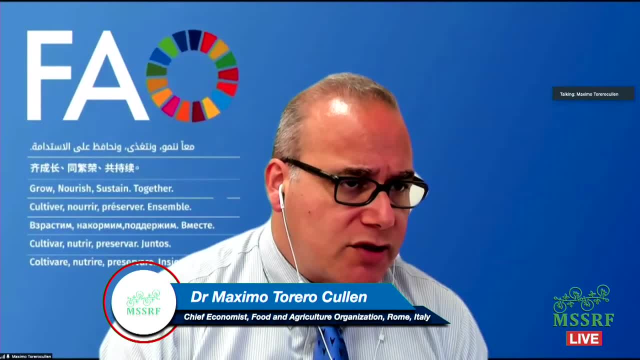 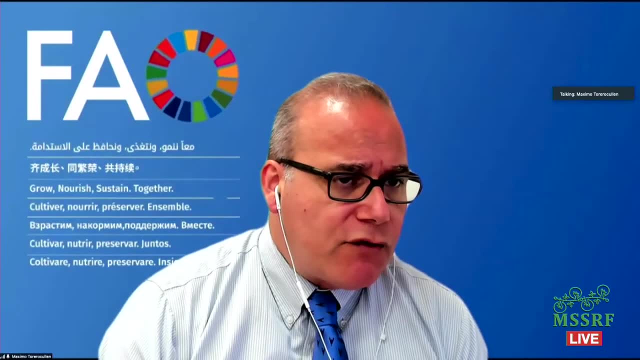 So it brings farmers closer to markets, with lower transaction costs, meaning that you reduce the amount, the level of intermediation that you need to be able to sell your commodity. So that, for me, has been something important over which we can gain and do a lot more. 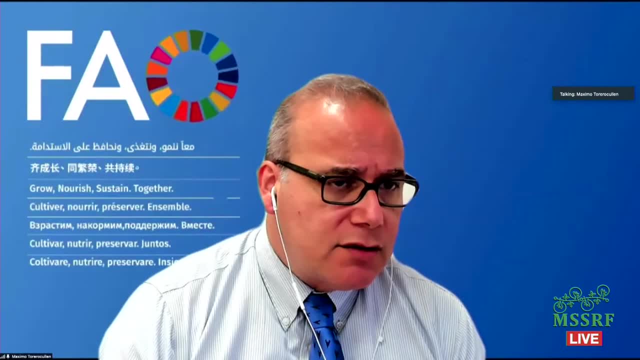 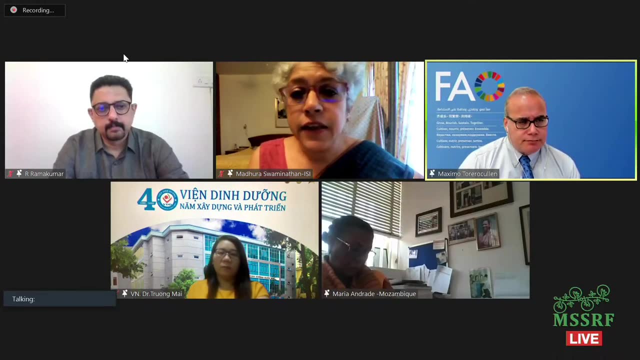 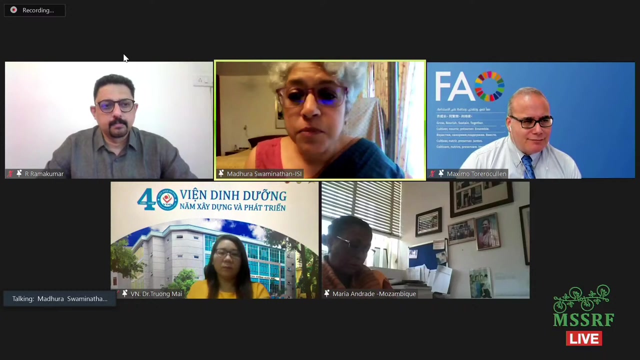 and open the window for important role of governments to increase access to broadband and then, of course, operate with private sector operators. Thank you, You're muted. Can I ask? Dr Maria Andrade? you know your experiences in Africa, particularly Southern Africa. 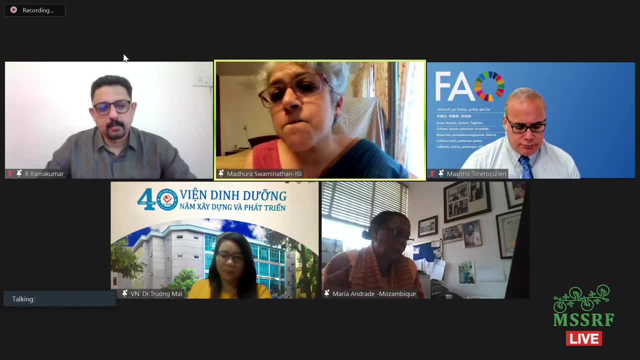 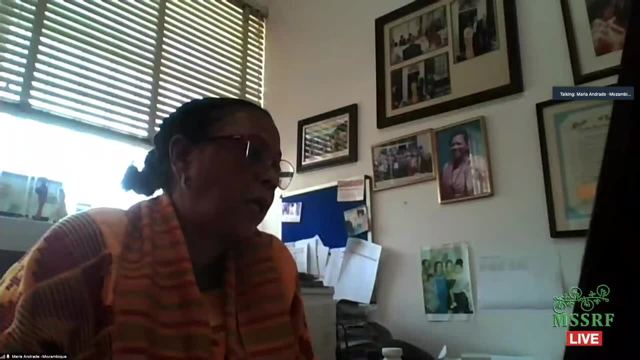 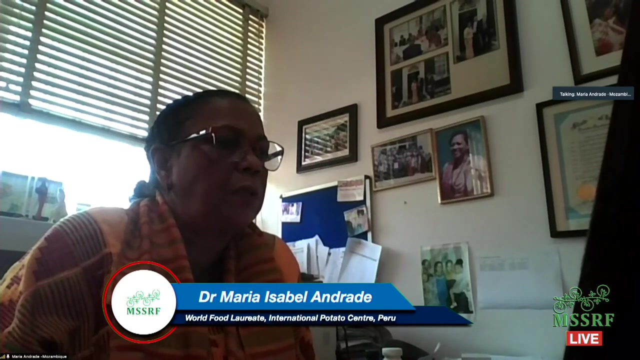 any success stories in the pandemic? Yes, Thank you very much for the question. In Africa, like Hama Kumar mentioned, we could see also that there were increase in production, but that has something to do with a lot of people lost their former job. 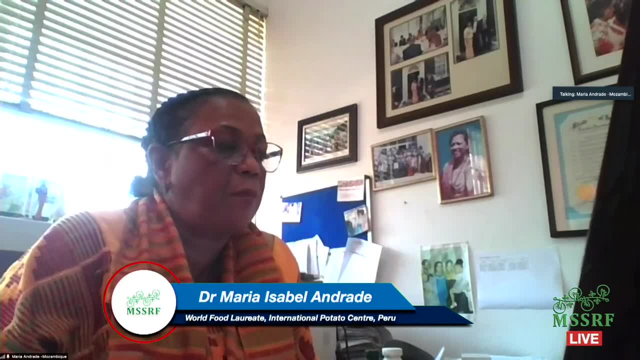 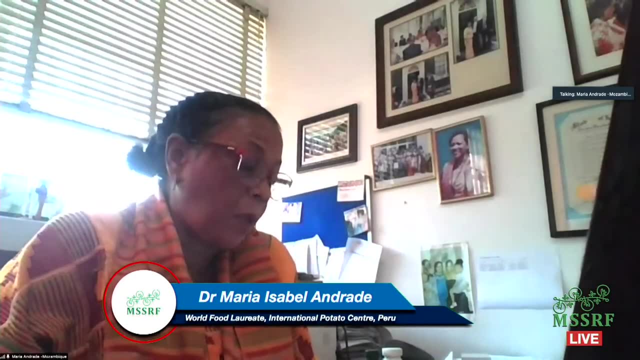 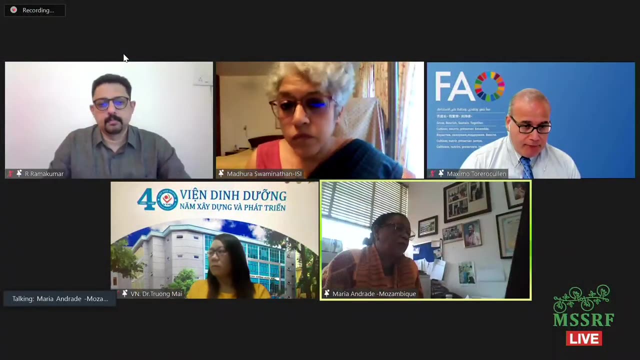 and every people, some of them even with very little knowledge in agriculture, invest in producing food. However, the food, there was some limitation because the roads are very difficult, The law and regulation with the government on the local transport which they have to keep this physical distance. 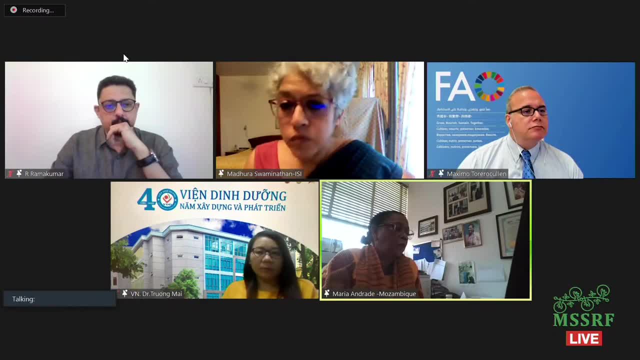 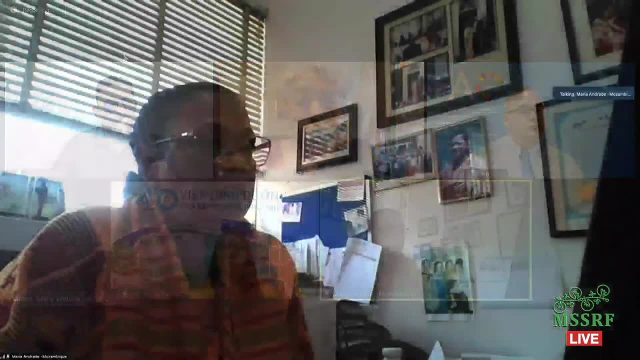 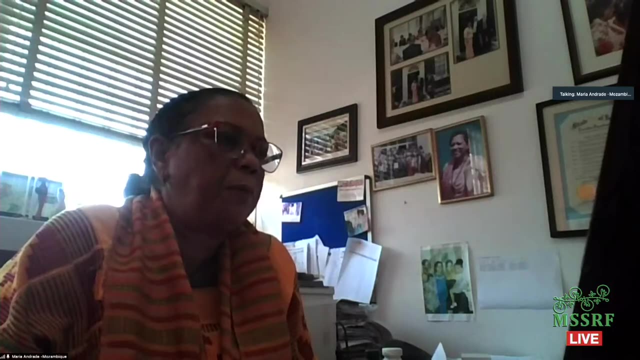 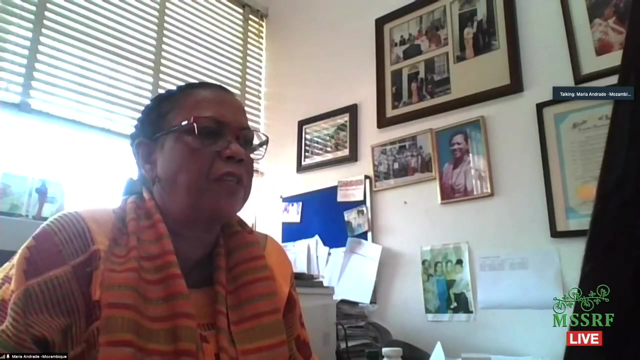 very few people could get into the public transport and few agriculture products could be transported. And even in the local market, where you see so many people selling their agriculture product, there was huge regulation. every day You see battles with the municipal police and all that. 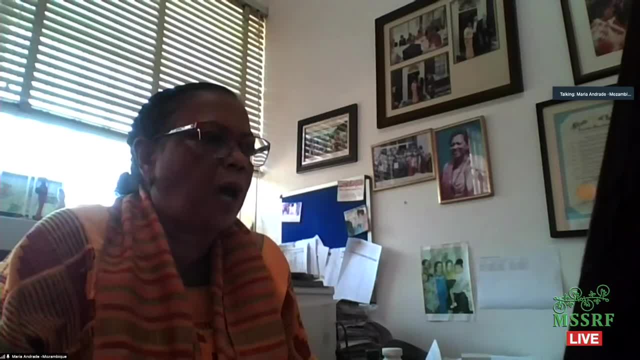 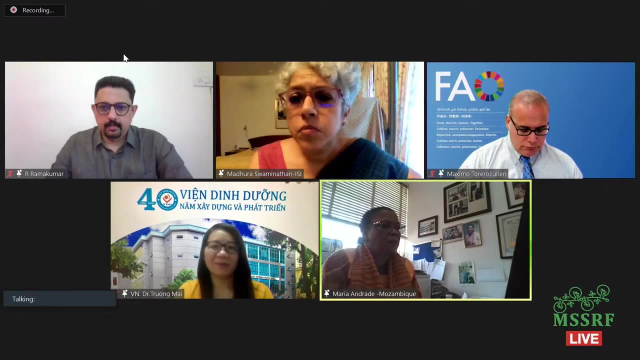 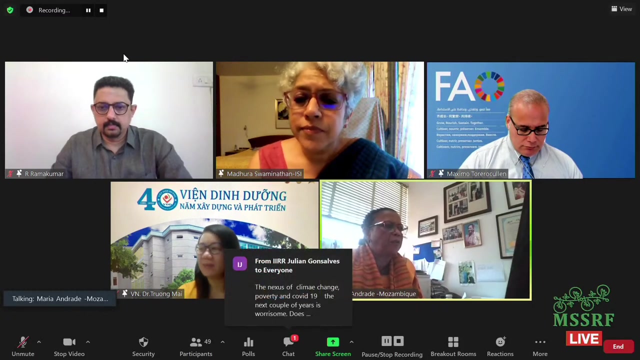 trying to send them off to the house because of the pandemic. So the productivity was very, very high. but also if you reach into the market also the price was very low. If you look at the women that depend on those informal market. 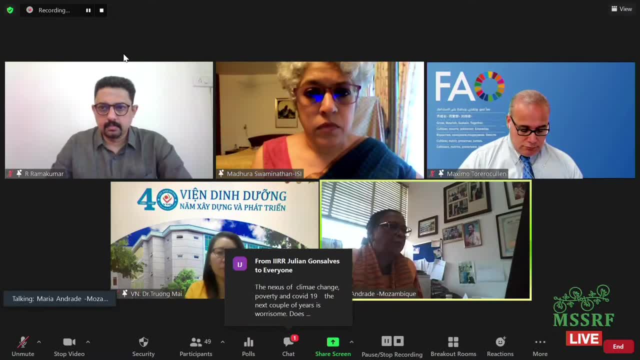 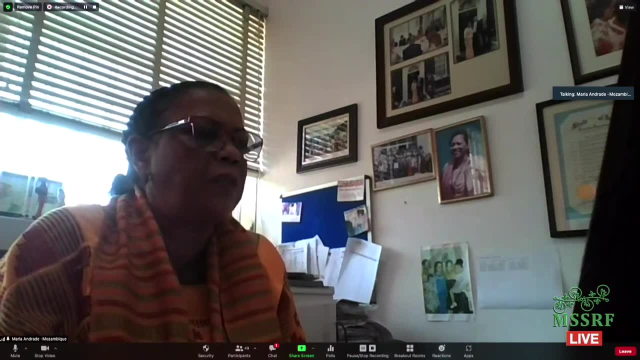 saying it's very hard for them to be get any income, because some of them even depend on the daily income to go and buy, let's say, 100 grams of sugar, and all that to prepare that only meal that they prepare at the end of the day. 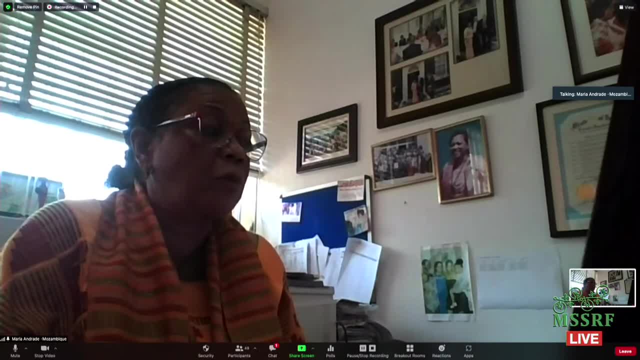 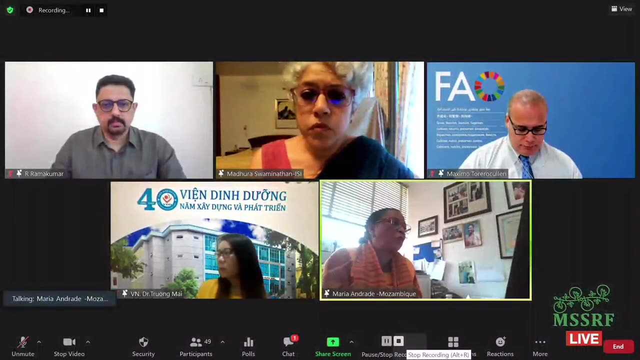 So it was very, very tough And also social program. if I'm thinking in Mozambique, it was very limited because- and people really but the productivity you see in the, but also the knowledge on nutrition, really among female groups, 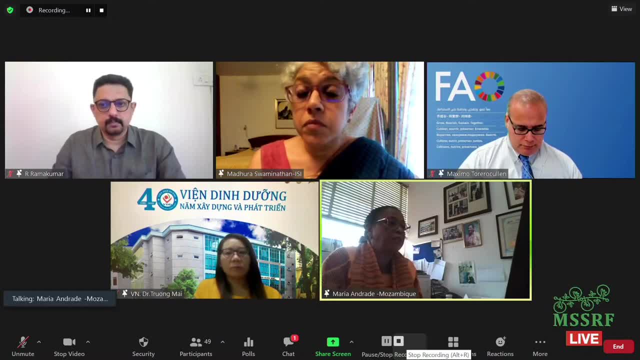 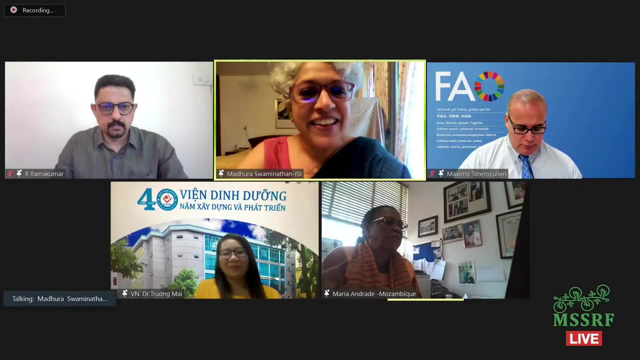 and men increased because everybody is going looking for herbal teas and garlic- I think garlic and other herbs were, and ginger was highly seen in the market at very high price. So there was a lot of knowledge on nutrition of people who never took. 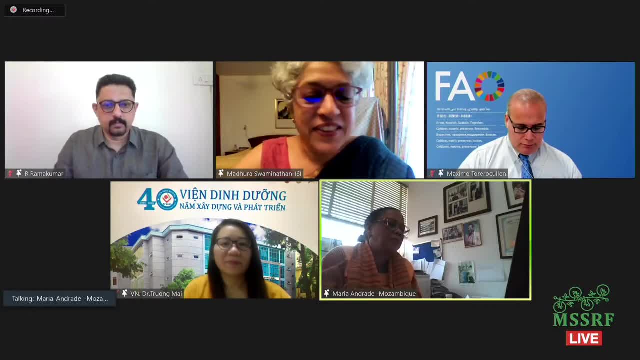 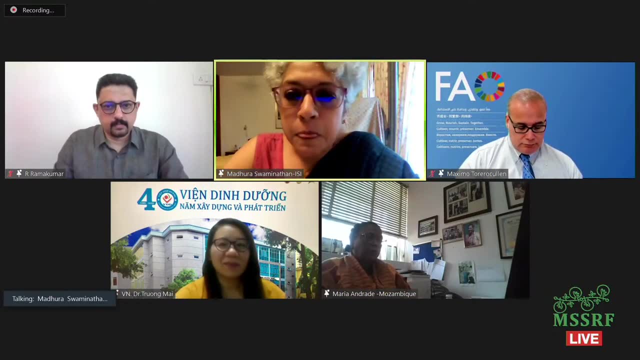 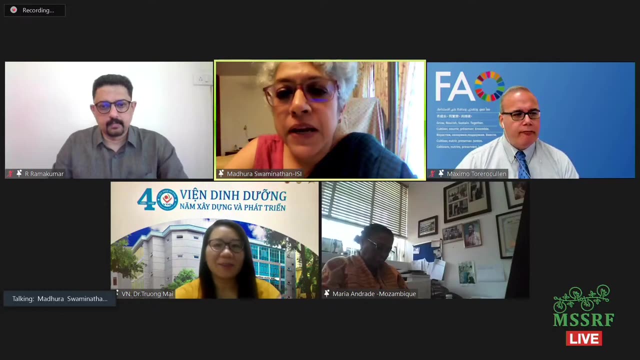 thought it was very important. Thank you. Thank you so much. Can I ask Dr Truong- this is again a question from the floor- that in what way have social protection measures been expanded in Vietnam after the pandemic? What were the main? 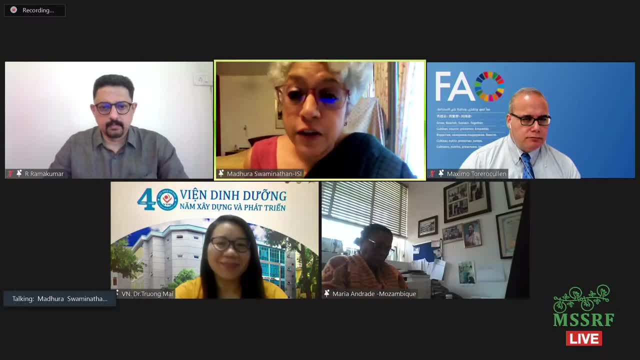 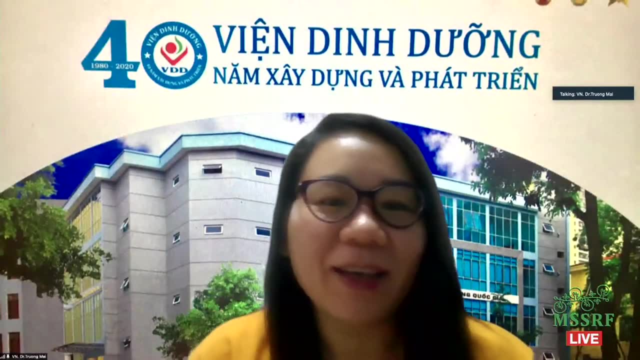 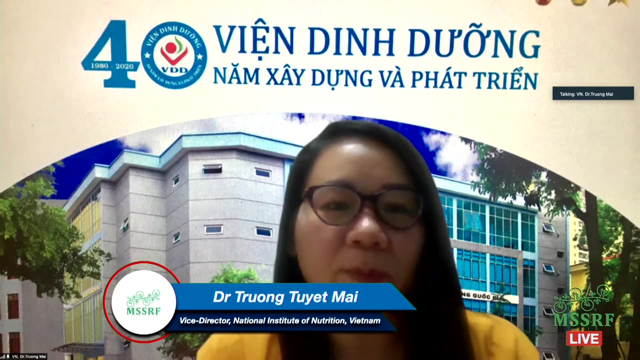 social protection measures, new or strengthened after the pandemic. Okay, Thank you. Thank you. question from Madam Chen. Yeah, So I think it's very important to the first action from the Vietnam government. we have to put the very big package. 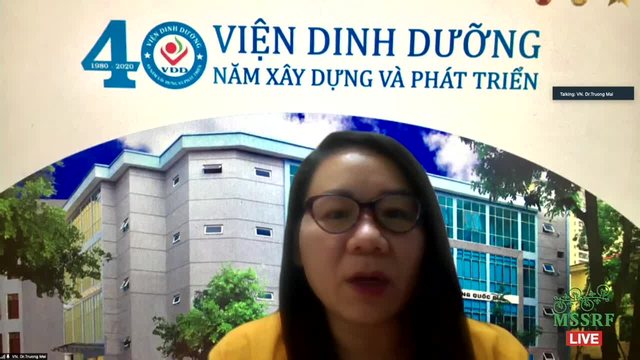 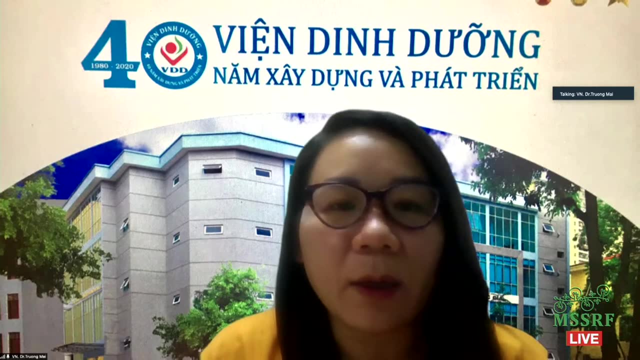 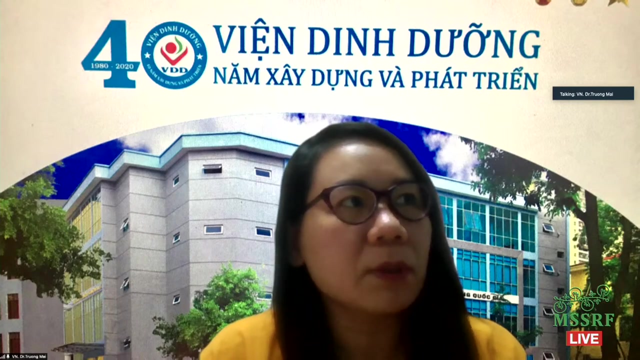 of the money to give the people is a lot drop in the Vietnam during the COVID-19.. So it's a government. I uh how i can live by in the uh 60 into the either uh nearby the 90, uh 90 000 billion vietnam. so 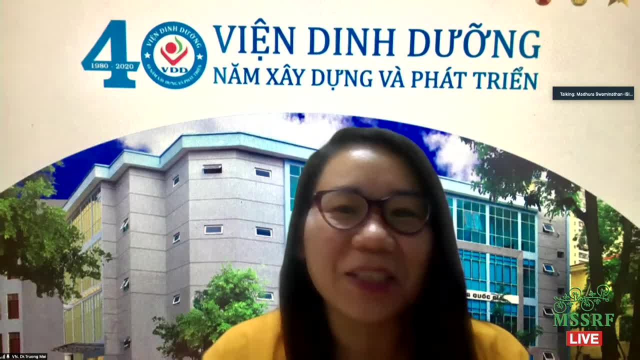 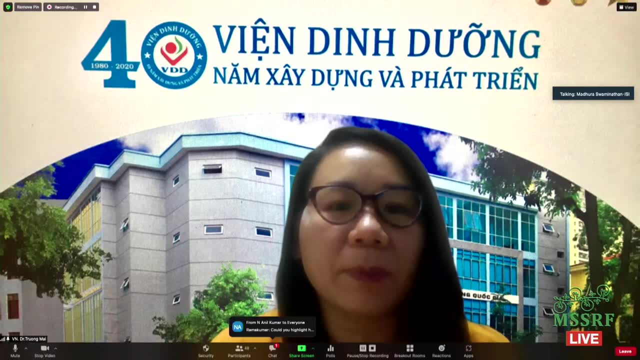 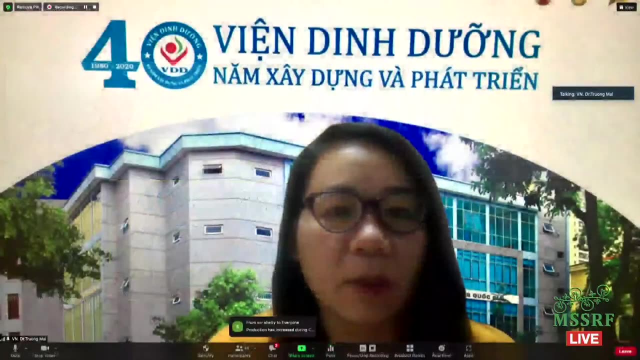 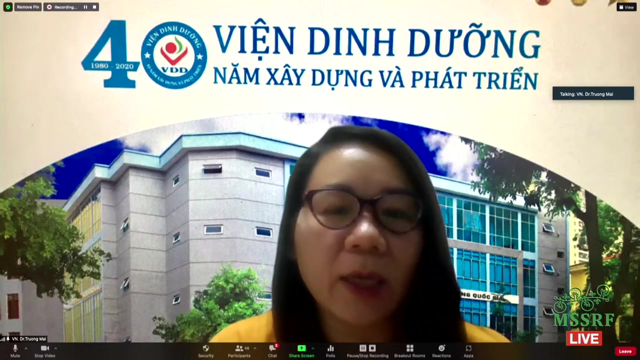 that's mean in the, i, i, i, i, i can't get ready, no, no, i think it's a very big the, the, the amount, so for the people. so do you know, in the the social protection is a very important for for the poor people and to not drop the people in the vietnam. so the government action very quickly. so in the 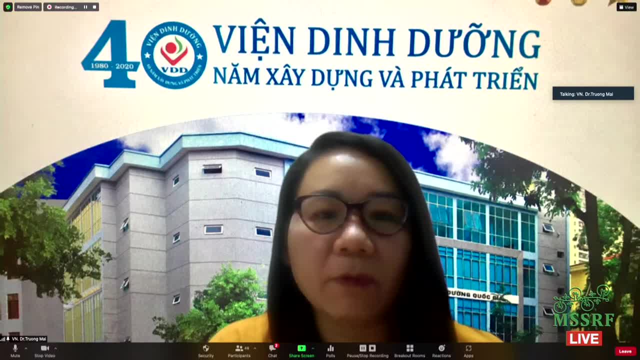 last year in the. this year we have a two time for the government to support. so another support we know in the vietnam, in the, directly to the give the money in the another social protection we call the volunteer uh, the social uh organization to can support the money uh to uh to to get the. 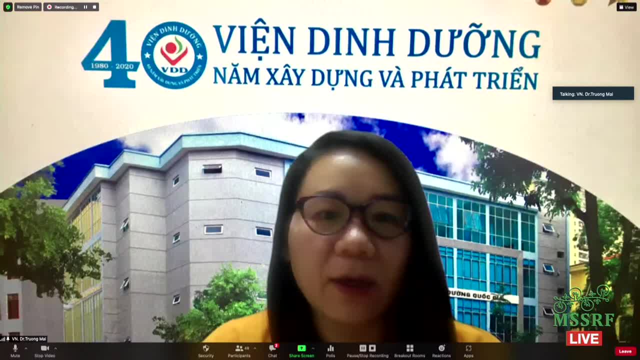 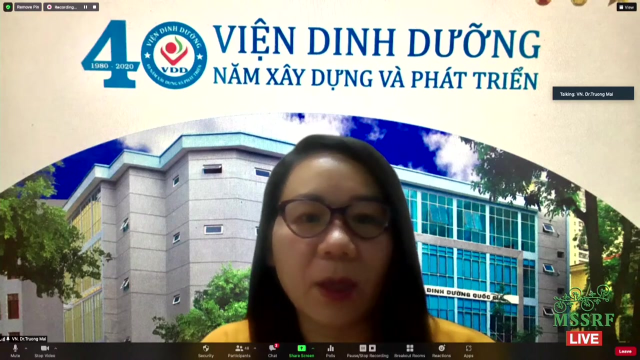 fund uh for the fund kovic lighting fund uh. you call the government to support to get vaccination. so, and then to uh to keep the, the, the food and the money to the the lockdown area. people can get the food and can get the, the, the something uh, the some uh, something to serve. 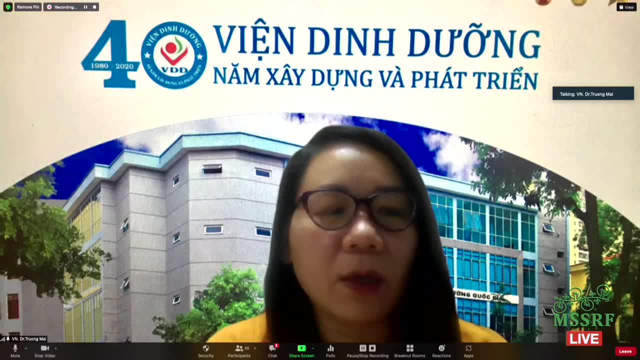 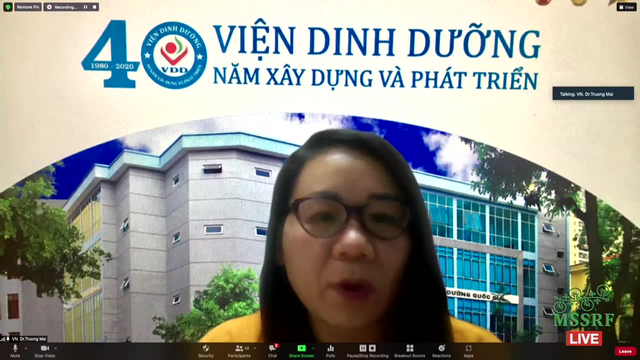 the living. so i think in the very good uh situation now in uh the the social protection uh action in the vietnam, i think is a very uh good action. so but if is a continue, the kovit 19 of course i think is a government uh budget in the low degree. 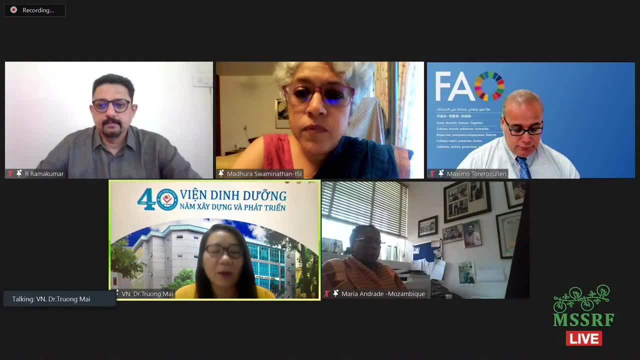 cause the people cannot get the money can can get the income so but i think is maybe in the vietnam now we have to get the two targets already in the reducing the kovit 19k and the increasing the action for the working. we know in the working do we can open the some some. 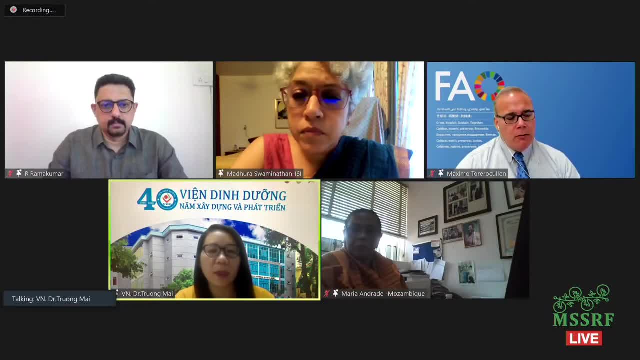 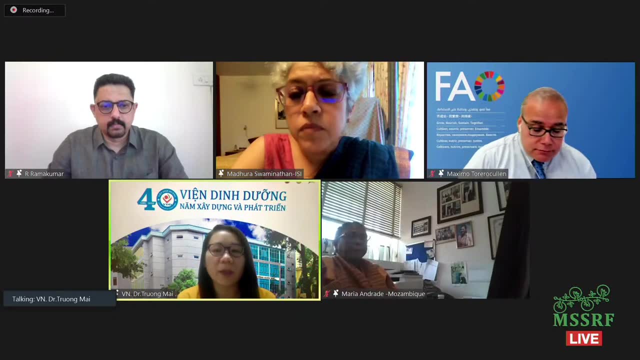 some company uh can do doing send and and can to give the some people can the two opportunity to get the work. so i think in the duty uh in the vietnam government to keep the target of the gdp uh increasing uh in the nearby in the 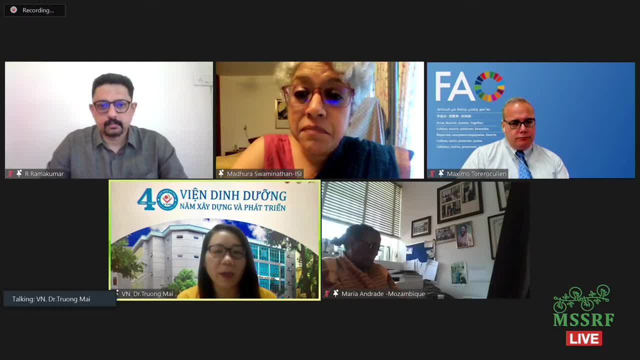 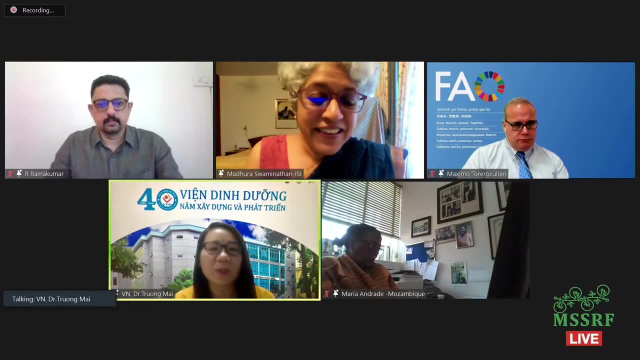 six percent in the this year. so i think that's why now is the government is a very strong action to put the uh, how to get the two target uh already, yeah, so i think it's a very important. yeah, i would you something. yeah, thank you. so question from what i'm saying. no, thank you. we. we learned from. 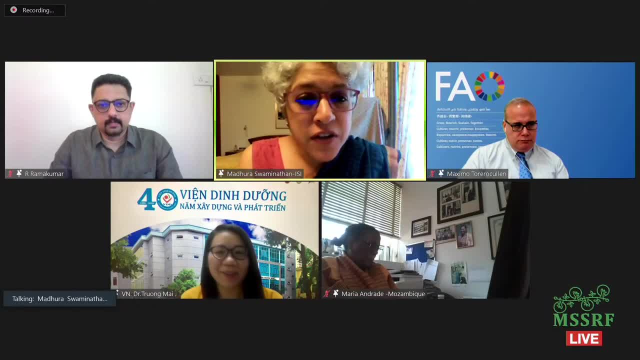 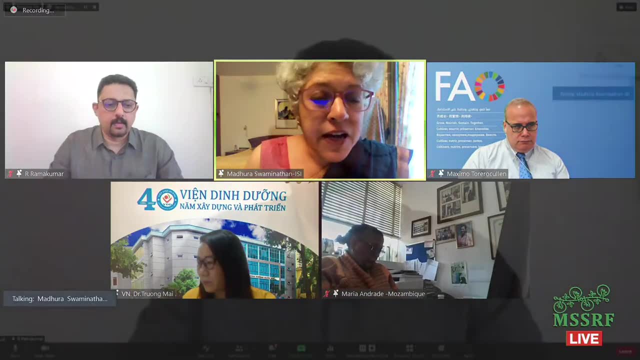 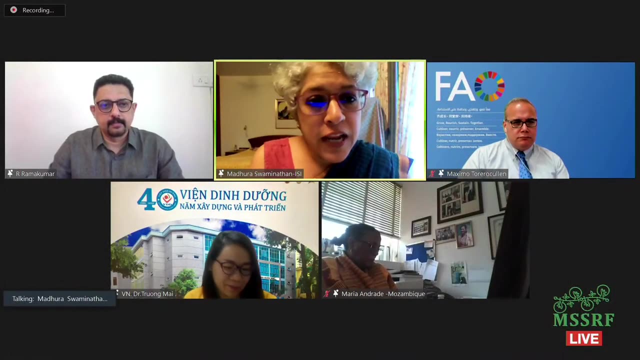 vietnam's experiences, and i do ask dr ram kumar to say a few words about the social protection measures in kerala, as as was being described in vietnam in terms of volunteer force, cash transfers, food transfers and so on. uh, so if you could elaborate on the kerala experience in the 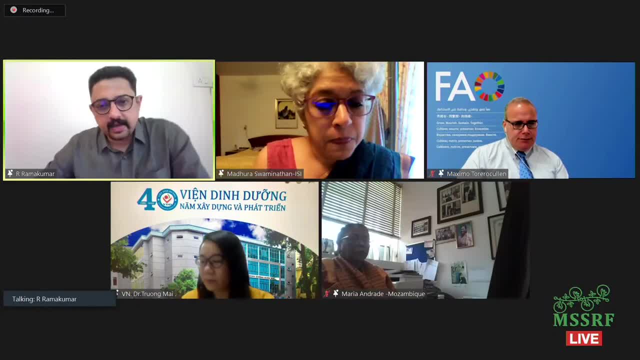 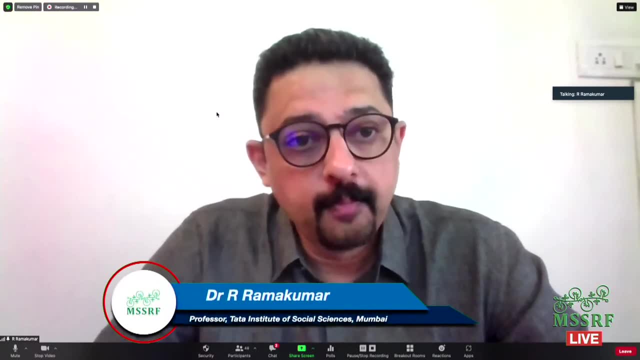 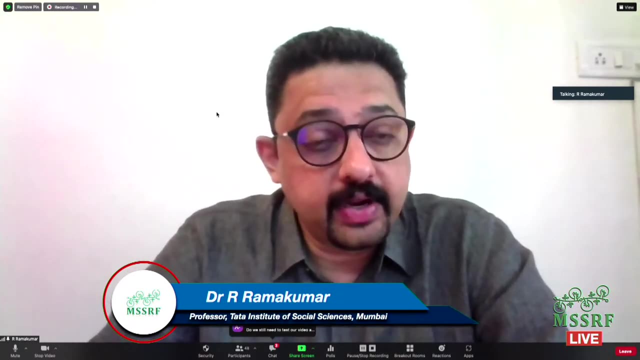 immediate, the short term, the lockdown measures- yes, thank you. um, i think the kerala's experience during the pandemic with respect to ensuring food security or to all, is some kind of a lesson, provides a number of lessons, may say, for other similar countries and regions of the world. one of the major announcements that the 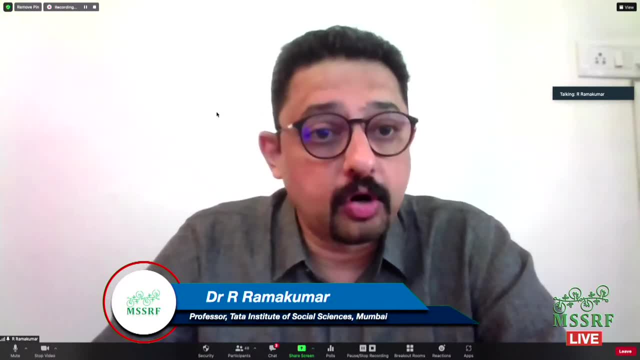 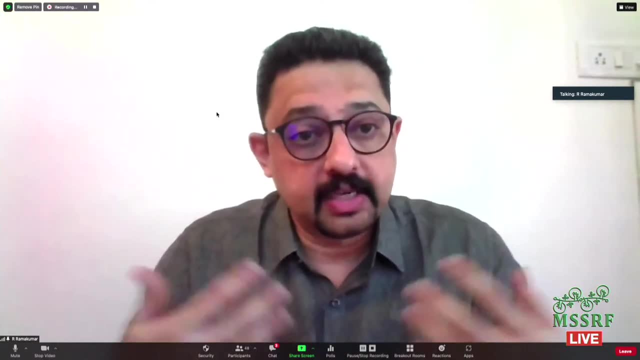 government of kerala made and kept and fulfilled it throughout the pandemic was: no one will go hungry during the pandemic. that was an announcement that they made and multiple steps were taken. the government of kerala had announced that they were going to distribute free food grains to 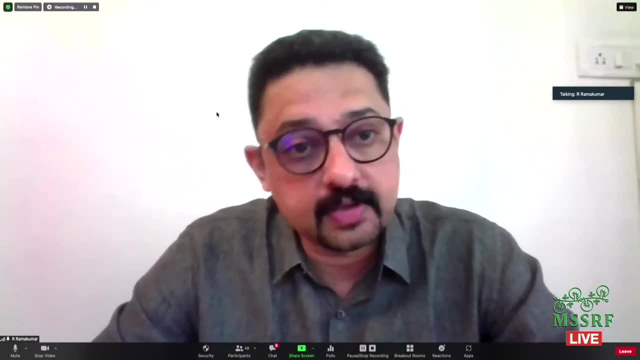 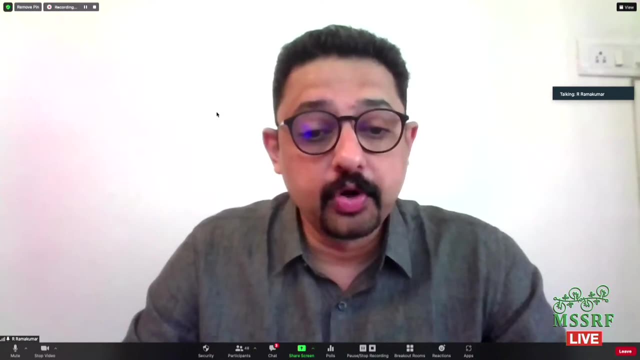 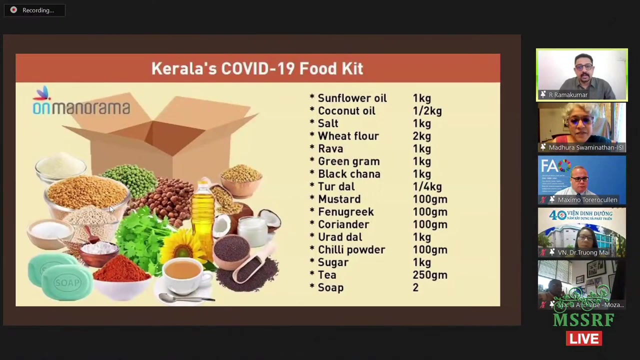 everyone five kg of food grains through their public distribution system. kerala had announced it and had started distributing it alongside what kerala also did. i'm going to share my screen to show you give you a flavor of that uh. one of the most important uh things that kerala did was was: 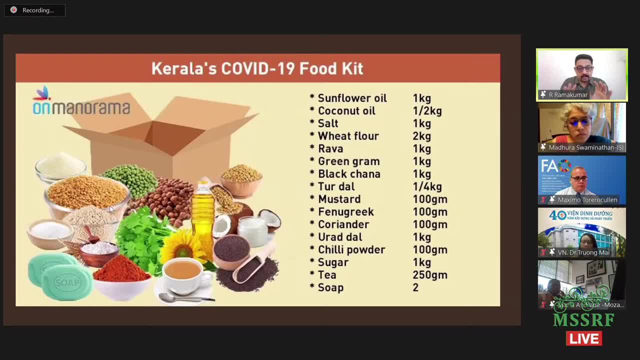 that every household in the state received a food kit and these were the components of that food kit was close to rupees 2000 to 2500 rupees in value. uh and uh, which household could use, as my friends told me, over a period of one month, okay, and every month they got this kit uh fresh. so this was given. 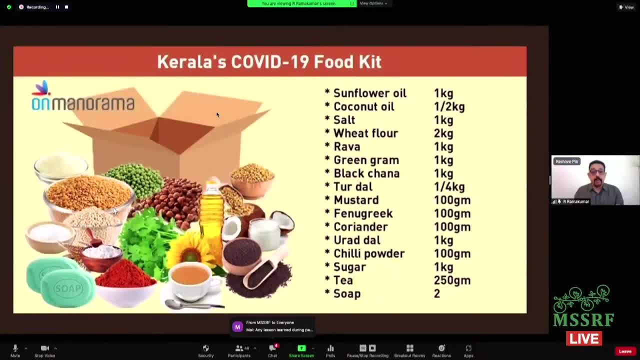 to every household in the state every month and that was a very important relief measure in kerala. the second was across the state in every panchayat, which is somewhere close to a village, but slightly closer to a village in india. every panchayat opened community kitchens so people who did not have 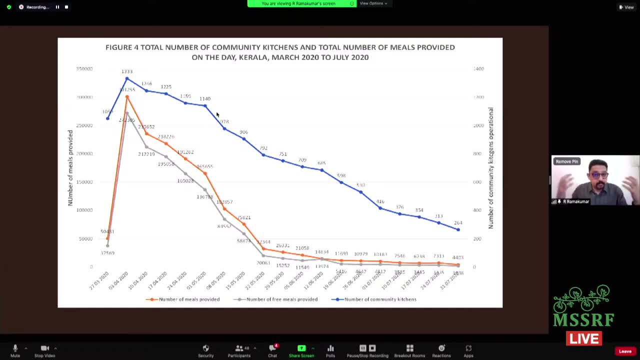 facilities to uh, to sort of uh uh to cook or access food and so on. they could simply walk into that community kitchen and have food for free. uh, you could make a donation if you want, but you can also have it free. so you can see here, uh, more than at the height of the pandemic. 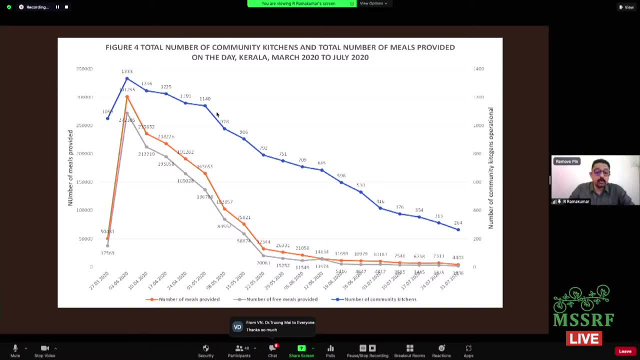 uh people access these community kitchens uh. uh during the april- may months of 2020, which, of course, has uh decreased over a period of time, uh, as the, the pandemic and the lockdown was eased. but the the core help you provided during the height of the lockdown was very useful for for. 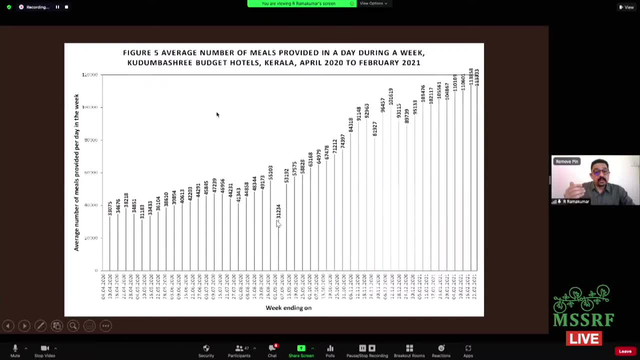 people uh. number three is that the state institutionalized what is called as budget hotels, uh, where you could simply walk in and have a food packet for just 20 rupees uh per packet, and you can see. these are the number of food packets that are distributed uh such in the state, uh at the end of every week, or this is. 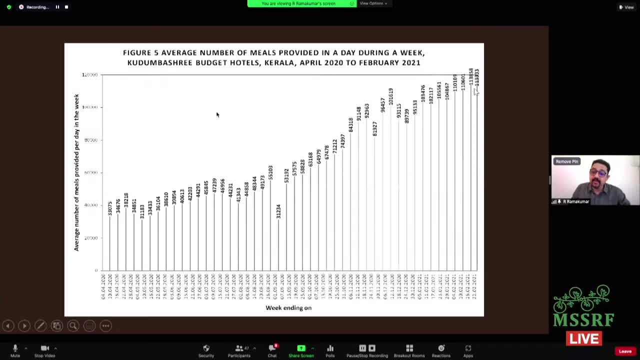 the daily at the end of every week you will see that every on an average by early this year, uh more than 100- 100 000 uh food packets were being sold through for budget hotels uh in the state per day. all this was partly using uh the government's funding, partly mobilizing money from civil society locally. uh better off. 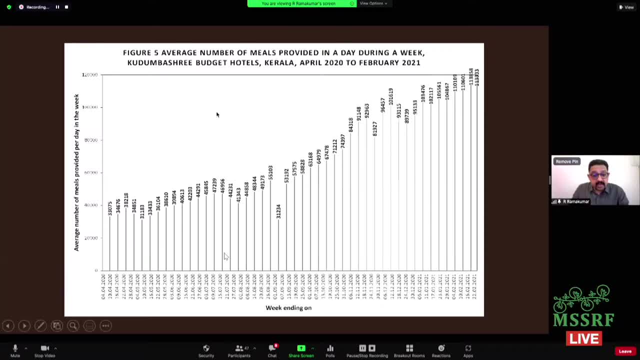 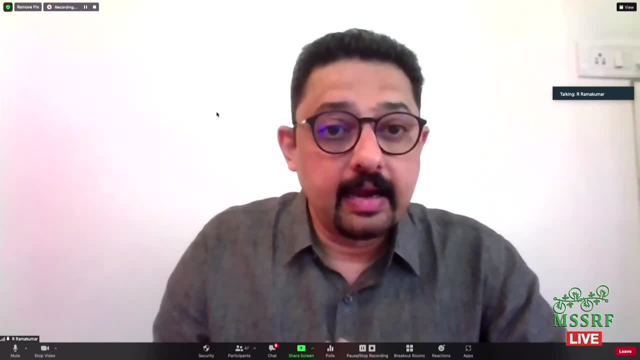 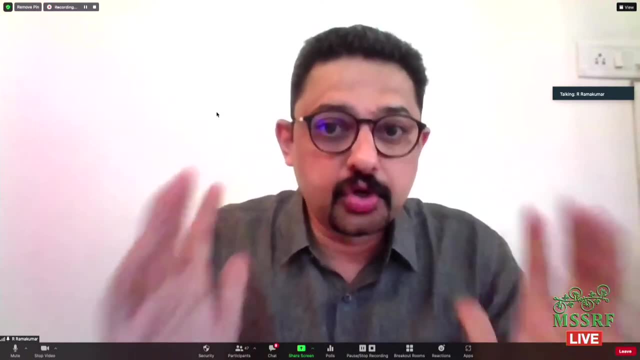 people and so on. uh. so kerala has uh some very interesting lessons on how uh it has addressed the question of hunger during the pandemic and uh and uh most important has been that the state ensured, uh announced, that nobody will go hungry and it actually ensured that actually happens. on. 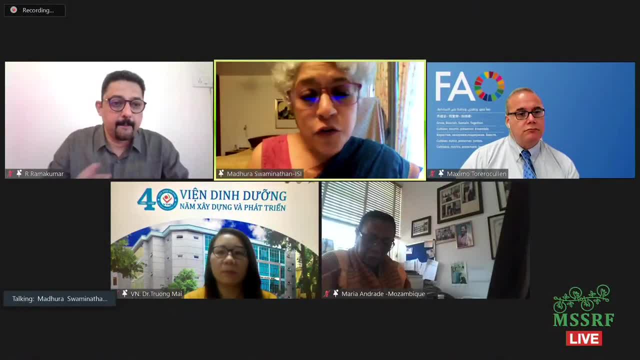 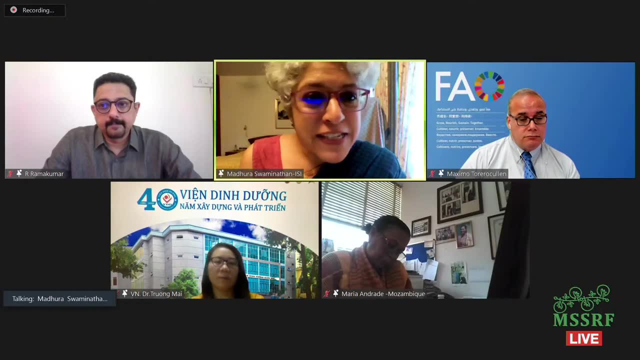 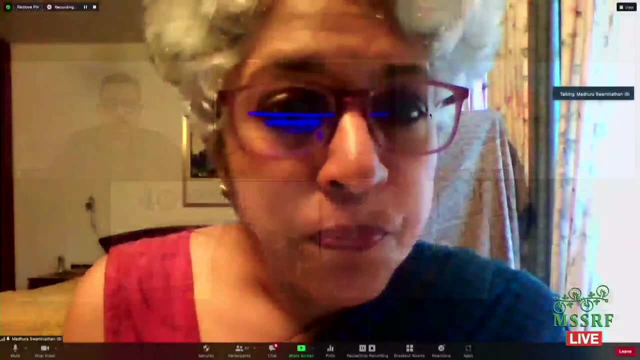 the ground. uh, thank you very much, ram kumar, and i think that brings out, i think, what many of us have been demanding at the level various national and international fora, and that is political commitment. so i think. a person who asked about success stories: uh, things are, although the situation as we heard at the 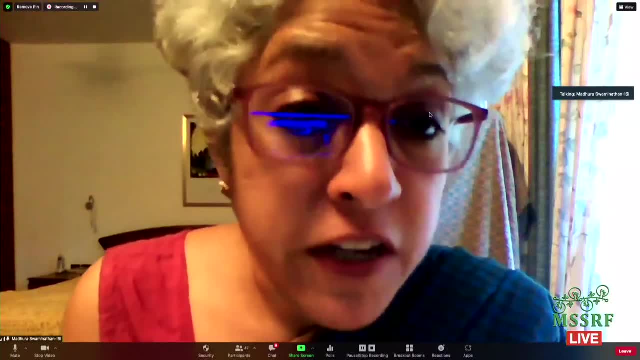 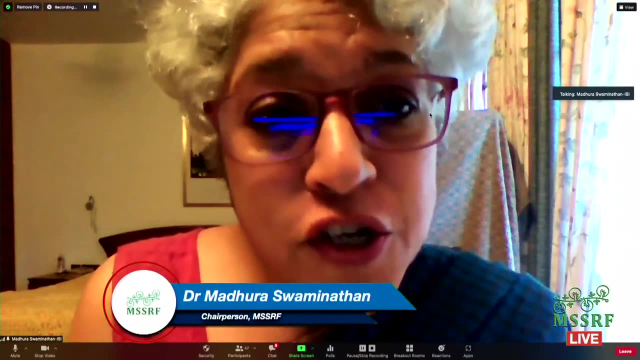 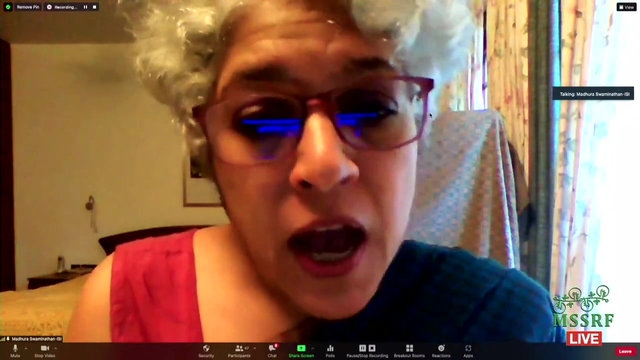 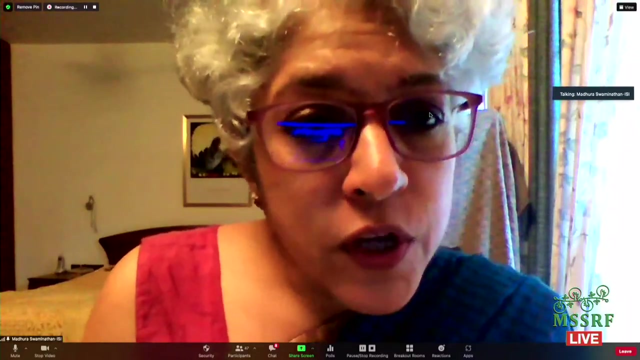 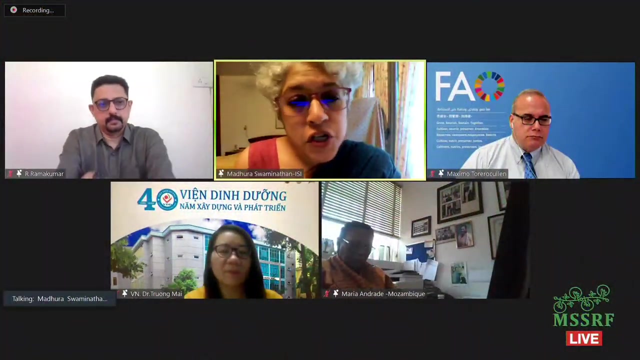 beginning from dr maximo terero, situation looks very grim. whatever indicator you take is political commitment to ensure food and nutrition security. then we can find ways and means to ensure that. i would like to just add here before we close that one of the areas in which mssrf, i think, was a pioneer was in the use of the new forms of information. 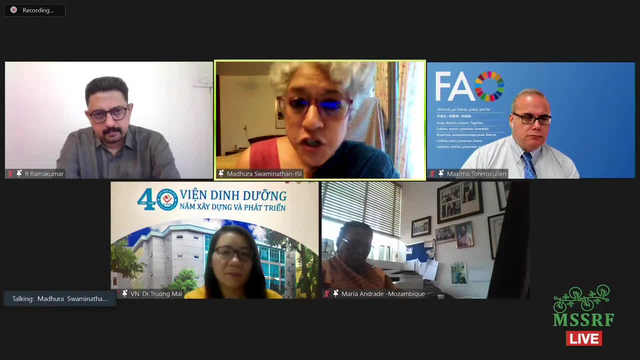 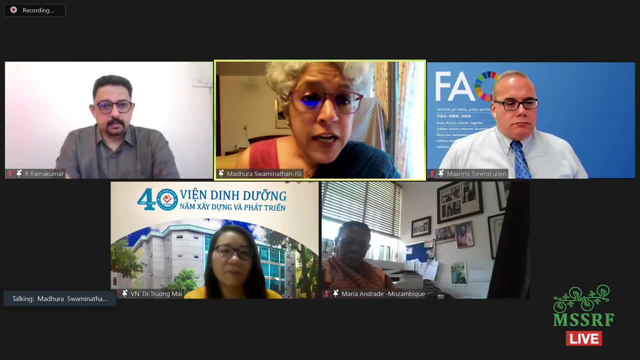 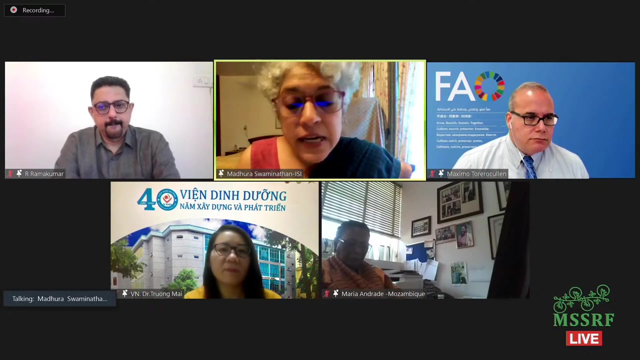 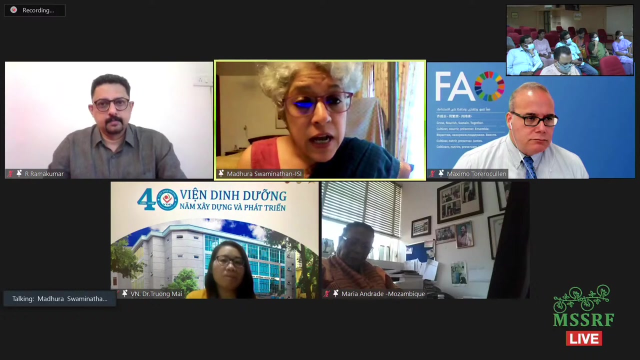 communication technology to reach farmers and fishers, particularly smallholder farmers and women, those in tribal areas and so on. so, starting from uh, using uh, you know, mainframe computers and in small village knowledge centers more than 20 years ago, today, using phone based, sms based, tablet and other app based ways to communicate, has has there are a number of experiments, so i 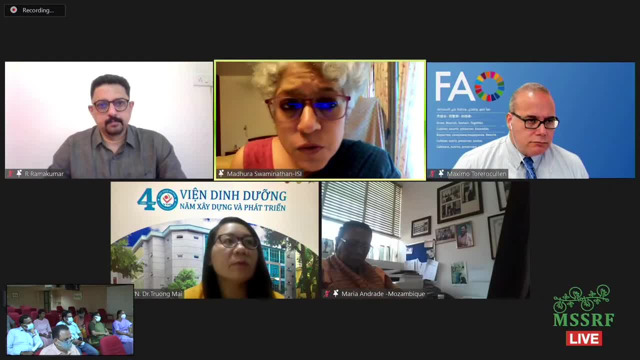 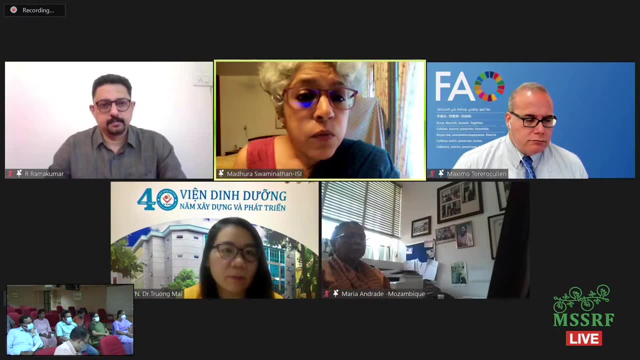 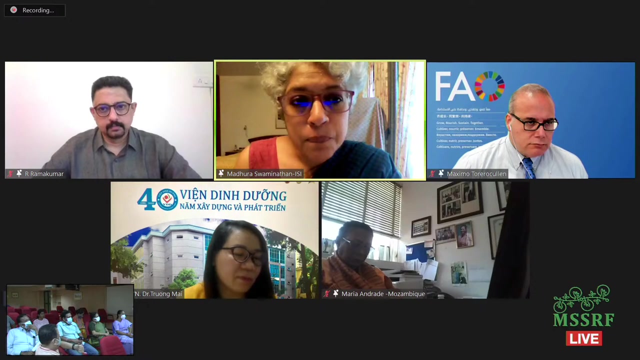 think, uh, going forward, looking at what needs to be done and what can be done, as dr terero also mentioned, you know, about digital transactions, we do have tools and we do have technologies. so if we have the right political commitment and investment to the right kinds of infrastructure and support, i think we can do better for our people. and although 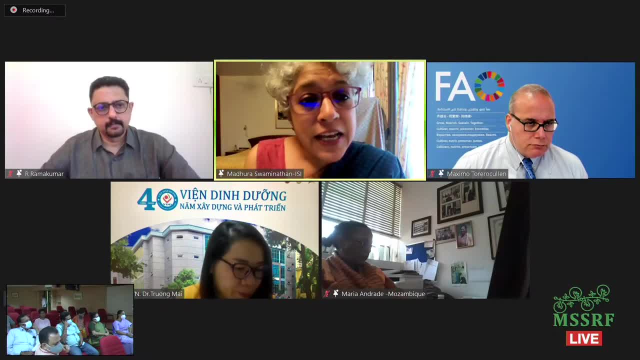 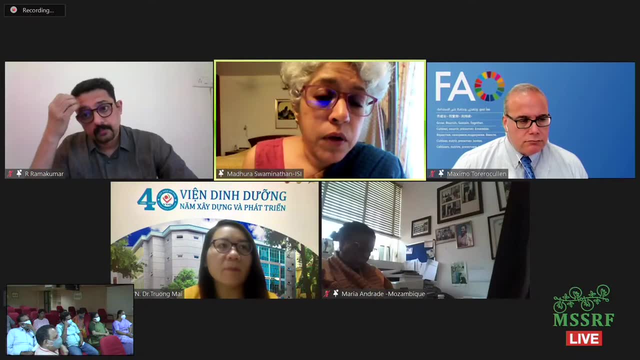 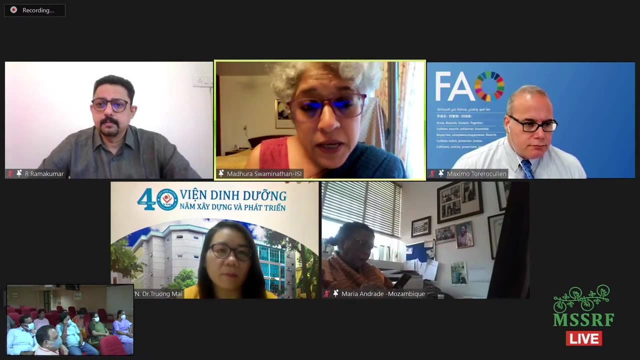 we look like we're falling off all the sdg targets. uh, i think, if we have a renewed commitment from governments across the world- um, as i hope, uh, we will- we can address the issue of the pandemic and actually go beyond it by creating infrastructure that's going to be in place, uh, for a longer term. so, uh, with that, i would like to thank all of you. 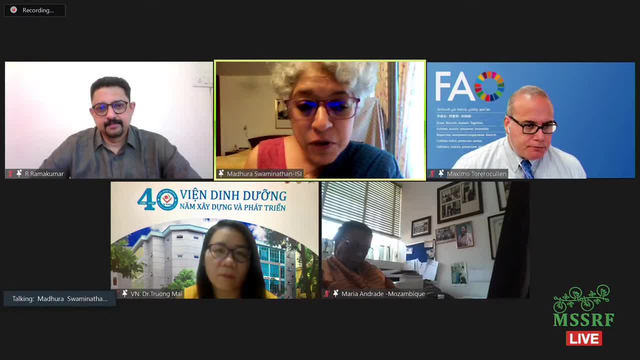 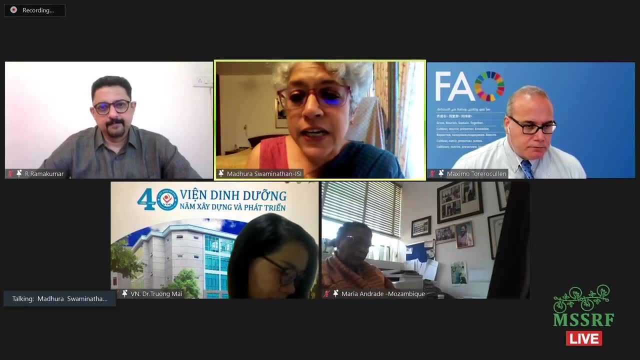 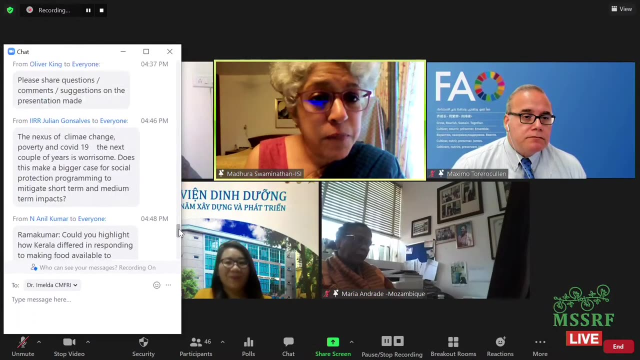 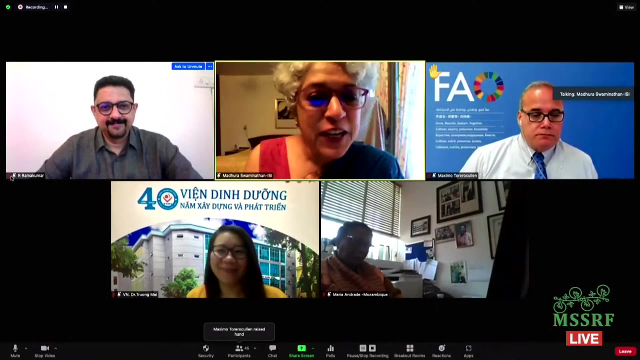 are there any? anybody who's the audience or anybody who wants a very quick question comment? i haven't seen any in the chat box, but the floor is open for a couple of minutes. any of our speakers want to give a minute to wrap up. okay, i think it's been a long day. uh, we've heard. uh, we've been debating these issues. uh, thank you all. 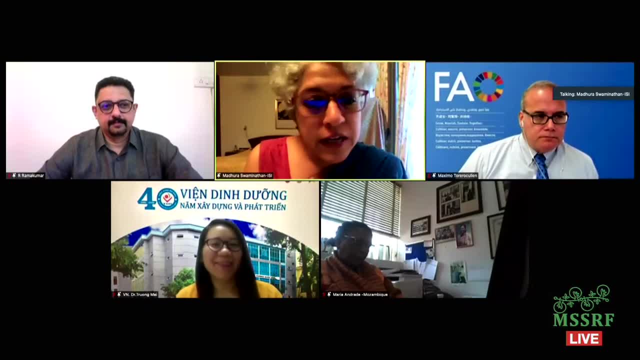 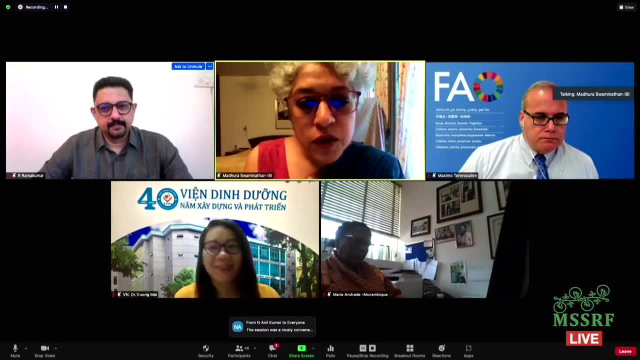 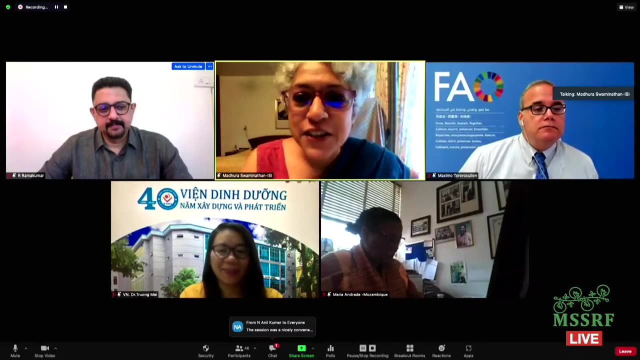 for joining us and we shall be sharing uh the recommendations that come out of uh the deliberations of our conference with all of you and hope to have you see you in person once the pandemic is in control. with that, i would also like to thank uh the session organizers.